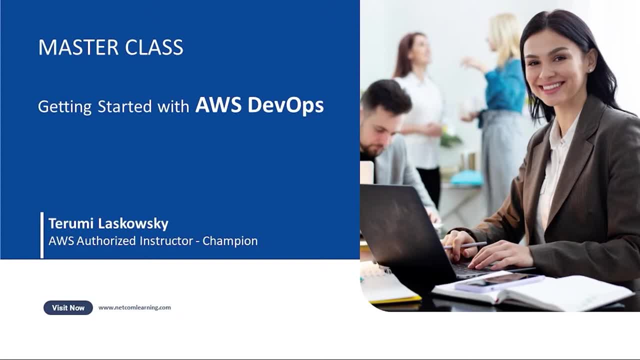 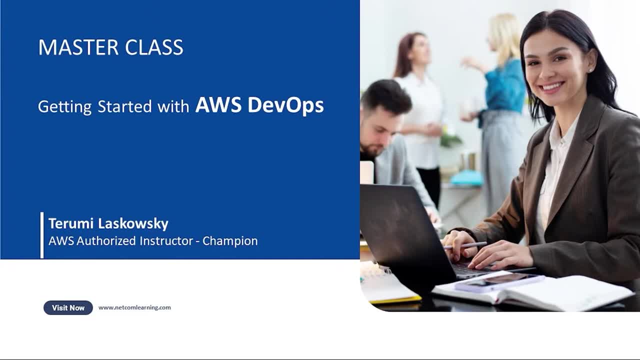 And we're very excited to host today's event Masterclass- Getting Started with AWS DevOps. And presenting today's topic is Tarumi. Tarumi is an Amazon AAI training consultant and author, holding more than 25 years of experience in IT. 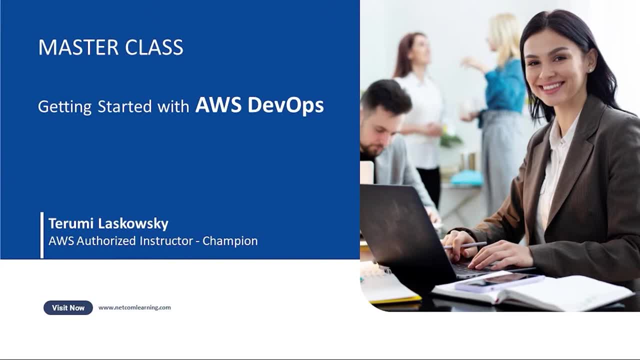 Her passion for cloud computing developed at a very early age. Being a teenager, she always showed her enthusiasm for understanding the technologies that make computers tick. This deep sense of curiosity on technology led her to achieve all the associate professional and specialty certifications and was recognized as an AWS Authorized Instructor Champion. 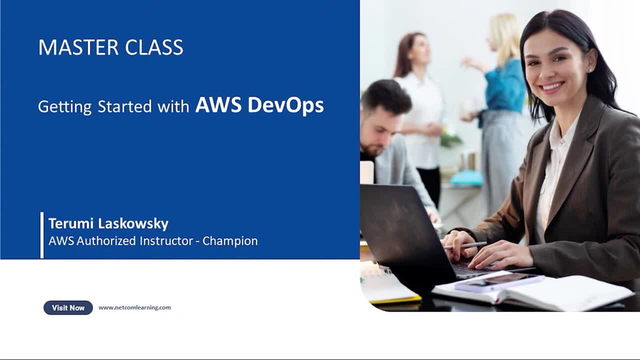 Now, please bear in mind that this is an event that is not a regular event. We offer a collection of technical and business courses that can be tailored to your specific requirements. If you are interested in a further discussion, you can make an appointment with our learning consultants through our website at netcomlearningcom. 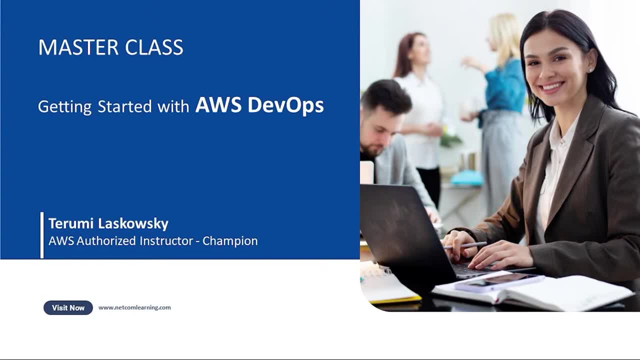 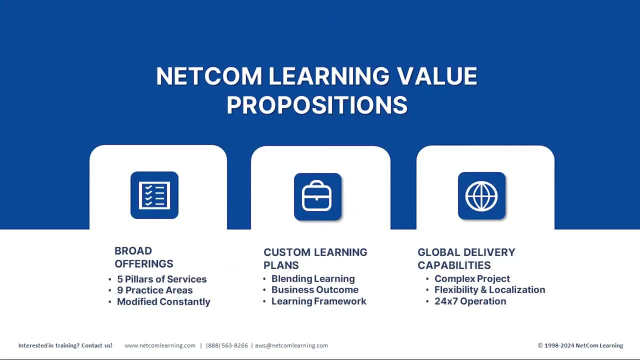 Today's session is also being recorded, so you'll get free access to the recording in the next 24 hours via email. NetCom Learning helps customers build innovative learning skills. We help customers build innovative learning organizations by achieving a smarter workforce, adopting to change and driving growth. 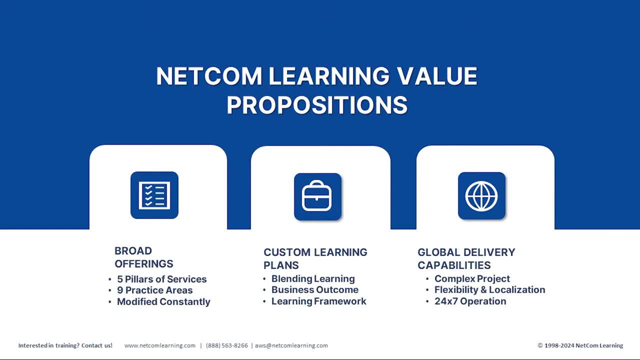 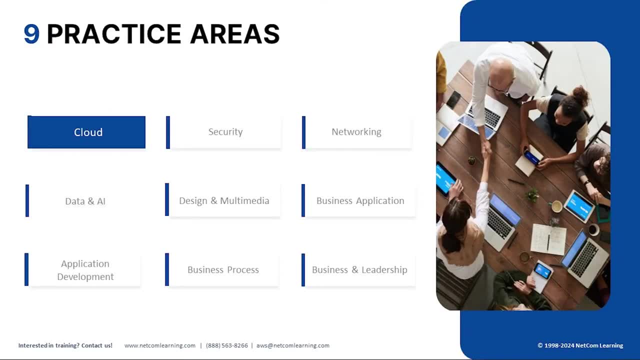 We do this with a broad catalog of offerings, developing customized learning plans and our global delivery capabilities. Since 1998, we have been empowering organizations with our managed learning services to help them reach optimal performance results and address challenges. We do have nine practice areas in which we specialize. 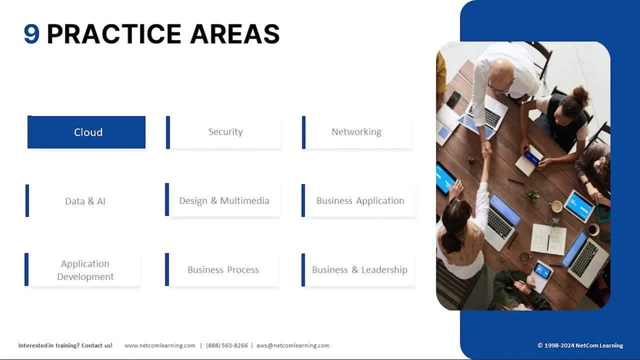 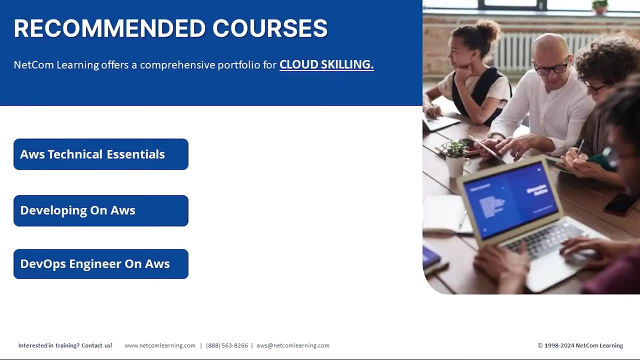 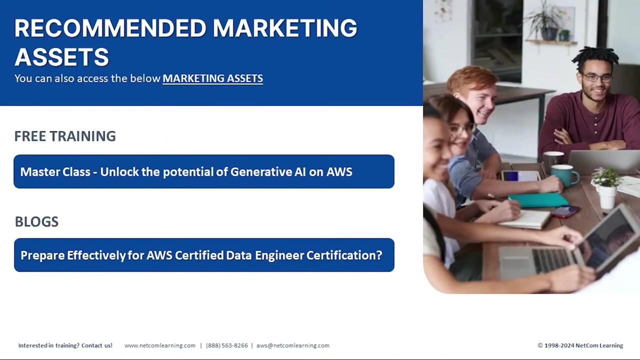 They encompass people, process and technology training. Today's presentation is from the cloud practice area. NetCom Learning offers a comprehensive training portfolio of courses for the topic being covered today. Our upcoming classes include various trainings on the given courses. You can also access a variety of marketing assets, such as the free training and blogs, by clicking on the available event handout. 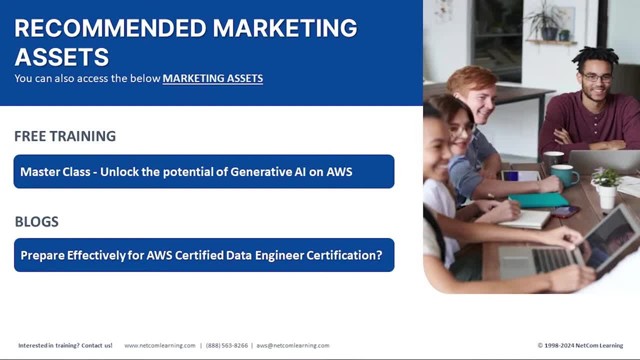 Thank you. You can also access a variety of marketing assets, such as the free training and blogs, by clicking on the available event handout. You can also access a variety of marketing assets, such as the free training and blogs, by clicking on the available event handout. 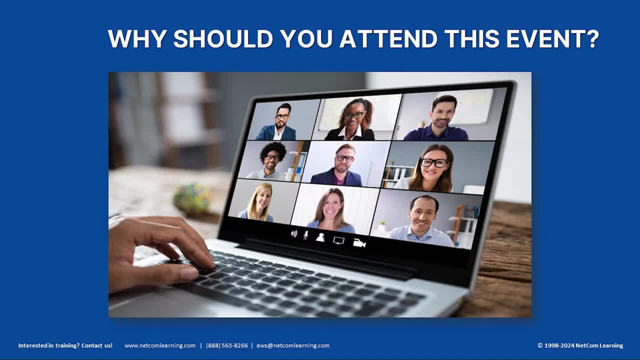 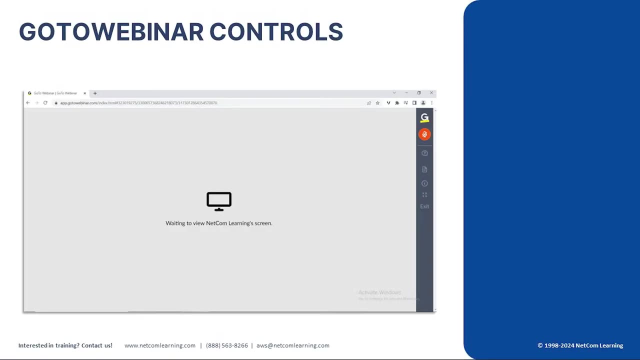 In this event, we'll learn the basic practices to help your team master the most common DevOps patterns, practices and tools required to develop, deploy and maintain applications and services at high velocity on AWS. And now I would like to give you a quick overview of the logistics before we get started. 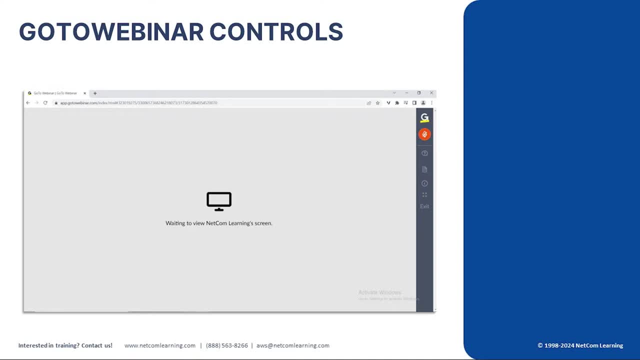 To begin with, you do have the option to view in full. You can view in full by clicking on the full screen button on the right side of the GoToWebinar viewer. Simply hit the escape key to exit the full screen. Everyone has been muted, except for our presenters. 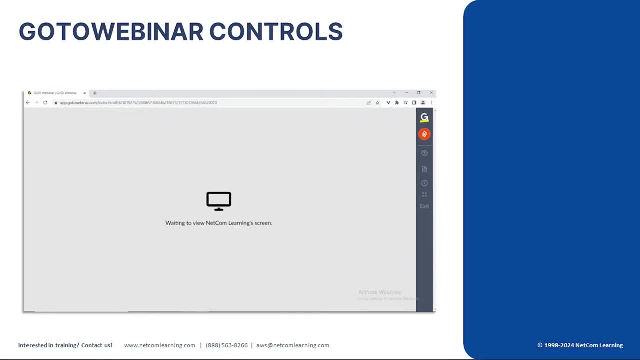 Feel free to submit any questions you have for the presenters here in the questions pane and we will address them at the end of the session. And, to get the best out of today's events, we've included the slides, courses we talk about and marketing assets in the handout section of your GoToWebinar. 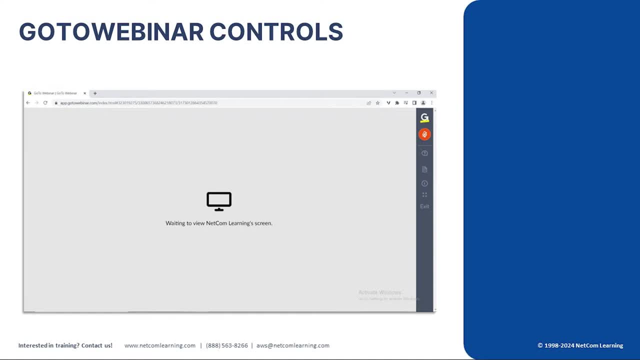 You may refer to them at any time to get a better understanding of today's topic, And we do realize that some of you may have to leave early and want to let you know that, as you do leave the session today, you will be presented with a short survey. 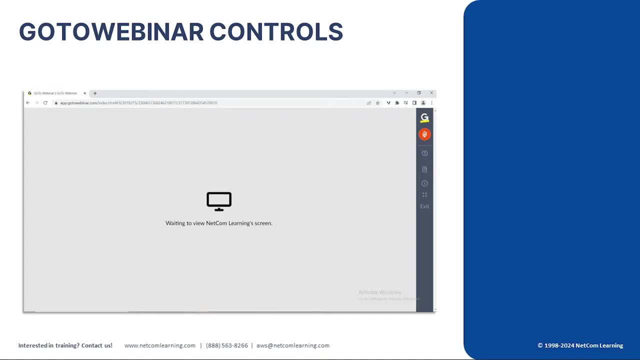 We would like to request for you to take a quick moment to participate in that survey. Your feedback really helps us understand your learning experience and improve our future sessions for you. The survey ends here. Your answers are measured on a scale of one to five, five representing outstanding and one representing poor. 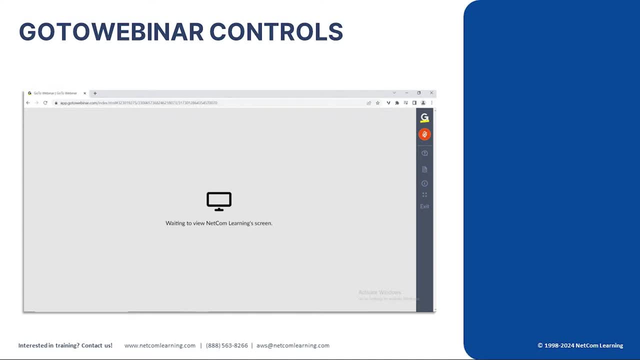 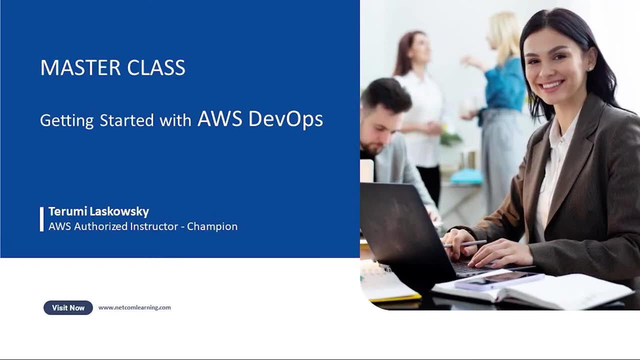 And now I'd like to pass this over to our trainer to present today's topic. Hey, Tarumi, thank you so much for joining us today. Hey, thank you so much for inviting me, And hi, everyone, And thank you so much for that introduction, by the way. 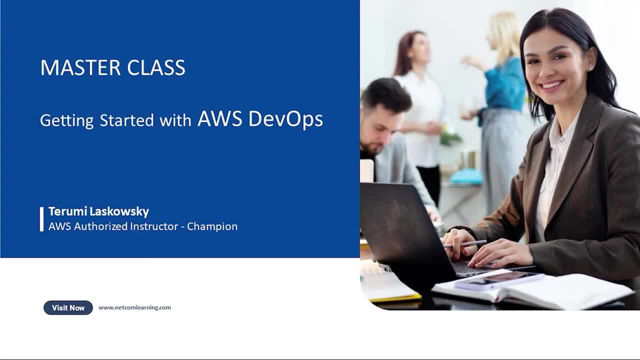 I hope you can hear me, OK, And also I'm kind of sharing my screen right now. Can you see the screen? OK as well? Yes, you are audible and we can see your screen. Everything looks great, Great. Thank you so much. 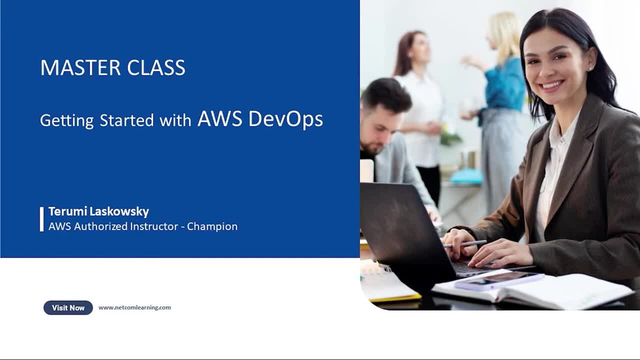 As I say, hello everyone. In fact, let me just say aloha. I'm in Hawaii right now And this is my pleasure giving you the masterclass, And the title of the class, of course, is a getting started with AWS DevOps. 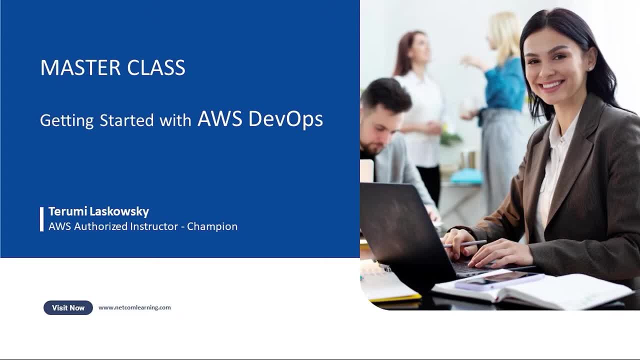 And, by the way, this webinar Will last actually has a couple of sections, So if you have any questions at all, please feel free to post your question any time at all, and I'll definitely get to them when we have the time for that. 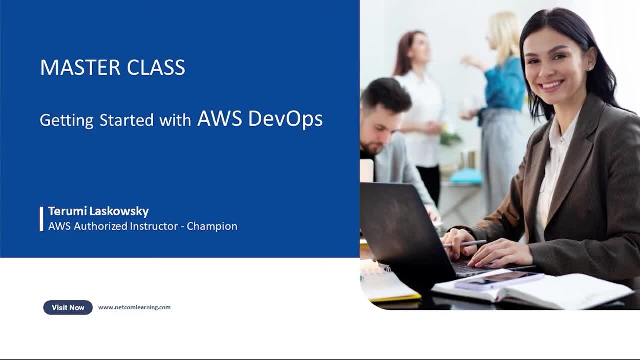 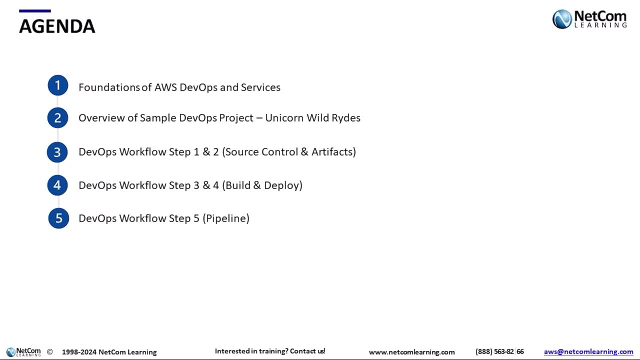 OK, so let us get started. OK, the today's session, as you see, is on DevOps and it's specifically on AWS DevOps. So let me show you the agenda for today. There are five sections within today's webinar. 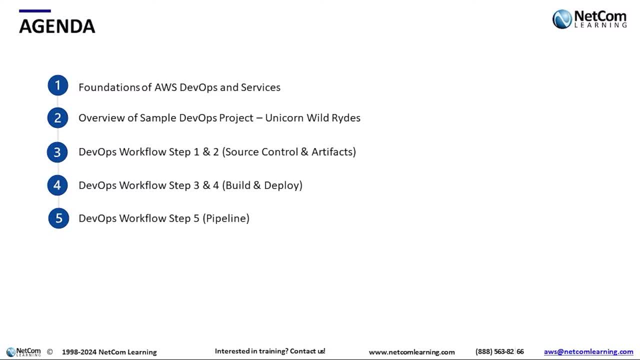 The very first one is a foundational topic, So it is a foundation of AWS DevOps and AWS DevOps services. So I will be covering what is DevOps, That is, regardless of any type of cloud vendor and such. I'll introduce to you what DevOps means. 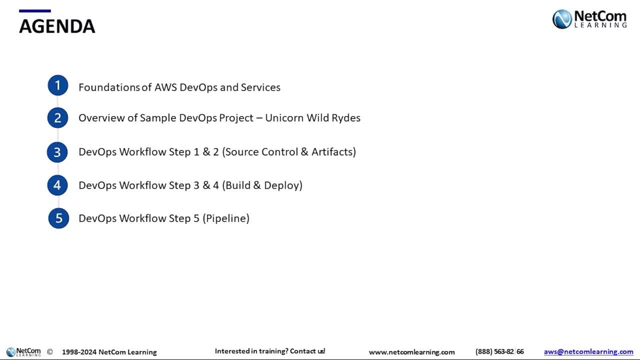 Then, on the- The latter half of that- I will introduce you what AWS means by DevOps and some of the services that they have to offer for you. The second topic is: I thought it might be nice for not just to hear about the concept but to actually see DevOps in action. 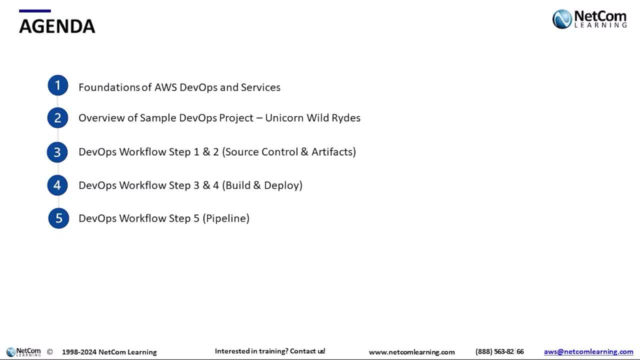 So I have a sample project ready for you that you can just go and follow along, And it's called the Unicorn Wild Rides. So it's like a little Uber, but instead of a car, a unicorn. Unicorn will come and get you right. 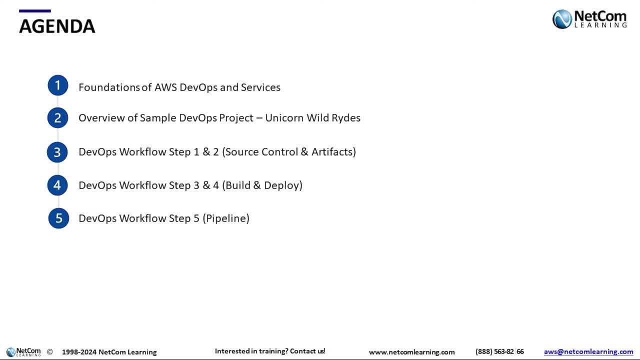 So that's going to be the application that's actually created by AWS, So it's available if you like to do it on your own at a later date And within that demo. there are a couple of sections, So the first part is the DevOps I have in here. workflow step one and step two. 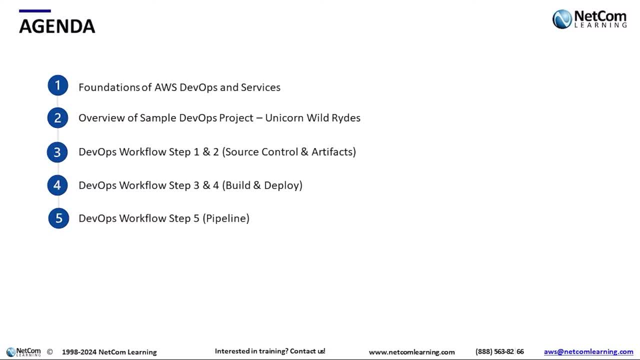 So this is the very first step of DevOps, which is to specify the source control service, And then we'll talk about something called the artifacts. that will come in my first part of the discussion. The fourth part is step three and four, which is arguably the very core of DevOps process, which is the build phase and the deploy phase. 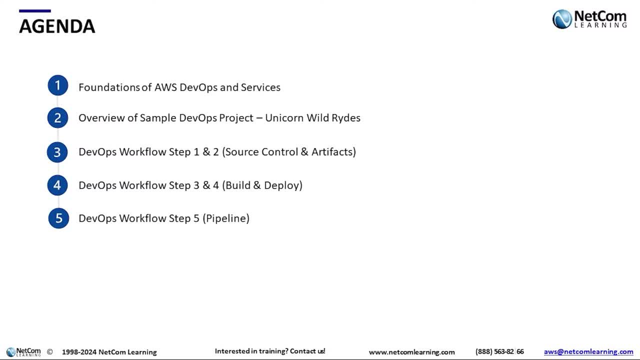 Then on the last one. this is where you actually get to see the end product of DevOps, which is the pipeline phase and actual deployment and automating the whole process. So there you go. So that's going to be agenda for today. 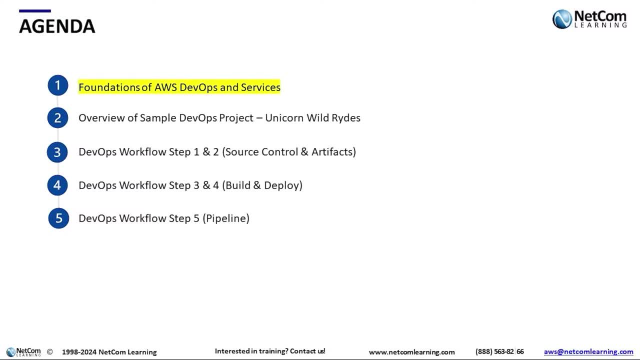 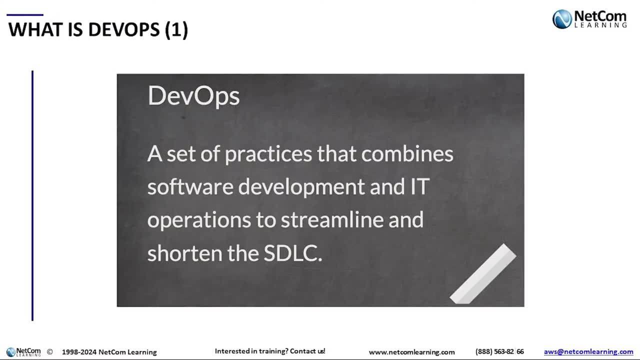 All right. So let us go ahead and get into the first part, which is the foundation, The foundation part. Okay, All right. So here we go, Just to get started right from the beginning. right? What is DevOps? Okay, 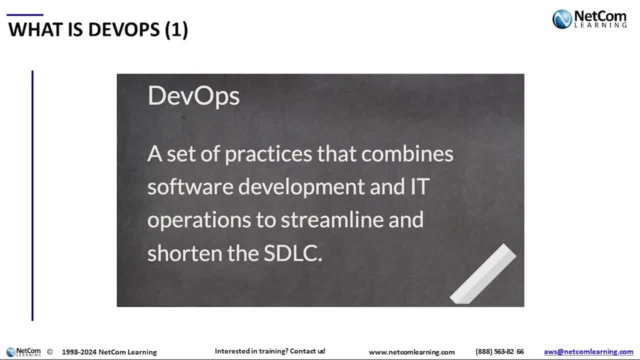 So there you have it in front. Let me go ahead and read that for you: A set of practice that combines software development and IT operations to streamline and shorten the SDLC. Okay Now, if you are familiar already with development process or operational process, this may sound okay to you. 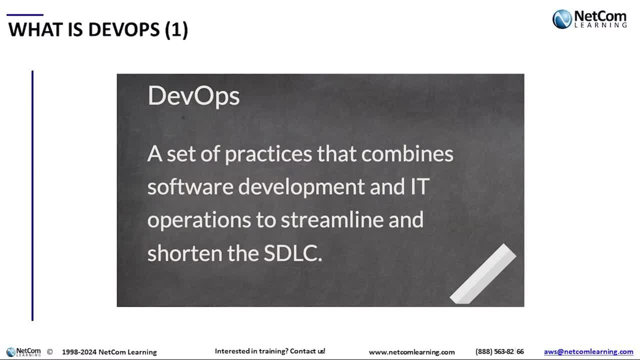 But if you're brand new to the topic, you know, you may say ah, but you know what's DevOps, You know what do those terms mean And also what is this thing about. you know software development, IT operation process. 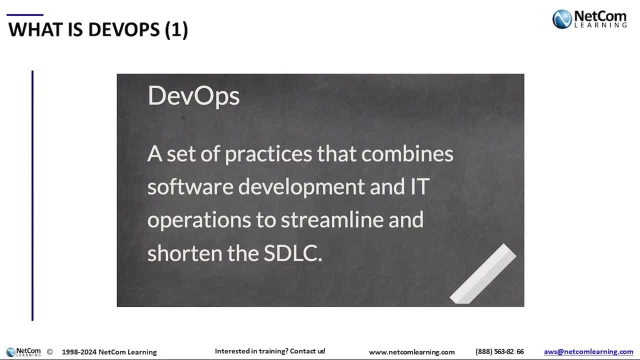 What does that mean? to combine them together, Like how come they're not together already? Or maybe you know you may have some questions about what is this SDLC thing right And you know why do we need to shorten the SDLC? 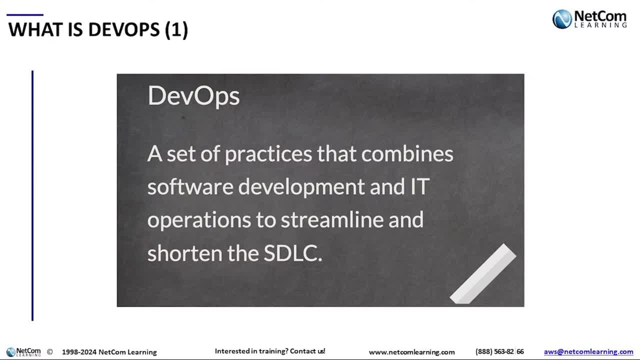 Okay. So we'll definitely cover that part. So kind of keep this on the back of your mind, And we'll revert back to this definition a little bit later on. So first thing first, let's go ahead and talk about what this SDLC thing is all about. 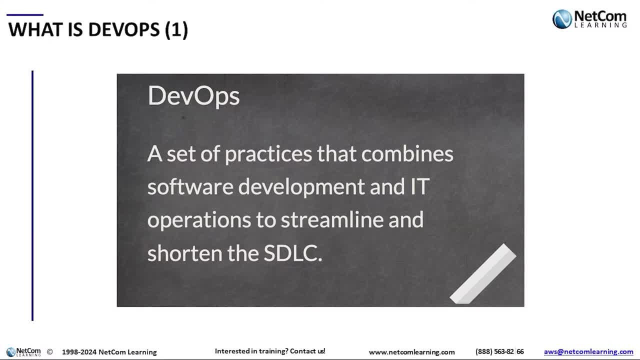 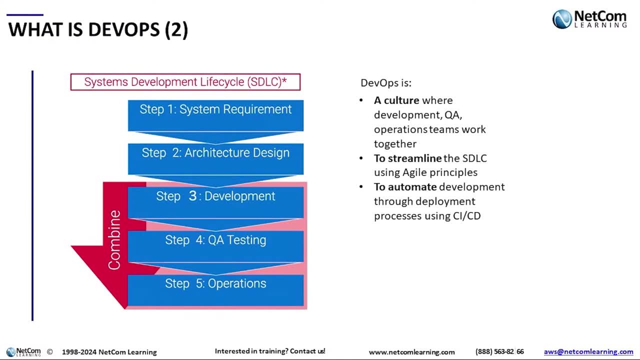 Because that seems to be key to this definition. So SDLC stands for a couple of meanings. Some people call that software development lifecycle, right? So SDLC, The one that I have in front of you, is systems development lifecycle. They're just a little bit different, but not too much right. 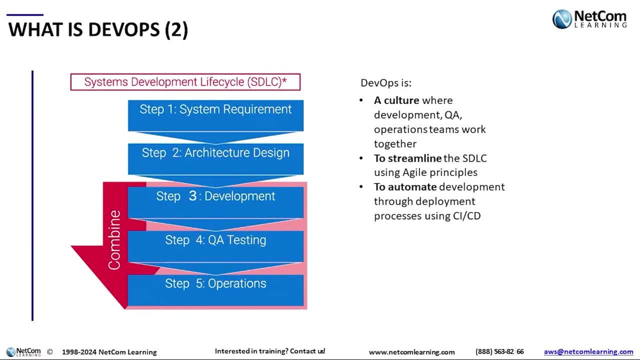 And the reason why I chose systems development lifecycle, because it actually includes more parts where you have the step one and step two, That part. sometimes it's not part of the software development lifecycle, But I just want to kind of show you, you know what a company may go through. 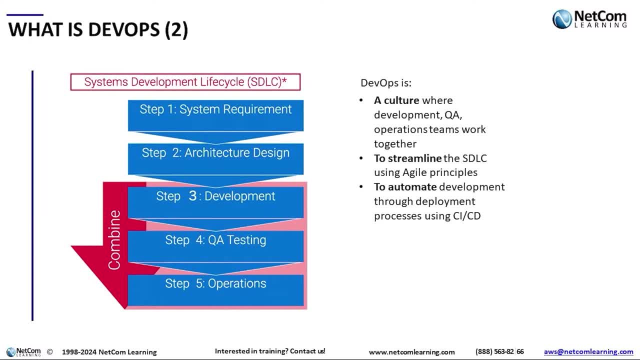 when they are trying to come up with a new product, new software product, right. So let me explain briefly. When a company endeavors to create a new product, right, You have to kind of consider the reason. why are they doing that? Well, hopefully it's for their business, to increase the customer base, right? 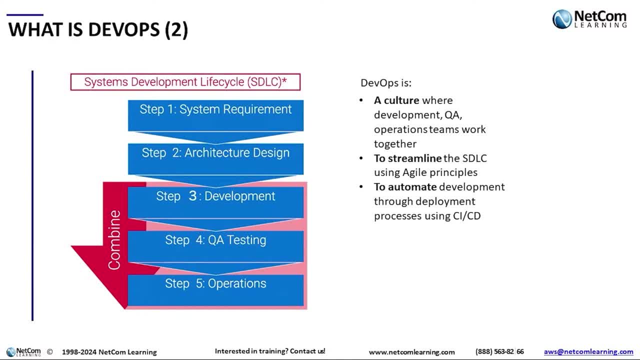 To give better products to their existing customers, et cetera. right, So it should be a business reason. So this is going to be the systems requirements document that states what a product is supposed to look like. Then, when it comes to IT, information technology department, 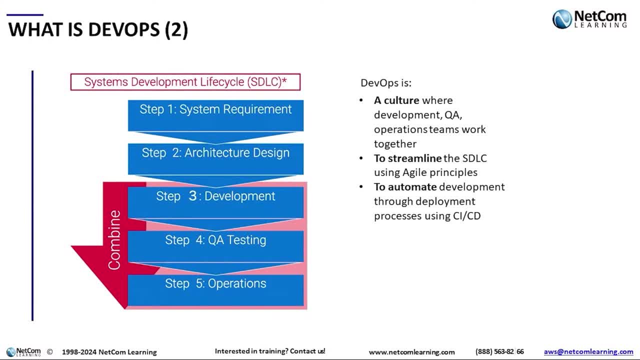 now they have to turn that business Needs and wants into something that is a systems needs and wants. So that would be a systems requirement document. That's why we have step one. Then someone will take that requirements and then create a architectural design from that right. 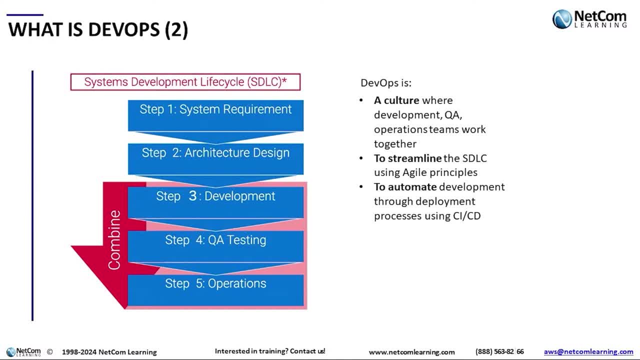 So those are the very first steps that you know one takes in SDLC. Then, once the architect has finished with their design, usually that's passed to a development organization. Now the development organization could be programmers. It could be people that purchases software and integrates them with existing software. 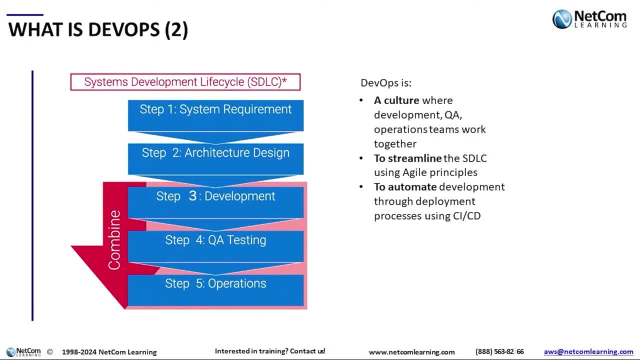 Regardless it's where they create that new product or new service. Then before that could be given to a set of customers, it needs to go through some rigorous testing, So that's called the QA testing or quality assurance testing. Then, after the product passes the quality assurance testing, 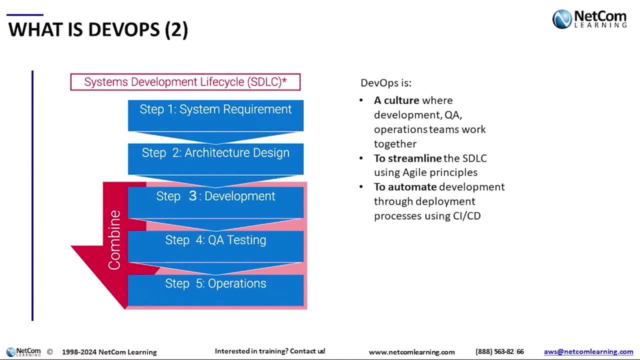 then now that is ready to be deployed Or made available to what's called a production environment. So production environment is the actual environment where the customer will be using it, right? So if it's a you know Internet site, sure, right? 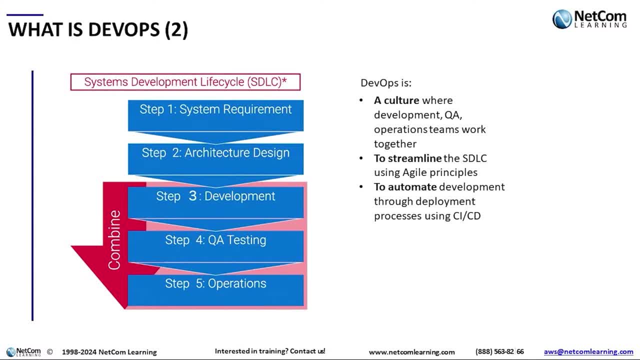 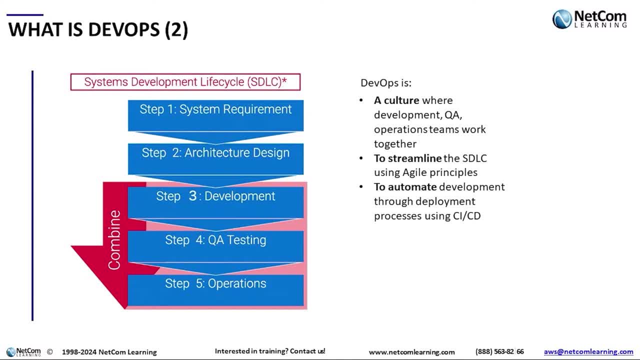 Maybe they'll have to patch it. They may have to make some tweaks, changes right, Listen to the customer and see how the application is going. So those are all the things that are included in the operation. So that is the very short description of what an SDLC is. 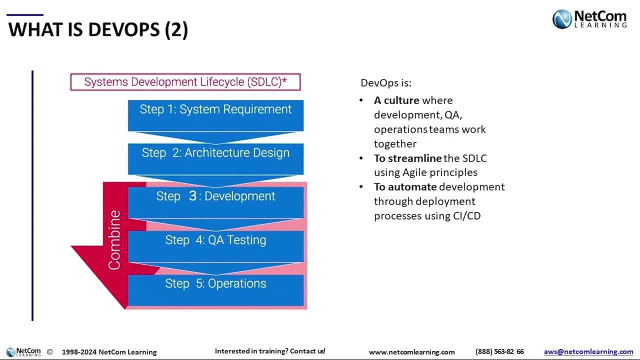 So I have in there the red arrow that says combine. So this is the part that the DevOps is trying to streamline. So anything that created in the development all the way to where it makes, where it's being made available to the end customers. 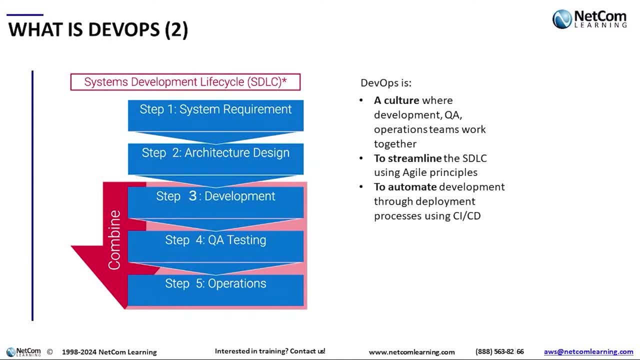 This is the process. This is the portion that DevOps is trying to do. you know, make a streamline, But we'll talk about why that is the case. But, as you see, there are three points on the right right. So DevOps is right. a culture where development, the QA departments, operations team work together. 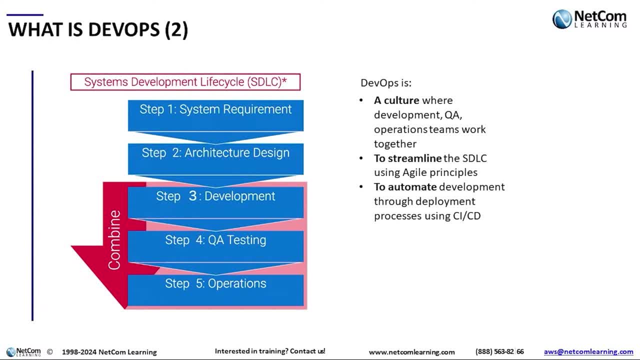 So we'll talk a little bit later on in about a couple more slides, why they're not working together. They're not working together in a lot of cases, right. But if you're trying to streamline stuff, right, streamlining means, you know, going to the minimalist option. 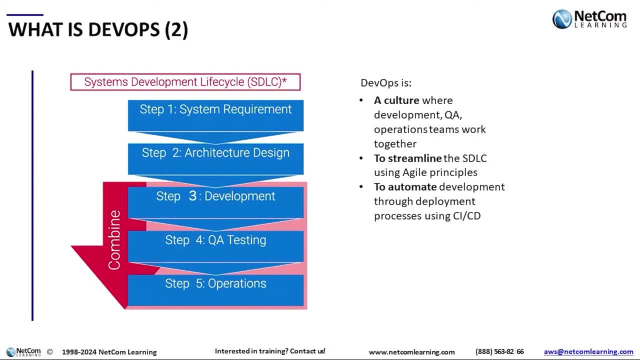 getting rid of all the frills. you know bells and whistles so that it can go fast. So people, all the different people that you see on the SDLC, they need to work together so that there are no barriers. You know there are no excessive friction as the solution moves from one stage to another stage. 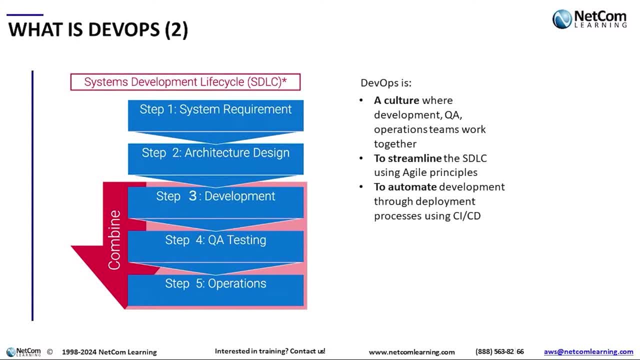 So that would be. we'll talk about that. We'll talk about the culture. I'll have a couple of slides on that- To streamline SDLC using Agile principles. Now, some of you may be familiar with what an Agile is. Agile is a concept that came up around early 2000.. 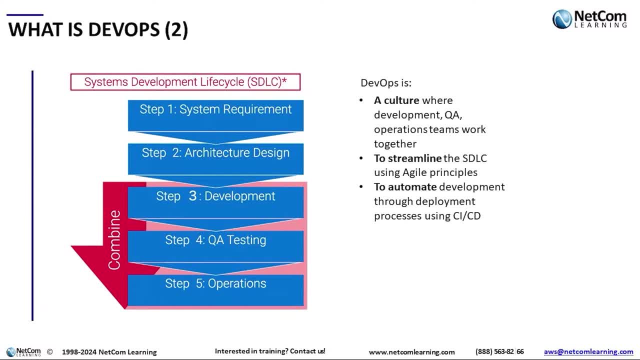 I think it might have been 20, I would say yeah, without naming the actual year because I may get wrong on that one, But it was in the early 2000s where a group of people came together and said: look, you know. 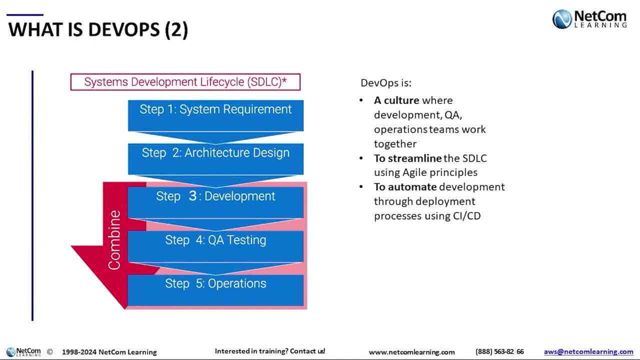 the way we do software development is: you know, it takes too long, It is just too cumbersome, too heavy. So let's make it light and let's make it fast. So the commonality here is streamlining, that is, making things fast. 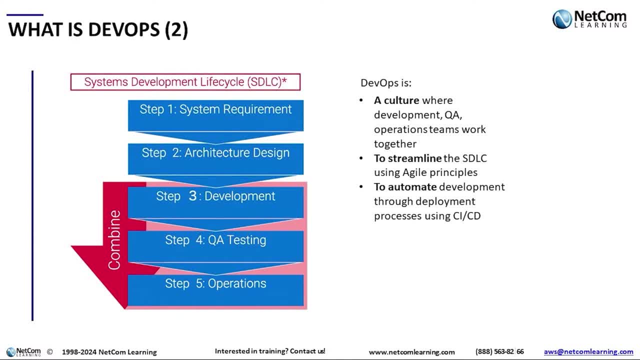 And last but not least- and this is the part that we're going to be spending a lot of time on this webinar- is to automate, So the automated development through deployment process using what's called the CI-CD. Just a quick explanation of the term. 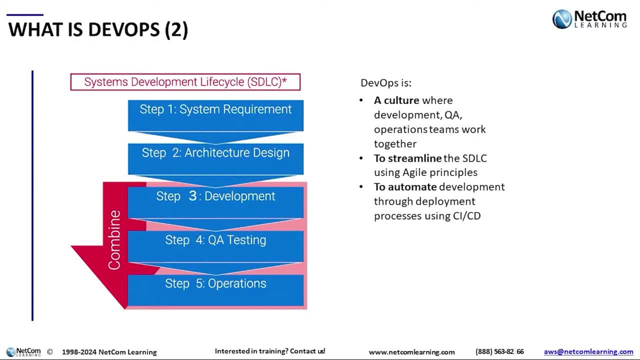 CI stands for continuous integration And CD stands for continuous deployment Or continuous delivery, which I have a whole set of new slides over, But just at this point just understand that you know CI-CD has something to do with automating this whole process: the step three, step four and step five. 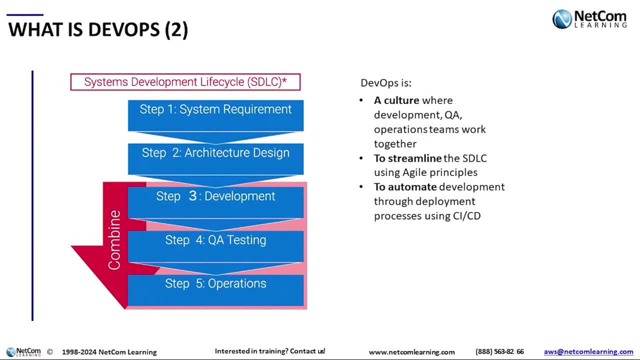 So anyway, so that is DevOps, And there are mainly three concepts that are involved with it. OK, so, like I said, if you have any questions, just go ahead and put it in the chat. All right, So now we have some kind of idea as to what it is. 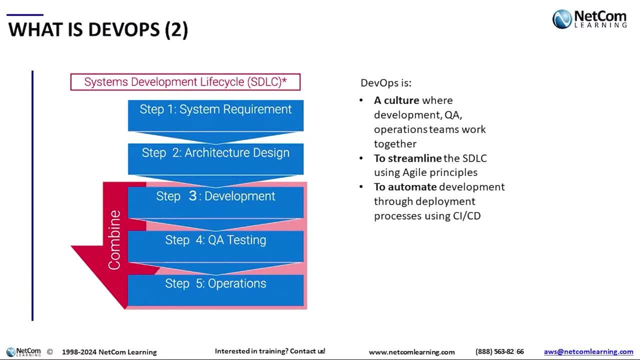 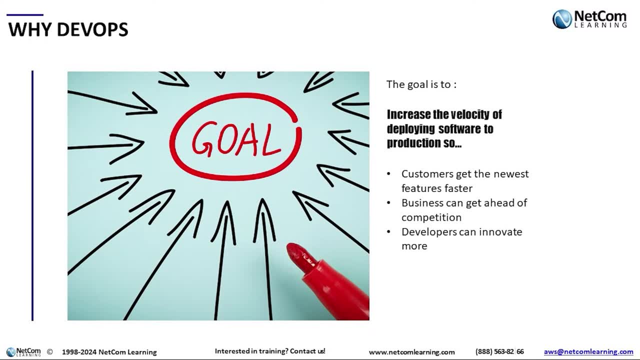 OK, But why do we do? Why do we do that? OK, So why do we have to make things faster? So, and here's the thing, The goal right of the DevOps is the following: To increase the velocity of deploying software to production. 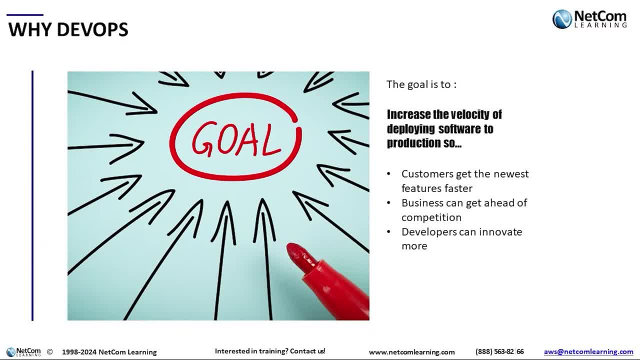 And put it another way: when you create something new, make sure that new feature or new solution gets to the hands of your end user. Make sure that new features get to the hands of your end customers as quickly as possible. OK, And I can attest. I've worked in project management before and I've been involved in projects that took like months, if not years. 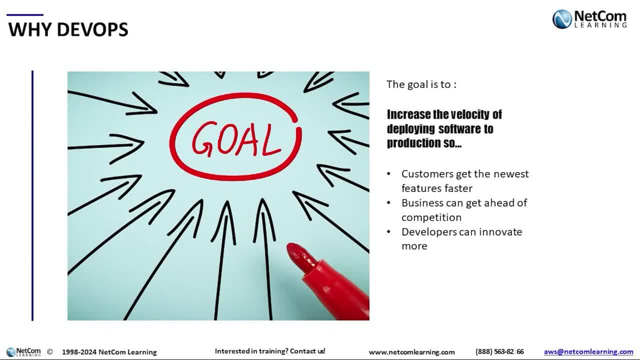 OK, So that's like OK, so someone come up with a good idea. You know, they make a request to the IT And it takes like months for that thing to be done and for the end user who asked for it to actually, you know, play with it and start using it. 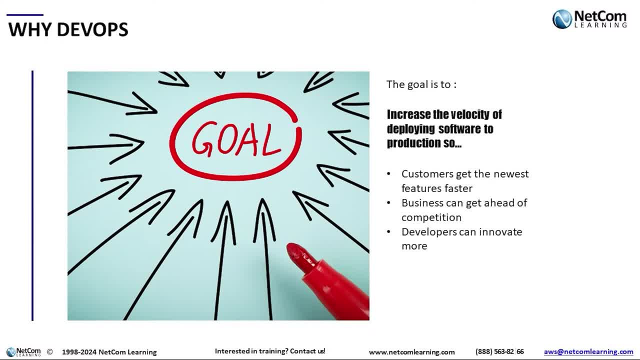 But in the time that we live now, that is just way too long, Right? And so why do we want to make it fast? Why do we want to increase the velocity of this whole process, Right Is? I've pretty much written in there three points. 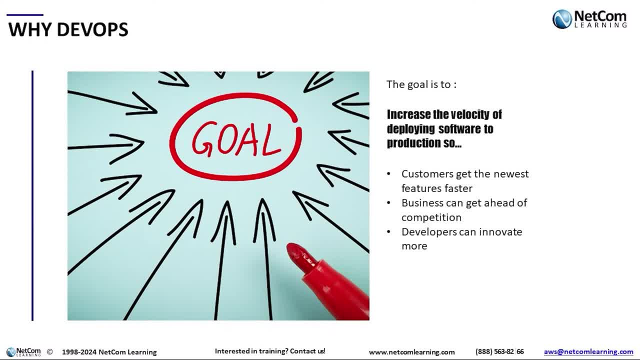 Customers get the newest feature faster. So that means customers will be happy, I hope. OK. The next one is the businesses side. Right, Because after all, businesses are the one that's paying for this development And they can get ahead of the competition. 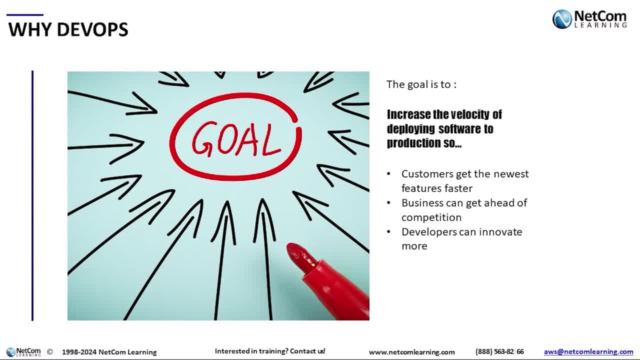 Right And I think a lot of the companies are living in the world where there are competition, where you know they're fighting for the same group of customers And the more you satisfy and give customers a great experience and great products and services ahead of the other guys. 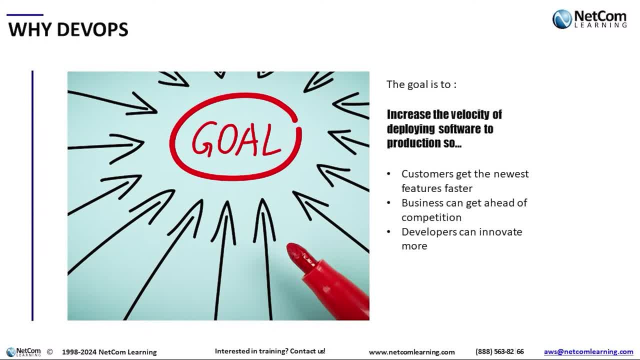 Right That you will be ahead of the competition, And then I'll put that third part in there. Developers can innovate more, And that may not be as straightforward as what you know, what you may think Like. why is it making the development process faster? 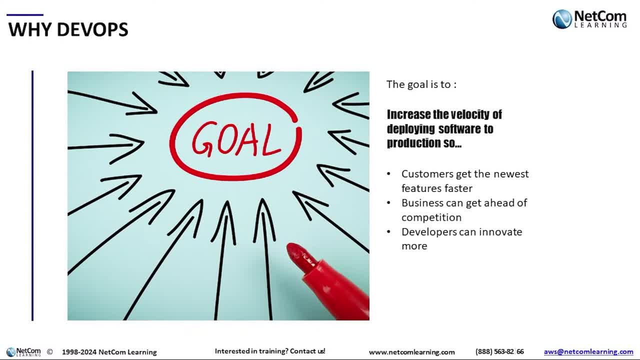 Right Is going to give developers more time to innovate, OK, So once again, I'll cover this, but this is actually really an outcome of DevOps as well. But anyway, I think the first two points are pretty easy to understand. 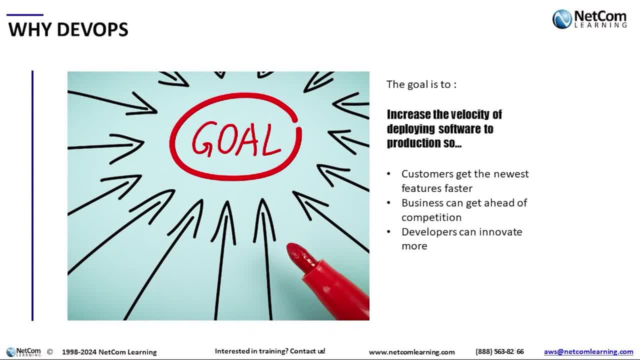 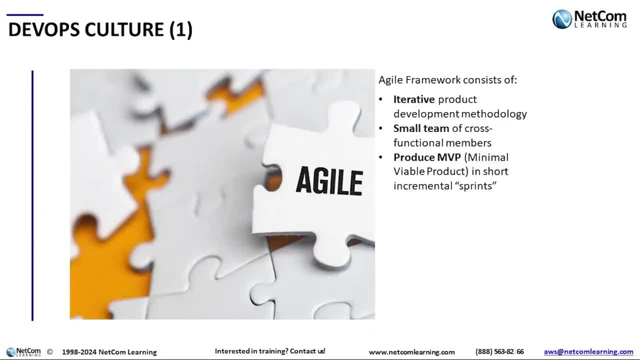 Right, So that's why a lot of companies these days are taking on the DevOps practices, Right? So let's let me go a little bit more into some of these terminologies. OK, So we talked about the culture, Right? So now let's talk about culture. 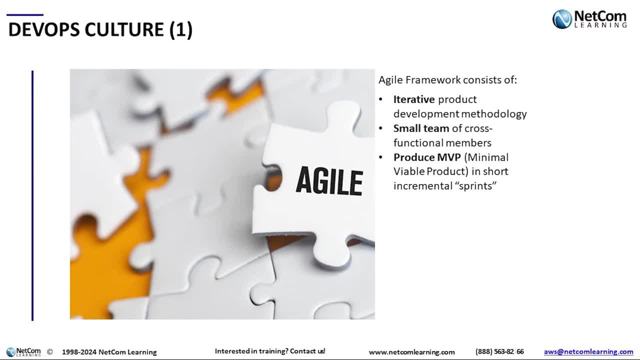 I have a couple of slides on this. So, on DevOps culture, And I mentioned that it's about being agile Right Or taking in agile principles. So here I have a short definition of what an agile framework, or you know, like a blueprint. 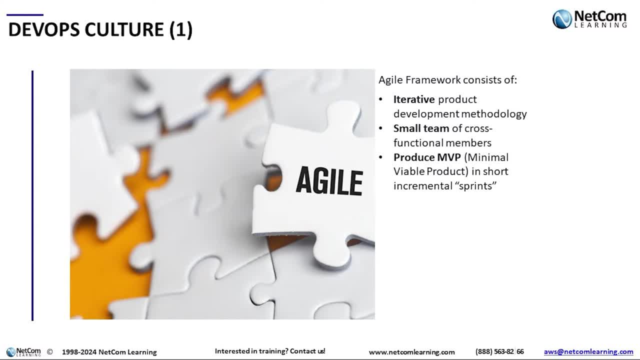 Right On how agile is applied to DevOps may look like: Yeah, So you know? I think the first one is that it's a product development methodology. Right, So it's an iterative product development methodology. OK, So iterative means you're repeating things over and, over and over again. 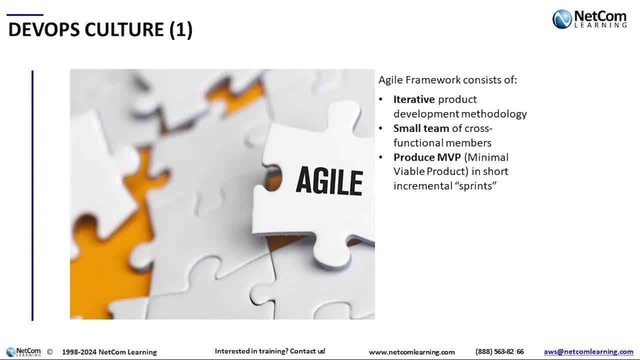 Right, And it's usually. when we say iterative, we're not talking about the first cycle going through like it takes like a year. Right, It doesn't take like a month, OK. So iterative means short period of time and you are producing something. 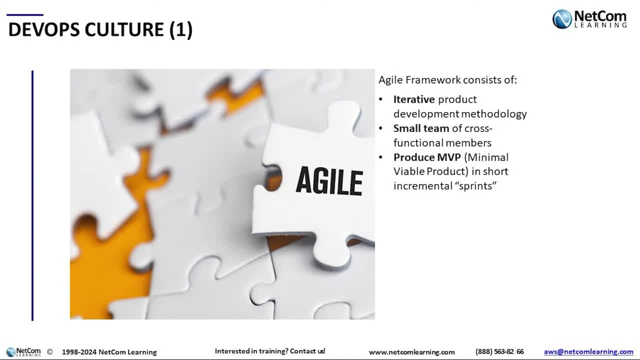 Right, Because it's a development methodology And normally a very tight loop that you go through. The amount of development that you can do is also limited as well, Right? So it's not, you know, in traditional the kind of like, let's say, financial organization. 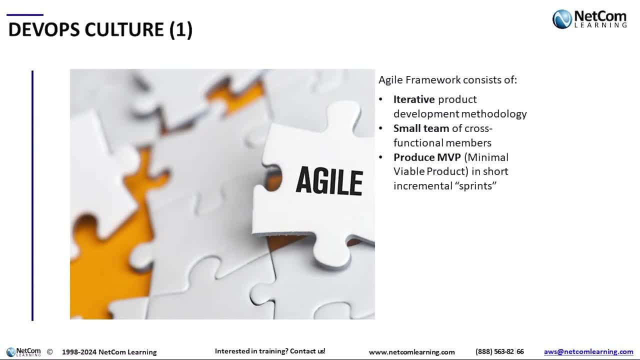 creating a new application. I've seen cases where they have like hundreds of people working on it- Yeah, Like hundreds of developers- And it was taking literally like months maybe, if not years, to create this big product. Well, that is not going to work in the agile framework. 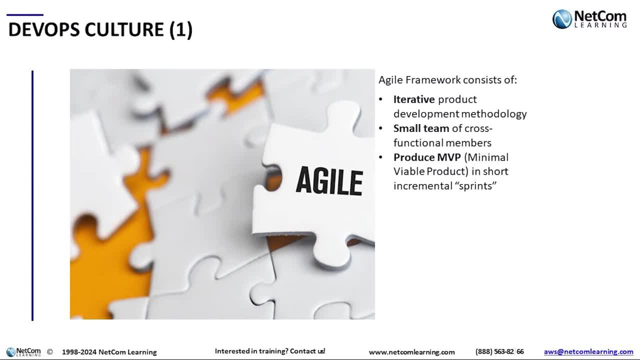 Not that well anyway, OK. So. so the teams have to be smaller, The actual software product have to be smaller, so that the process takes shorter. And then, instead of taking months, you know, you will start to deploy things in small chunks. 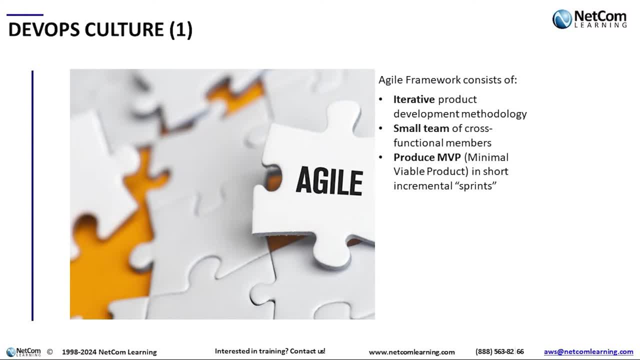 So that would be the iterative product development And, as I mentioned, it's usually small teams And what's important here is a cross functional teams. So cross functional team usually means OK, what does that mean? Right, Because in development you've got developers. 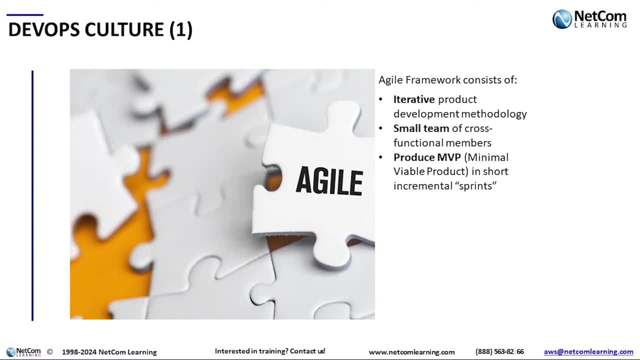 Right. What kind of cross function do you have? And actually not Right. Developers are developers. That's not a cross functional team. So the cross functional team usually means that you have other people with other expertise in your team. So, for example, maybe a QA tester, quality assurance tester- may be in your team. 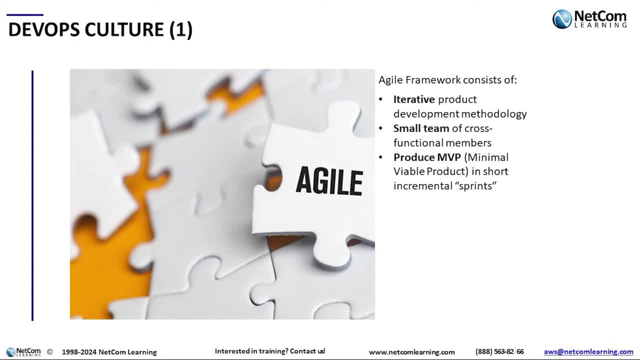 Maybe systems operations person may be in your team, Maybe security people may be in your team, Or maybe you are yourself. Let's say, if you are a developer, you have been trained, let's say in security, or you have trained in systems operations so that you have skills in multiple areas, not just. 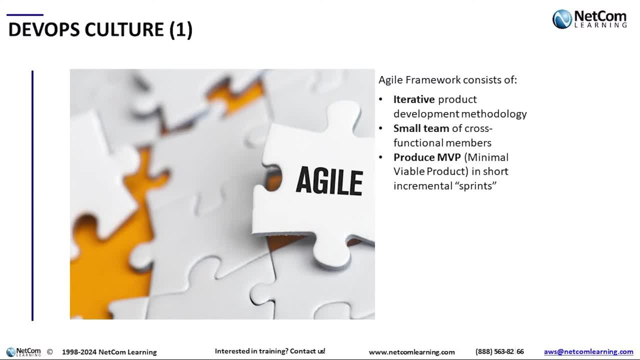 development, OK, And these, these jobs that I just mentioned is all part of the SDLC. if you remember, Right, Some of the people that kind of come together in the SDLC And, last but not least, producing the MVP Right. 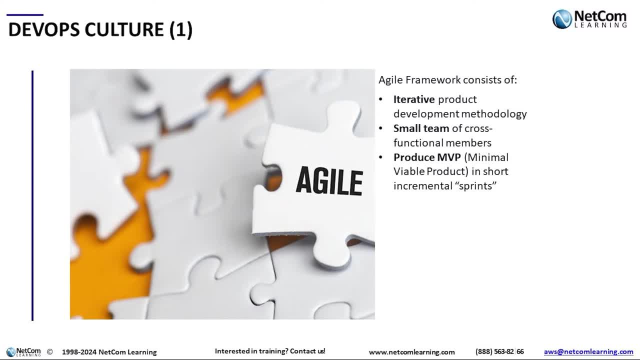 So the MVP stands for minimal viable product, and minimal viable product refers once again to small piece of product, Product code program. whatever you want to think about it, that actually stands alone. That is, it can do anything it needs to do all by itself. 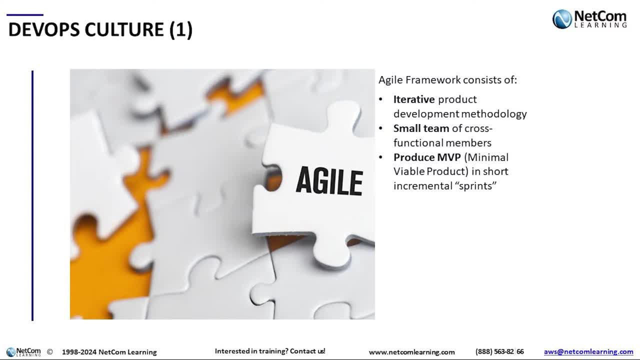 So that's usually what is what an MVP is, And the having your incremental sprints. So the sprint is the, the process that I told you about the iterative process. They're usually called sprints in Azure methodologies. So there you go. So these things you will see in a lot of DevOps. 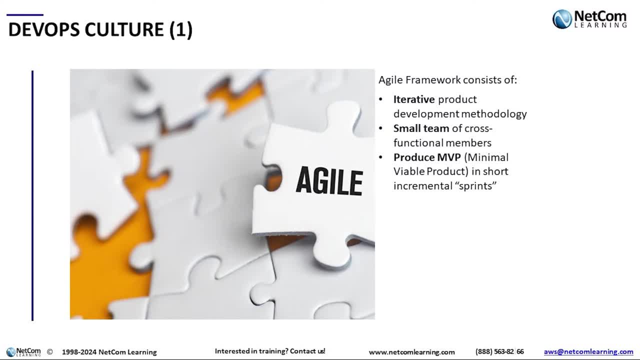 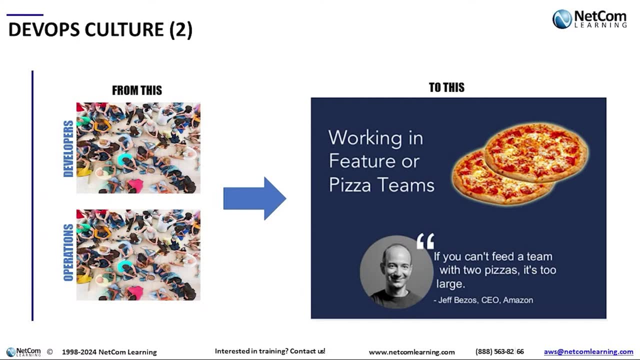 Being applied. So that is part of the changing of the culture when companies are moving into DevOps culture. So the second part here is this: It has a you know, something to do with that cross-functional team. So if you take a look on the left, right where I have from this, 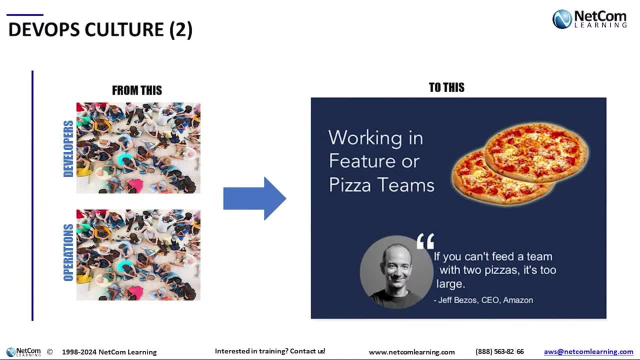 So under that I have two sets of bunch of groups of people Right, So one is the developers and the other one is the operations folks Right, And it's very common. You know I've been in IT For a kind of long time. 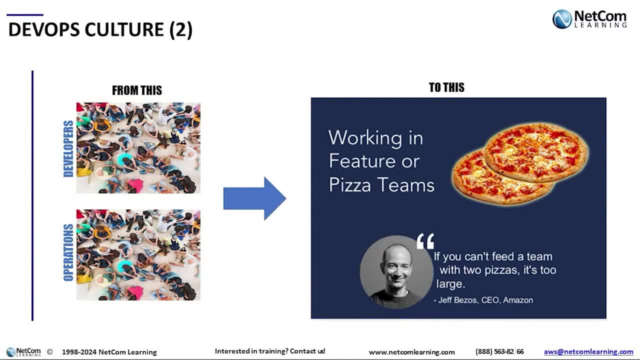 And it's very common for these development and operators to not get together. So it's not that they don't like each other, It's just that they have a complete different sets of jobs. Right Developers create things and operations people maintain things. 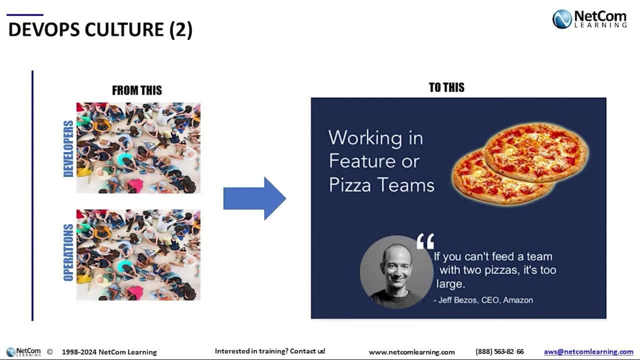 And you know there was really no major push to bring these two groups of people together. So so they. I'm sure that in a lot of companies still this way they're highly siloed And you know they're used to working. 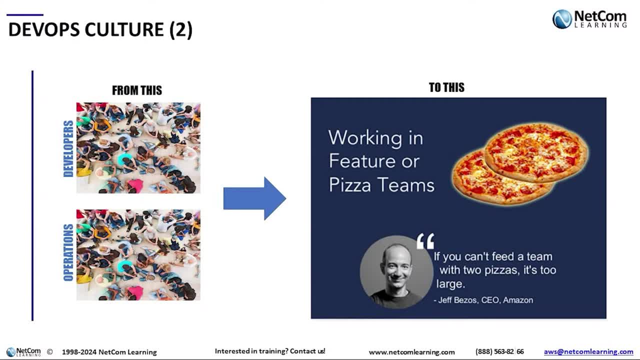 They're used to working on their own, not together, But with DevOps. the culture has to change. So if you see on the right, you see the comment of Mr Jeff Bezos, the CEO of Amazon, saying: hey, if you cannot feed a team of developers, right with two pizzas, it's too large. 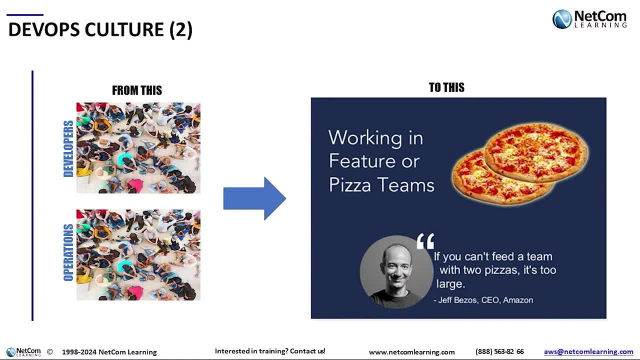 OK. so so you hear in the AWS DevOps practices a term: pizza teams or two pizza teams. So what a two pizza team is is exactly that. That's how large your development team is going to be. Remember the cross-functional team. 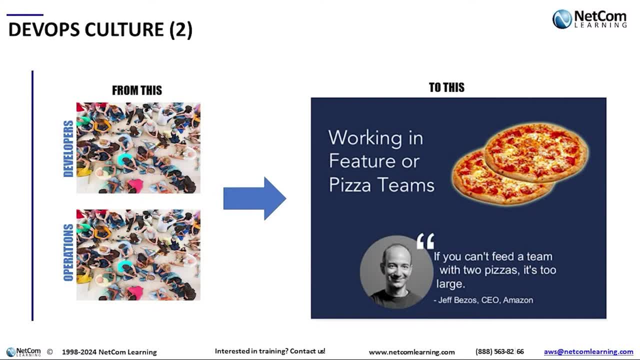 So that development team needs to be around four or five, six people, no more. Right, Just enough to feed for lunch. You know, just order two pizzas and that should be enough. So once again, the culture is smaller, Right, And then cross-functional. 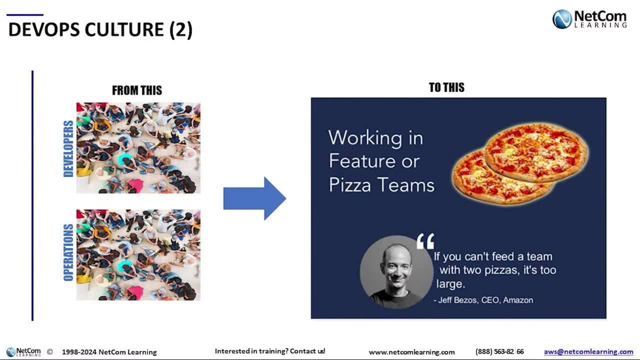 So within these two pizza teams of these, you know four or five people. they are all cross-functional members. OK, So they're not. they're not going to say: hey, I'm just a developer here, Right, So I have no idea what security is doing. 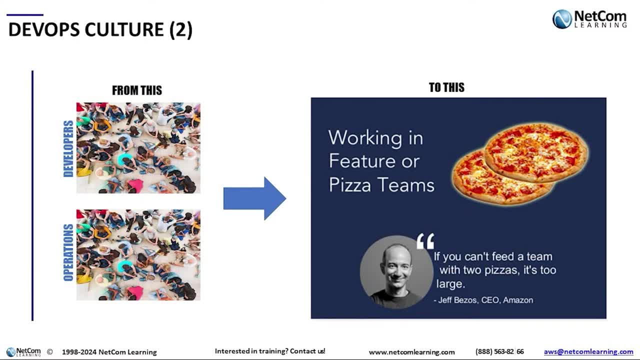 So you know that's somebody else's job. Well, that's not. that's not the idea of a two pizza team. So everybody is able to hopefully be able to- to at least be intelligently talk about, let's say, security, talk about testing, talk about operations, even if your main expertise is in development. 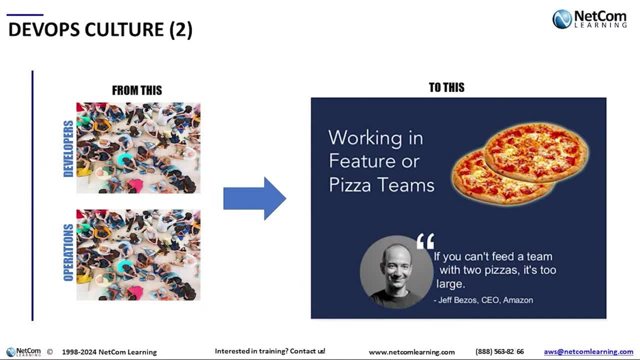 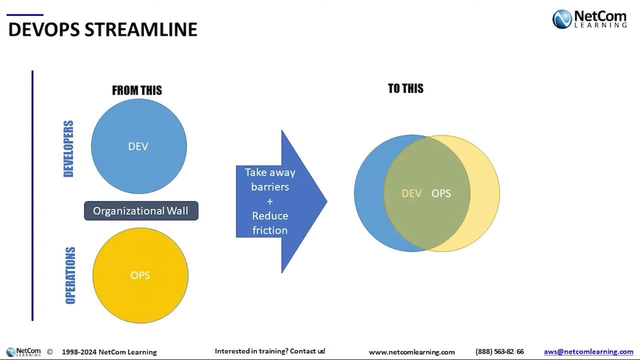 OK, All right. Two pizza teams, OK, so now you know what that is. So let's go into the two pizza teams. Let's go into the the next concept, which is streamlining. OK, so streamlining looks like this: 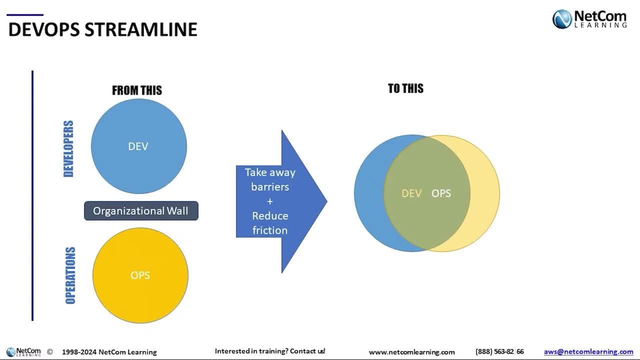 So, once again, if you look on the left hand side, it's from this to this to the right. OK, so from this states that you have two separate teams. You have the development organization and then you have the operations organization Right And, and a lot of times in my experience there is definitely an organized organizational wall. 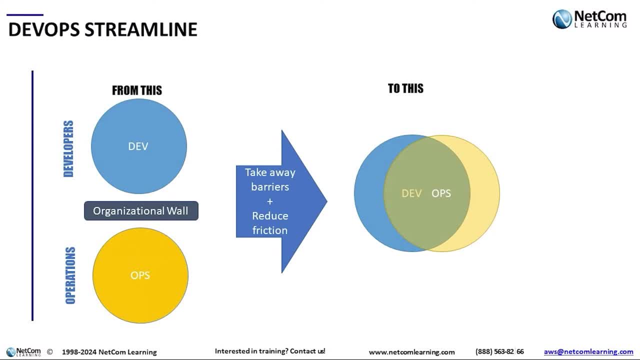 OK, that is between these two groups, because, one, they're under the development organization, One, they're under the different management And two, there are different mandates that they- you know, their jobs- are completely different. And third- oh, by the way, I probably didn't tell you- I'm a security. 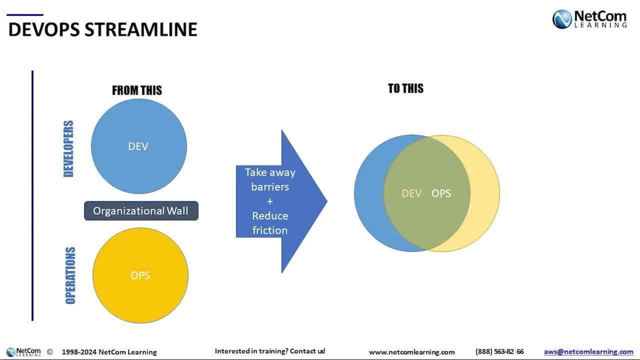 I have a security background. from security perspective, We wanted these people to be separate. Right, We wanted them to be separate for conflict of interest purposes. You know, we want to keep any irregularities that may happen in development organization to not bleed in to the operations. 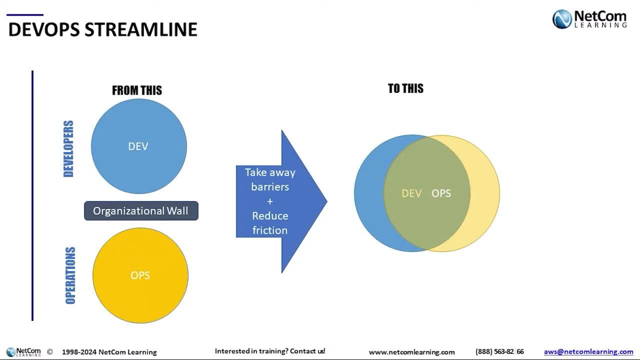 And vice versa. Right, So it was for accountability purposes, It was for responsibility purposes. that it was. it was easier to manage these two groups if they were completely separate. But that is really not conducive to speeding things up. Right, Because more separate you are, more coordination you have to do. 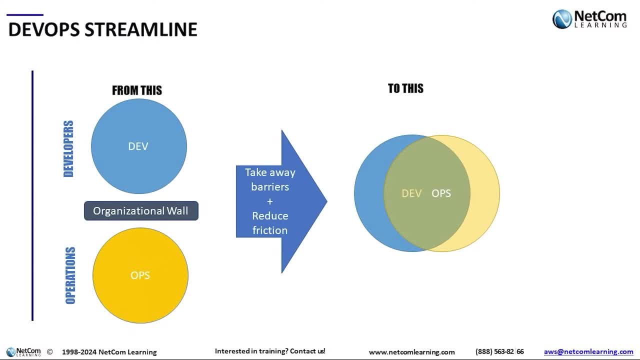 After all, developers are the one that's creating the product and the operations are the people that has to run the product. So how do you pass this And product from developers to the systems operation? So if you have the organization, organization law, the way I kind of refer to this, you know, let's say, software as being like a hot potato. 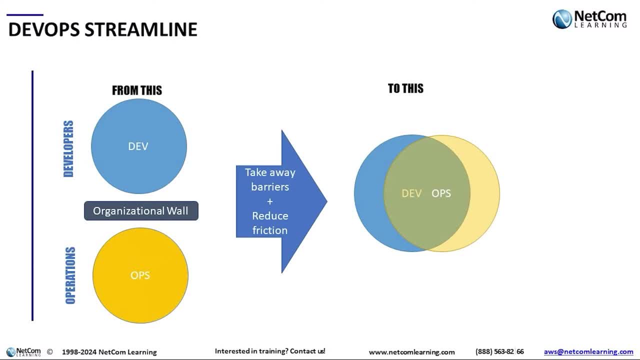 Right. So the developers finish with this hot potato, Right, It's nice and piping hot. It's too hot, So they'll toss it across the wall and say, here, here you go, OK, And then on the systems operations side, they're waiting for this hot potato. 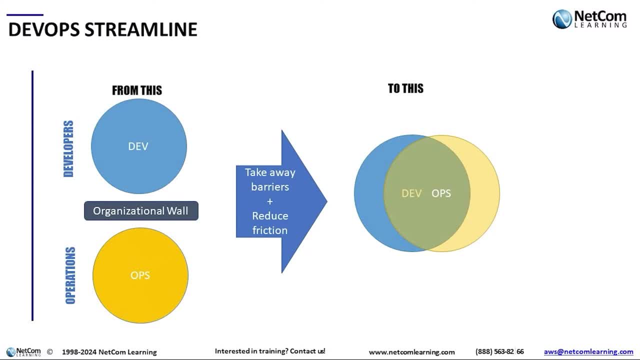 And that catches that, you know, says OK, well, that's kind of hot, kind of fumbles around with it and then puts it on the operations. So that's not really An efficient way to, you know, to transfer the responsibility of one product to another. 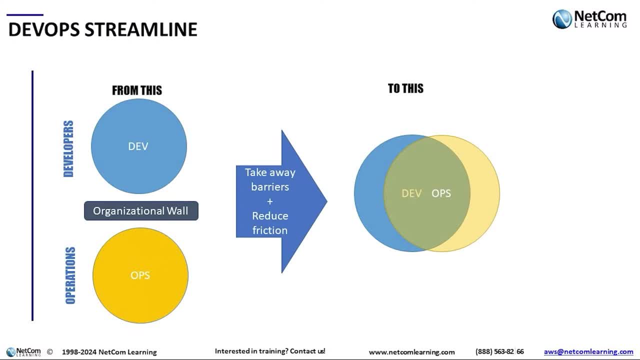 Right, Another group, So DevOps, seeks to take away these barriers. So take away most of the organizational walls, if they can. you know completely. And then the main point here is to reduce the friction between these two groups. But what are we reducing the friction of Right. 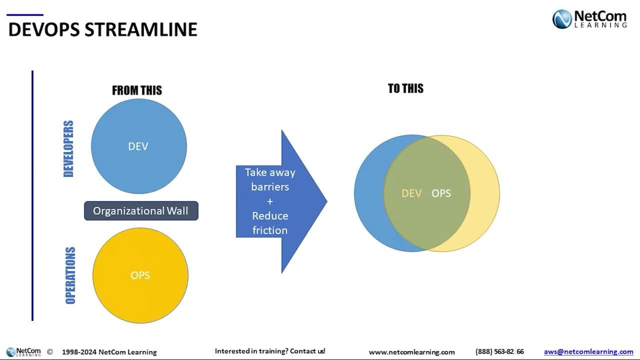 What you're actually reducing the friction so that that hot potato Right That can actually flow right from one organization to another Right, So that there is no You know process procedures, time wasted as the developers finish with this product that they can go smoothly into to the production environment, which is in the operational environment. 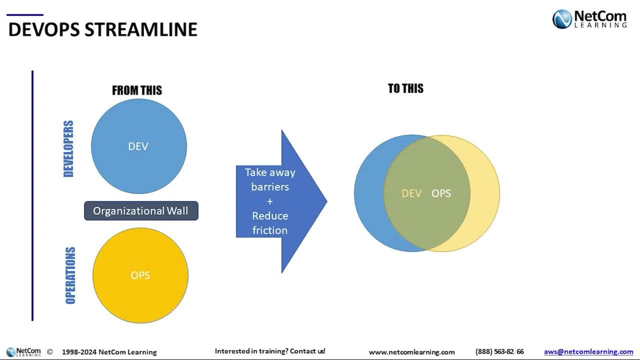 Right. So what we're seeking in DevOps- and you may not get there right away- is what you see on the right hand side, which is the development team and operation team Actually being one team. you know the two pizza team, Right, And then working on the same goal at the same time as a one team. 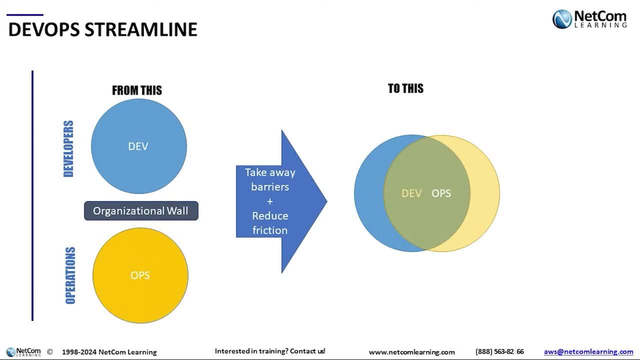 That's what we're looking for here. You have no barriers because, look, they're all in one team. Okay, All right. So that is the streaming streamlining, And let me get to the third point, which is pretty important here, which is automation. 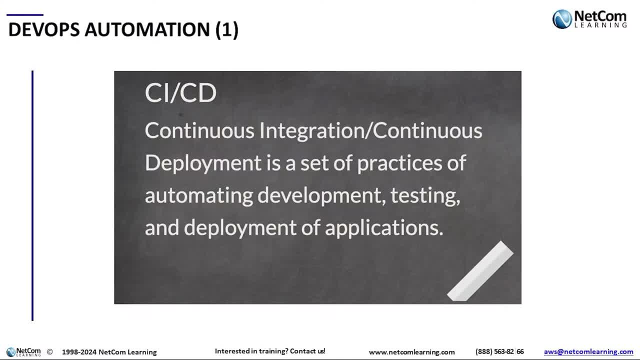 Okay, So automation, I think you know a lot of people know It's pretty natural Automation. Well, take normally a lot of human factor away from the whole process And not to say that you know we all need to kind of take away the- you know the person in the middle type of stuff. 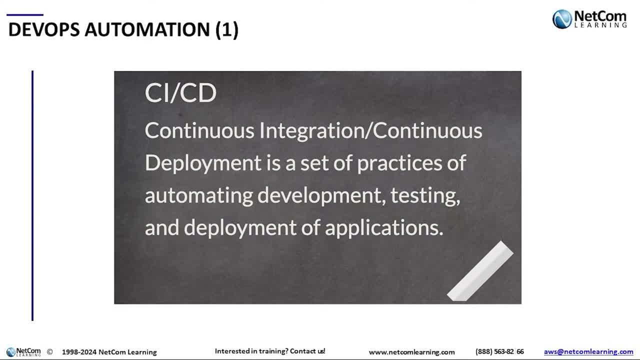 But you know, humans are really good at. people are very good at, you know, innovation Right Coming up with some brand new ideas. But you know, I'm not sure if we are that efficient if we're doing repetitive tasks. 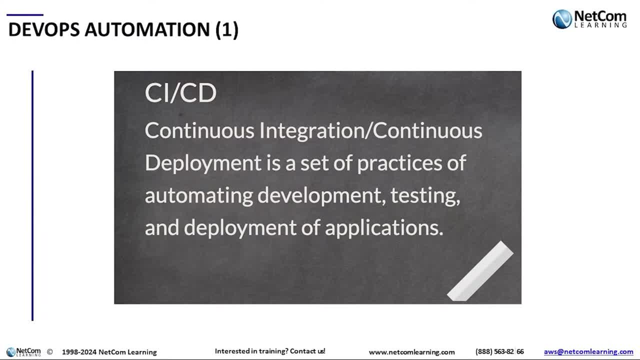 So if we're doing something is repetitive, Right, It probably doesn't really require a process, So let's go ahead and automate that, So we could take the negative part of having a person in the process, which is like making you know- I usually call it the fat fingering stuff. 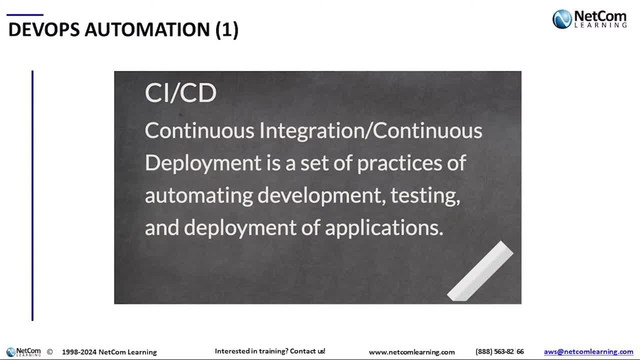 You know making mistakes, making, like you know, dumb mistakes and stuff. All those things will go away And you could run this iterative process Right In a very standard manner, in a very, very fast manner. Right, Streamlining, making it quick, increasing the velocity. 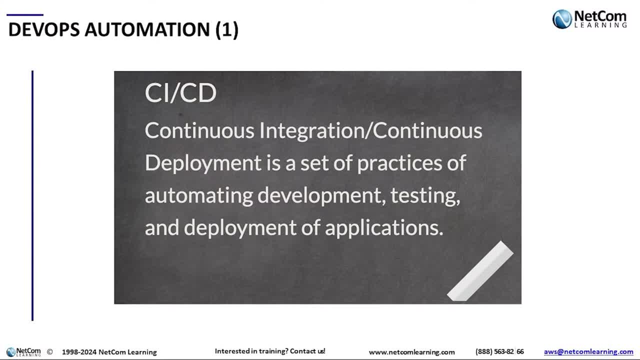 Everything kind of goes towards automation. Now in DevOps, the automation has a special function. It's called CI, CD. Remember I already mentioned that once continuous integration, continuous deployment- By the way, the D can also be delivery. So I actually have a next slide. 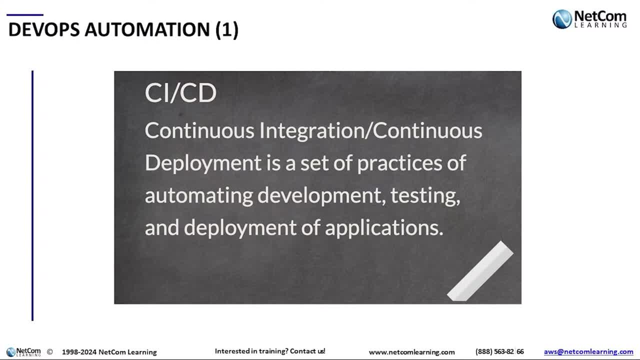 We'll talk about that. So it's a set of practice for automating development, testing and deployment of application. Oh my goodness, Look at that, That's SDLC, Right? So that means CI. CD is a way for you, for one, to automate the whole SDLC procedure. 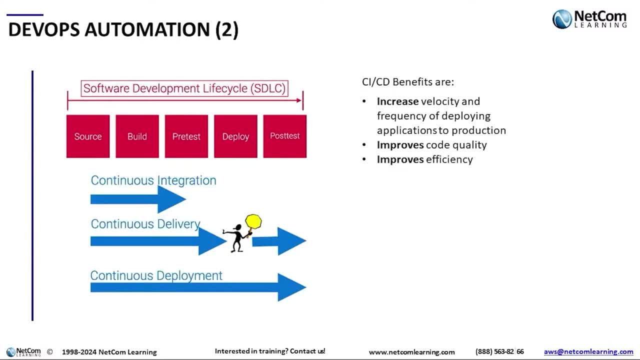 There you go, All right. So in taking a look at another way here, you have kind of laid the SDLC on the side this time, And now the software development lifecycle goes from left to right, And I've added a couple additional steps in the SDLC that you may see. 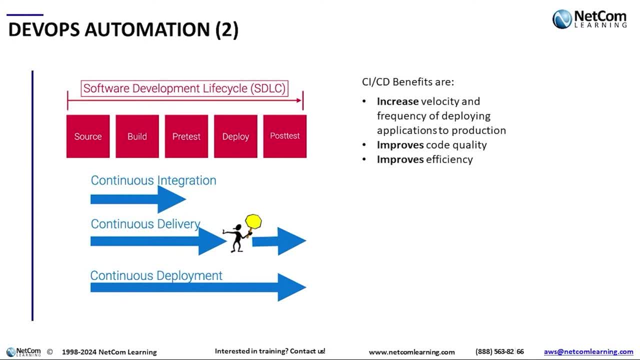 So maybe you know this is actually the difference between systems development lifecycle and software development lifecycle. I've actually switched it to software development lifecycle, Right? So here we have the CI, which is continued integration. So CI part is normally the traditional developers. you know what they will be doing. 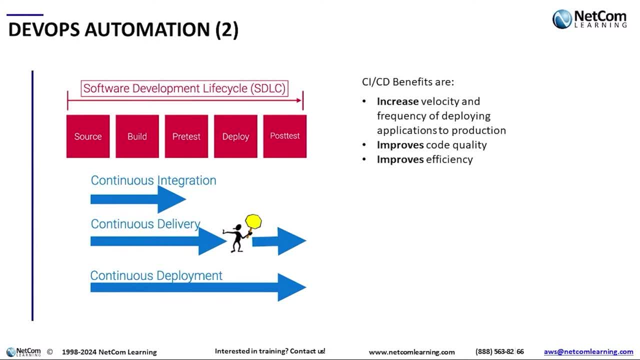 OK, so that means with the continuous integration, the developers are creating continuously new pieces of code that must be integrated with other parts of the code, So maybe there are other functions that must be integrated. That is, integrate means, you know, bring two things together or bring one. 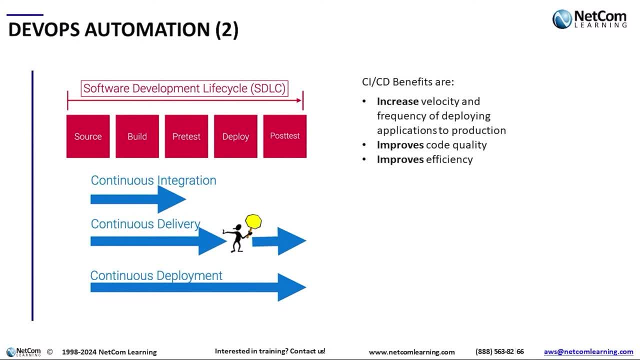 Things together or bring multiple things together Right As one piece. So the the functions. that's happening in the continuous integration is the developers will finalize their code and they will what's called commit to that code And once the code is committed, the developer saying: OK, I'm done with this part. 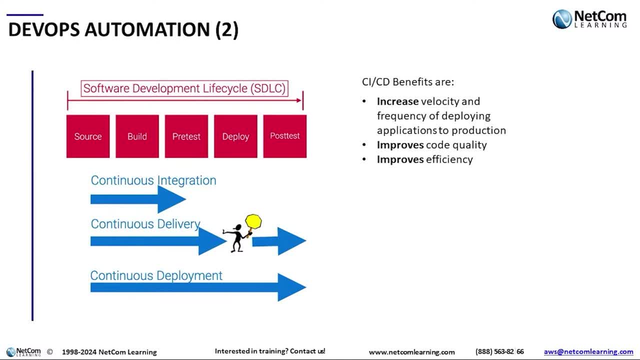 This can be tested And you know, if given approval, please deploy it right to production. So that's basically what the developer is saying in the CI phase, Right? So in the CI phase, the developers would do their testing and some of their testing would be something like: you know, unit testing is a very common one. 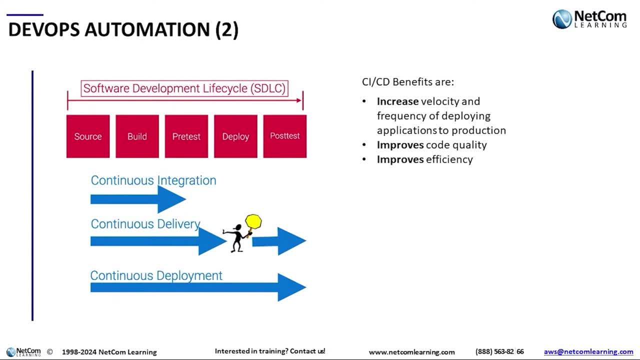 They may do integration testing, functional testing, Right. So in the development world there are different types of testing that the developers can do. So that's going to be done in the continuous integration part. But the you know that the continuous integration is over when there is a nice little patch. 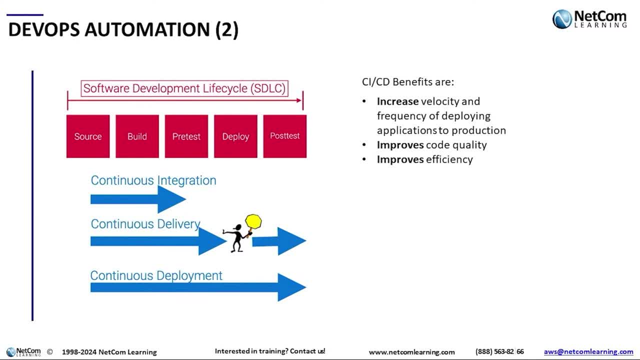 A package of software that's ready to be deployed. OK, so that's how you know that continuous integration is over. So at the CI phase you should have a what's called the artifact Right. So the artifact is a package. So if it's a Java program it will be a jar file or war file. 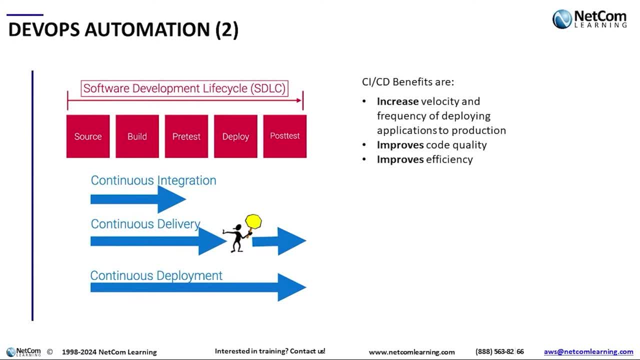 If it's a Python, maybe it's a zip file that's been packaged, But you know that's that's called the artifact, Right? So once we talk about CD, now I have two, So you have continuous delivery and then we have a continuous deployment. 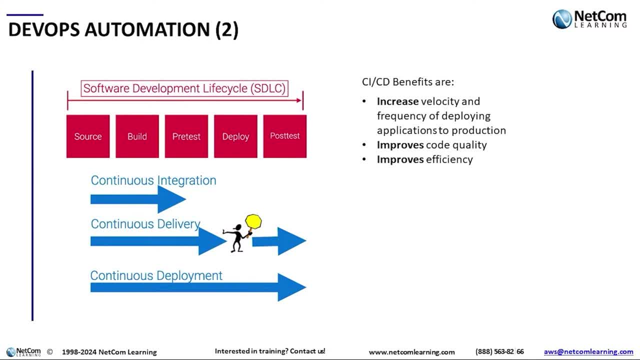 So let's take the continuous delivery. You choose one or the other. OK, so continuous delivery. Notice it actually takes you right from the source, which is where the continuous integration was all the way to the end, where you have a deployment and then testing to make sure that everything was deployed. 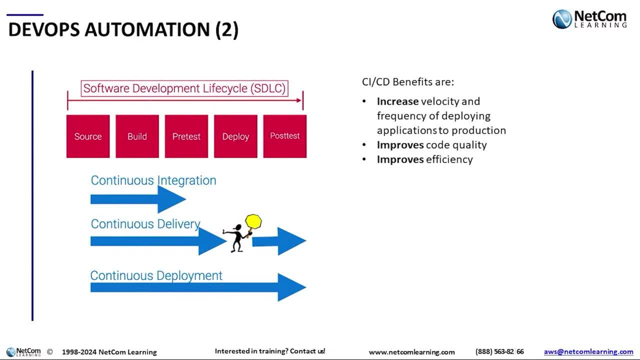 So here, ideally, we're talking about the production environment, But right in the middle, right where it says deployment, you have this little human. There is a stop, OK. so this is where you have a human in the loop, that almost everything's automated, except right at the end, before your product is ready to go into the production environment. 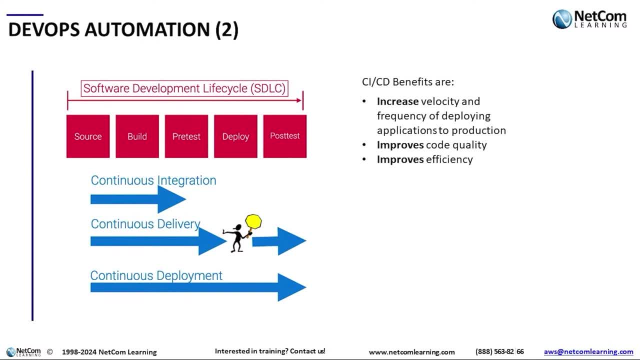 You have a person or a team of people that will look at it and say yay or nay, says OK, I think this is ready for production- or no? I don't think this is racial production. I think we need to tweak a little bit. 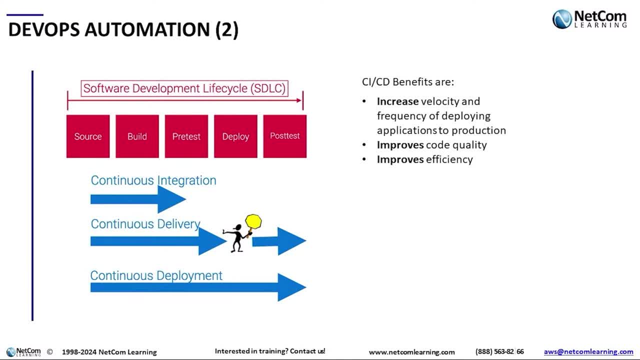 So this is where you still have a, Where you still have a person in the middle, And I hear that a lot of companies are in this model, which is continuous delivery, But for some companies this is still too slow. It's still. there's just a little bit more. 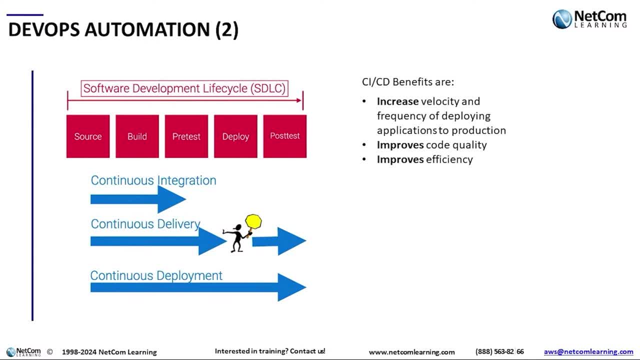 You know there's friction because there is a person in the middle. So they'll go for an up for something called continuous deployment. So continuous deployment is from the beginning, from the source stage, all the way to the production. Everything is automated. 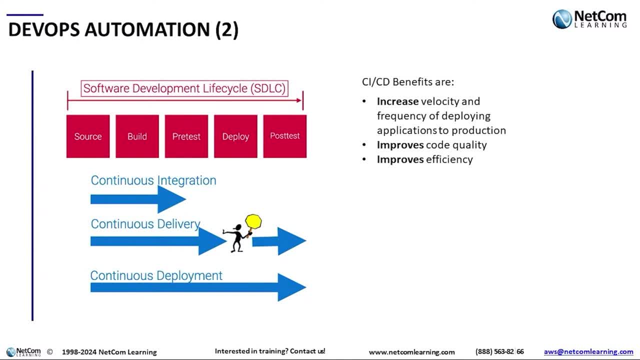 Like I said, I'm not sure If any company or you know, if a lot of companies are in this stage. I don't think so. I'm not. from the survey that's been taken by AWS, I believe about 80% of the customers that they've actually interviewed said they're doing this delivery rather than deployment. 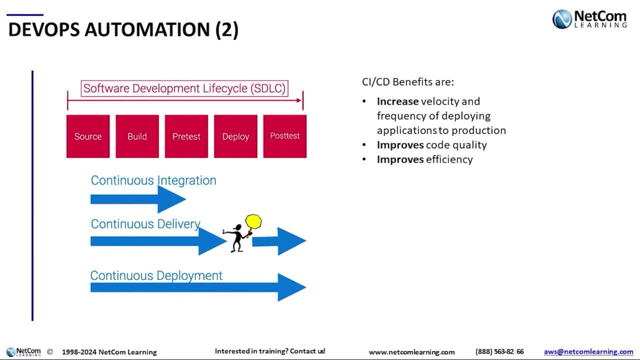 But if we're looking for maximizing- and you know, really, you know, stay in the theme of DevOps- then the eventual goal that we're looking here perhaps is continuous deployment, Okay, Anyway. so why is automation good? I think you probably intuitively know that. you know automation will make things faster. 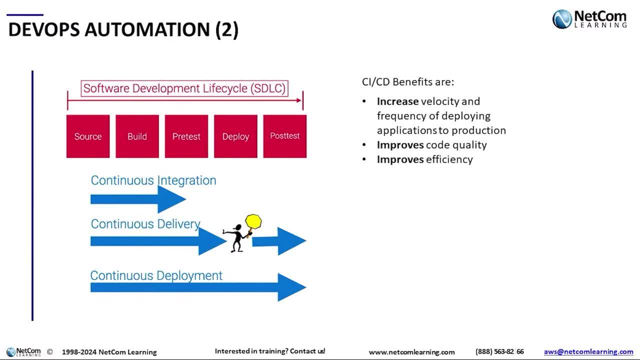 So definitely CI CD benefits are increased in velocity. Okay, And because we are, I remember we're working on smaller teams with smaller piece of code And remember, on the agile we do iterative processing. So here is actually frequency of deploying application to production. 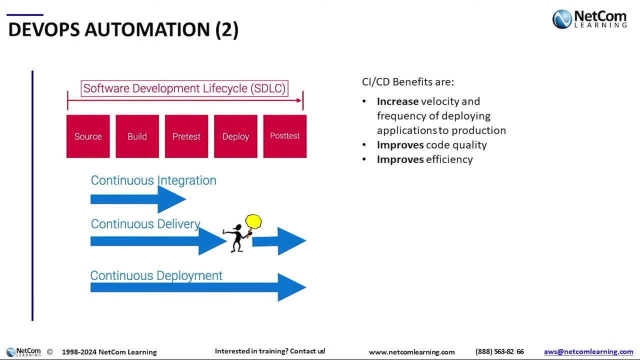 That means you can have, you know, a bunch of little Iterations and everything will be automated. So as soon as you're done with and commit the source code, boom right, The automation, the CI CD takes over. And if you're doing this deployment, everything's going to be automated, including testing. 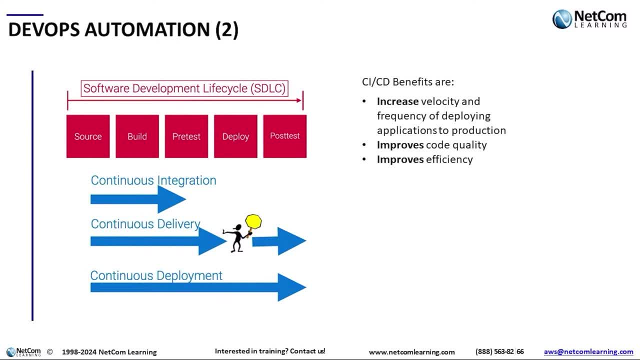 And then your product is going to be on. you know your end users are going to be using your product like right away, Maybe even multiple times a day, Okay, So I've heard some companies doing that multiple times a day too. Now it improves quality. 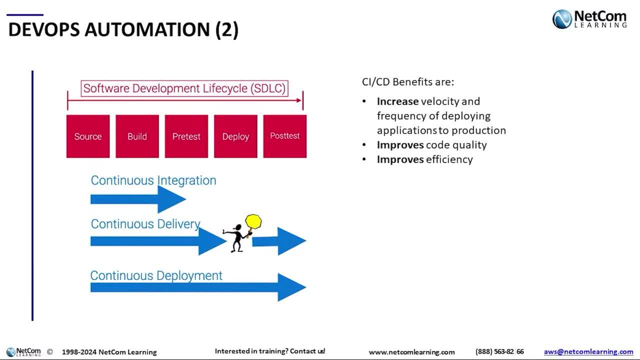 It improves code quality In general because you're doing iterative development, So that means you're making iterative changes, So that means you're you're working, you're making smaller changes And you're able to handle, let's say, let's say you, you know there's some kind of a mistake in the code. 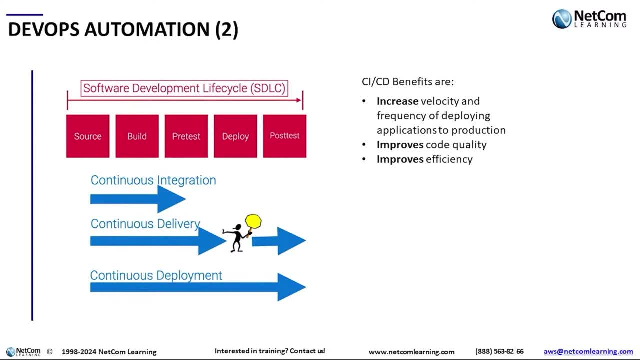 You should be able to handle that quickly and fix it. You know very quickly. Whereas if you have a humongous piece of code, which is usually called monolith, And it took you like months and months to create it, What if there's a mistake in there? 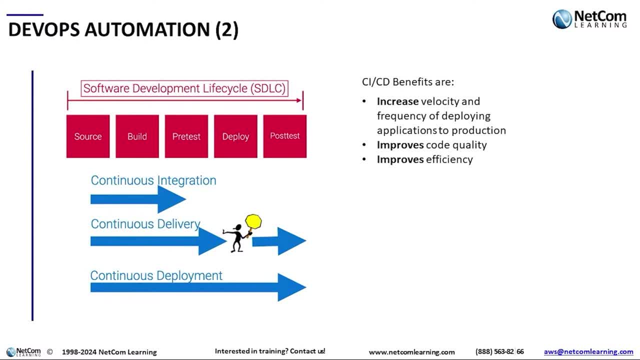 What are, like you know, bugs in there. How will you find the bugs You know in midst of, like, millions and millions of lines of code? It's hard, Okay. So if you have smaller piece, hopefully the code quality is going to be much better because they're smaller. 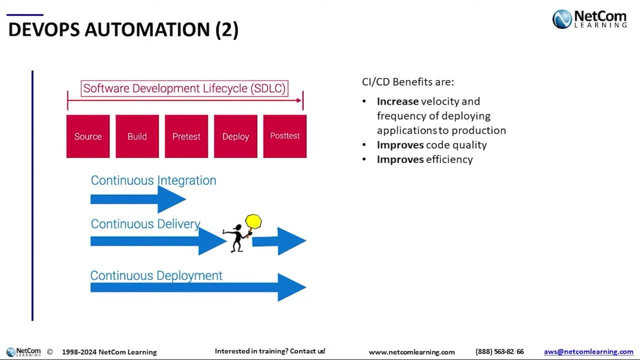 And you know you can get to the problems and find them easier. And then, last but not least, improves efficiency, Because it improves efficiency And now you are deploying incremental changes, Incremental improvements to your code. Okay, And you actually don't have to wait, right? 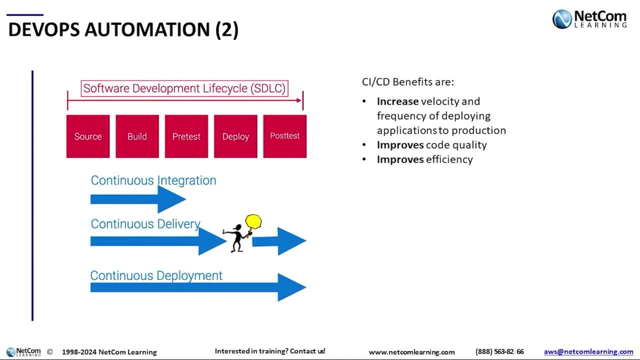 For all the people, dozens of people- to approve whether it's okay for you to deploy this code. You know, smaller piece, smaller team, They're totally responsible, normally, So that they can go ahead and improve it And then update it whenever they feel it's necessary. 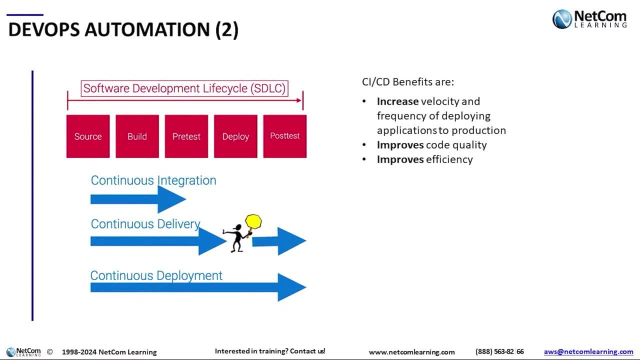 That usually goes hand in hand with DevOps, Okay. So there you go. So that is the DevOps automation, Okay, And now I want to kind of introduce you, now that I've kind of went over three of the core characteristics of what a DevOps is. 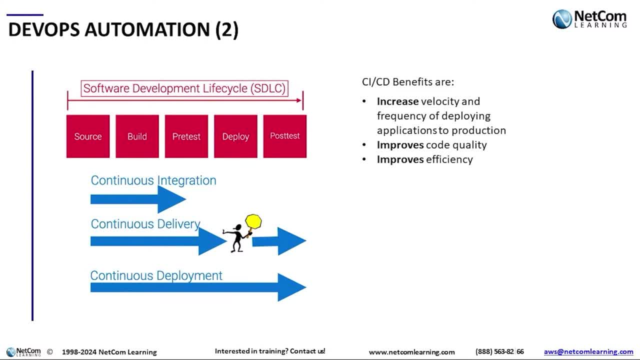 Remember the culture part of it, right Streamlining part of it And the automation part of it. There are three other supporting technologies procedures that I would like to introduce to you that actually supports the DevOps process. Now, these are not necessary for DevOps. 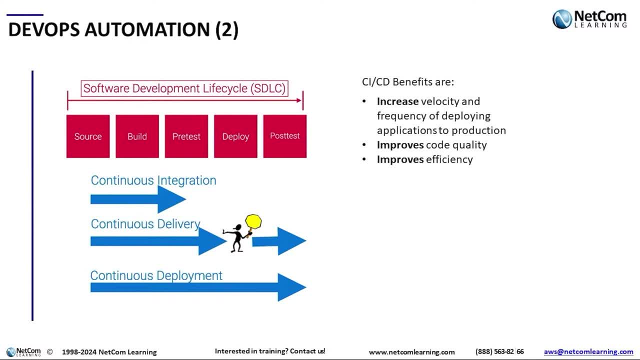 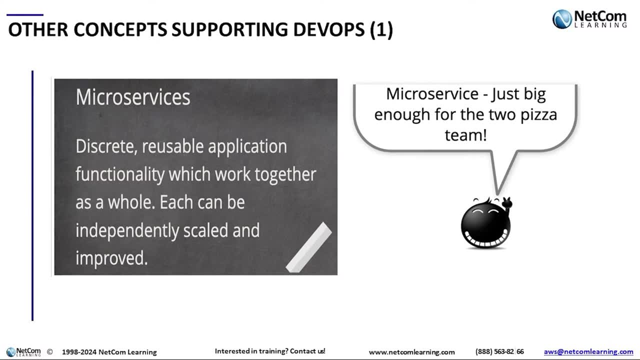 But they are very, very helpful. So let me talk about the first thing here. First one is called microservices. Okay, So from the name of it it says, okay, micro, very small right Services. Yeah So services. here we're referring to your application that you're deploying, right? 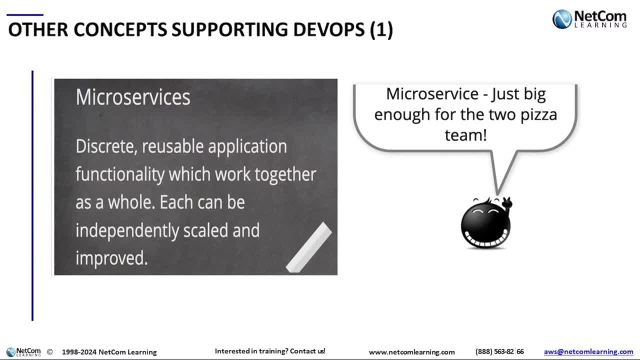 So here it is, the definition: Discrete, reusable application functionality which work together as a whole. Okay, Each can be independently scaled and improved. Right? So from this, What I want you to get here is that a lot of the companies currently are developing what are called microservices. 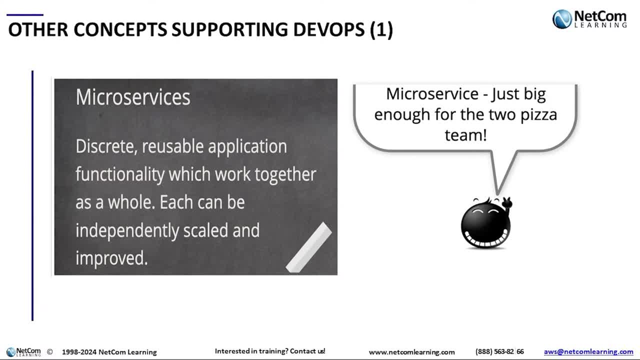 Because they are a small piece of code that is just big enough for guess what? Right? Two pizza teams, Right. So two pizza teams and microservices go well together, Okay, And these two pizza teams can be independently responsible for their microservices. 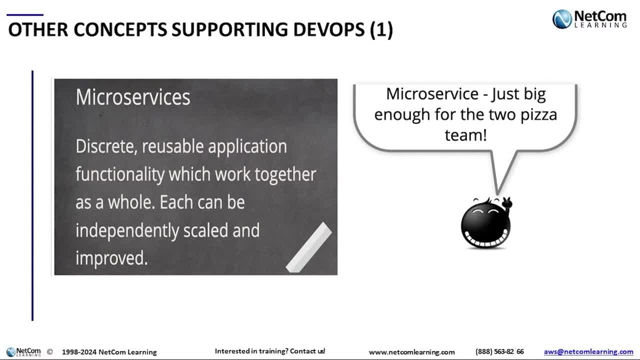 That's why they can go ahead and decide when they want to, you know, commit the code and then to deploy it in production. But because they are smaller pieces of bigger, let's say you know business function that these microservices will probably have to work with each other. 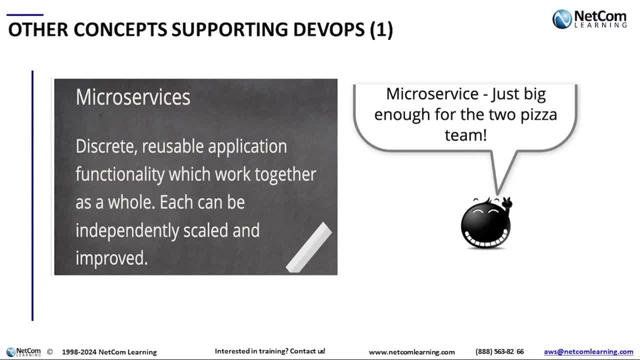 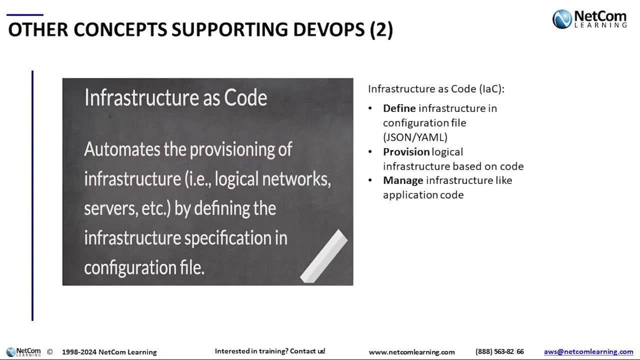 Right, So anyway, so that's called the microservices. Microservices has been around for a while now, Right? So if you're familiar with something called web services, microservices and web services are akin to each other, Right? So the next supporting concept here is something called infrastructure as code. 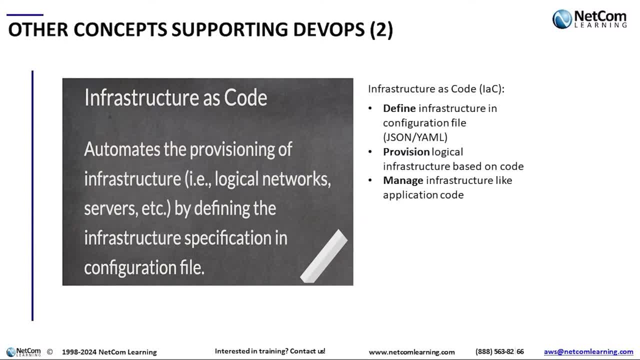 So you know that application is code, Right? So when we create application, we create something usually called source code, Right? So the source code needs to be compiled, Right, We call that building process, Okay. And then, once you compile it, you have something like you know, something that's called a source code. 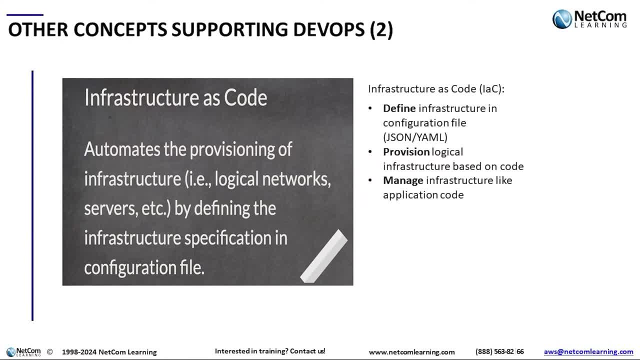 Right, Something, something that EXC file, Something, something that DLL file, Right? So those are the programs that you actually run. Okay, So I think it's pretty clear: Right, Application right is code Right. But what does it mean to have the infrastructure as code? 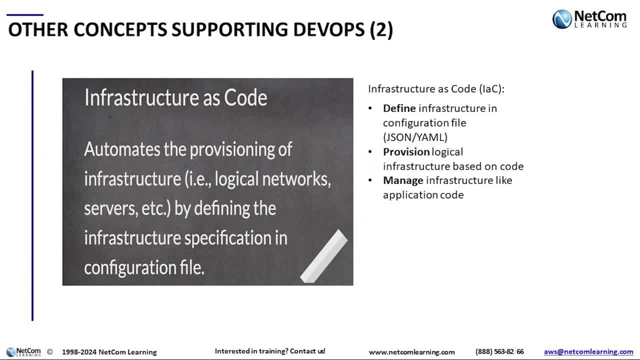 Right, Because infrastructure, you know, for me, I've been working, like many years, on networking. you know, setting up servers Right, Setting up Windows servers, Setting up Linux servers, That's infrastructure, isn't it? Put in security devices, like you know. put in firewalls and intrusion detection systems. 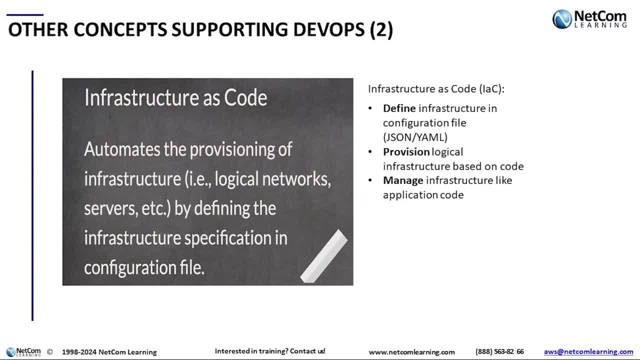 Those, those are. they used to be like boxes that I have to, like you know, plug right into the network. That's infrastructure. So what are you talking about? Infrastructure is code, What? Okay, Well, these days, you know, starting from, like you know, a lot of years ago still, maybe, like you know, 10,, 10,, I would say, let's see, probably close to like not quite 20 years, I don't think, where virtualization became very popular. 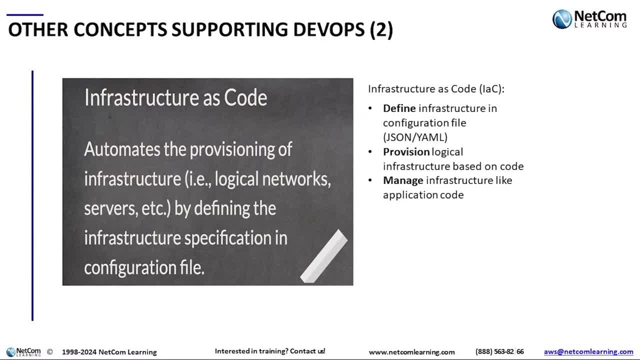 Right, And companies in their own data centers start to use virtualization, like you know, VMware and stuff- to say, yeah, I have servers here, but these are virtual servers. Okay, All right then. So if a server- a physical server- becomes a virtual server, the virtual server means that you know it's not a real physical server. 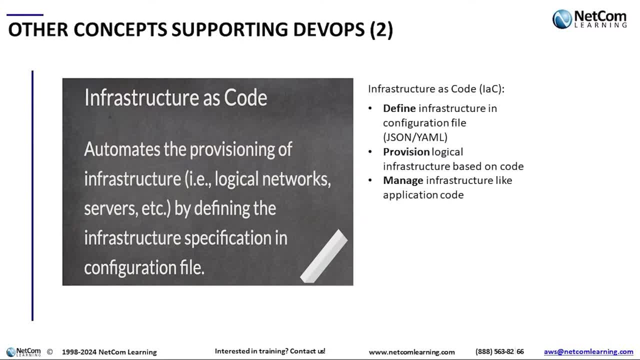 It's actually an application, Right? So it's an application that's kind of acting like a server. So if it's an application, guess what It's code? Okay, So infrastructure's code refers to the virtualness of a lot of things that we do these days. 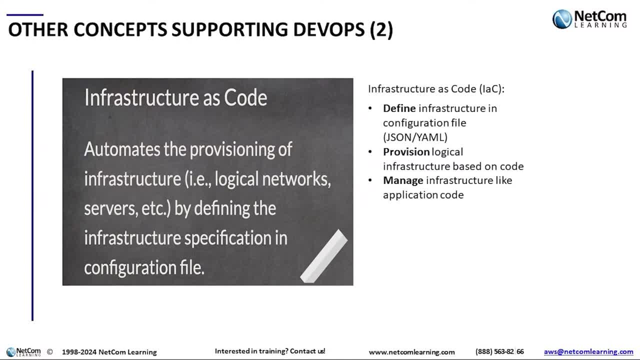 Right, So it's a virtual. you know it's a virtual network. Another way to say it is logical, Right. Logical network, logical servers, logical security devices: Right, There's no physical boxes to kind of, you know, throw around. 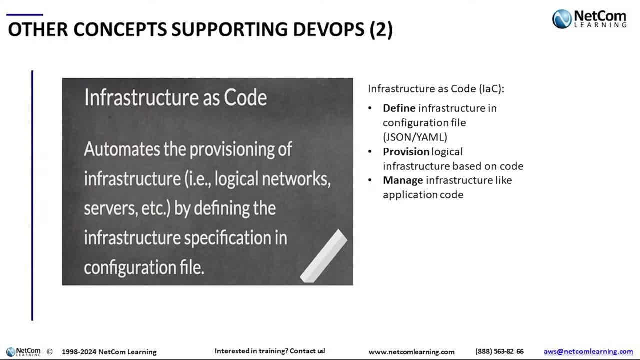 Okay, So that's that is. this is a supporting technology that is very, very helpful in speeding up the process, Because you can handle Infrastructure Right Like another piece of program, Anyway. So once you have infrastructure as code, you're defining the infrastructure components. 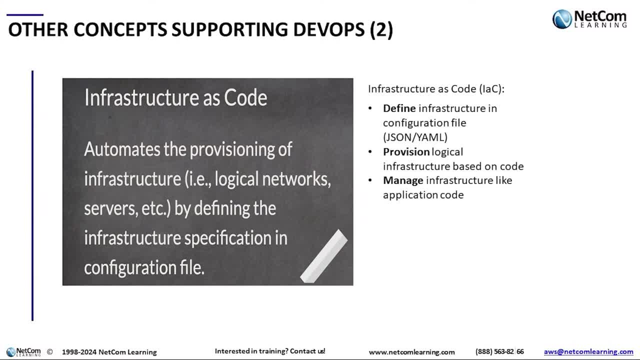 These are called resources inside a piece of text file, Right, They're usually in a JSON format, YAML format, Right, Just specialized for notational format. Then you could say: hey, please, can you kind of launch a server for me. 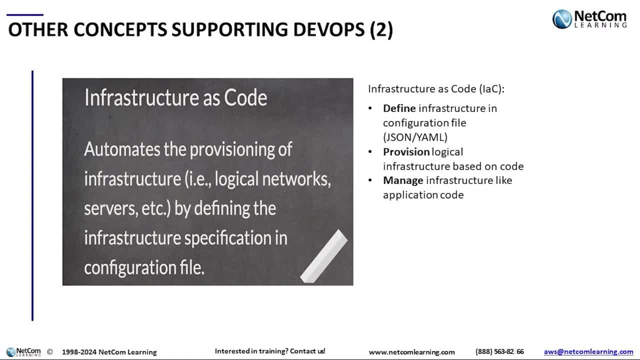 Can you launch a network for me So you can provision logical infrastructure based on piece of code, Right, Which is that you know the JSON file or YAML file that we're talking about And guess what? You can manage these infrastructure like another application code. 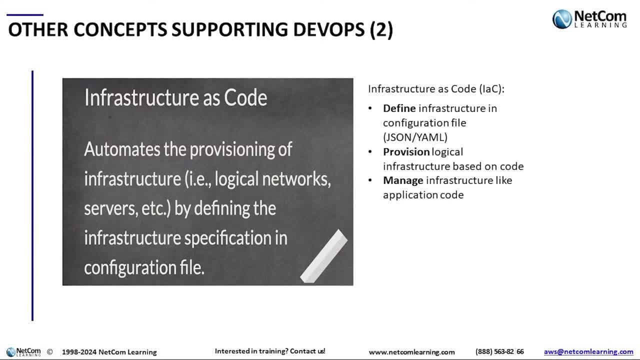 Yeah, Put it in a version management. Get a version 1.1 of the infrastructure. Get version 1.1 of the infrastructure. Get version 2.0 of the infrastructure. There you go Right. So that's the second supporting technology. 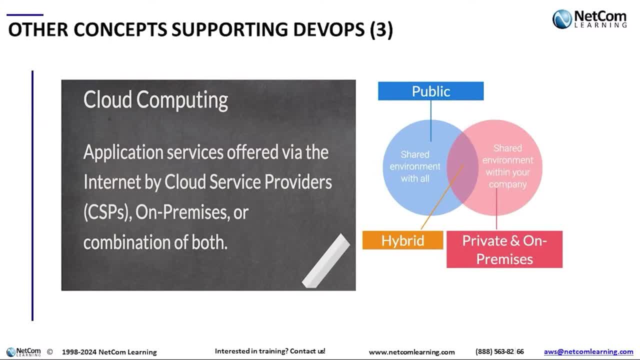 And last but not least, The cloud Right, The cloud computing, Now cloud computing. So this is you know. today, of course, we're going to be talking about AWS, But you know, cloud computing in general is application services offered via the internet. 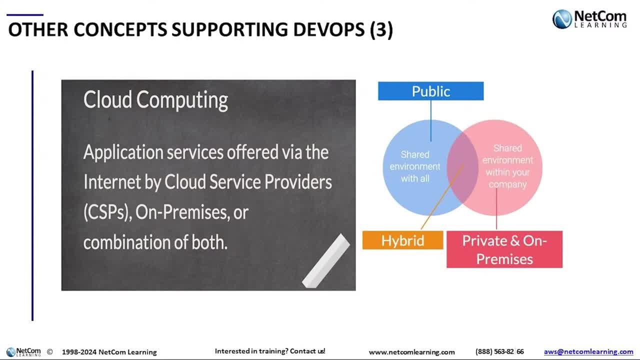 by cloud service providers, Right. Or you can have them on premises, that is, in your own data center, if you have something called the private cloud, Okay. Or you could combine them both, And that's usually called a hybrid cloud, Okay, So anyway. 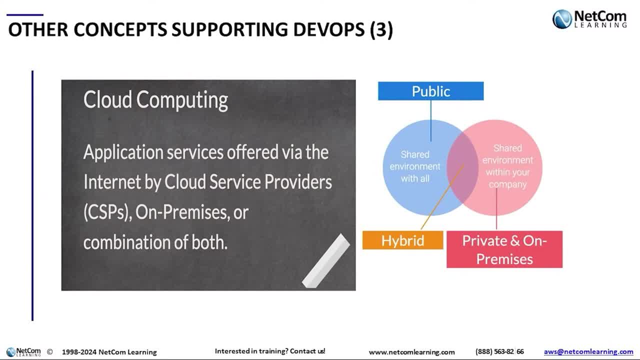 So cloud computing actually makes it really easy for cloud computing. It makes it really easy for companies to virtualize everything, Right, Right. So instead of saying, oh, you know, I have these, you know, I have like 10 servers and 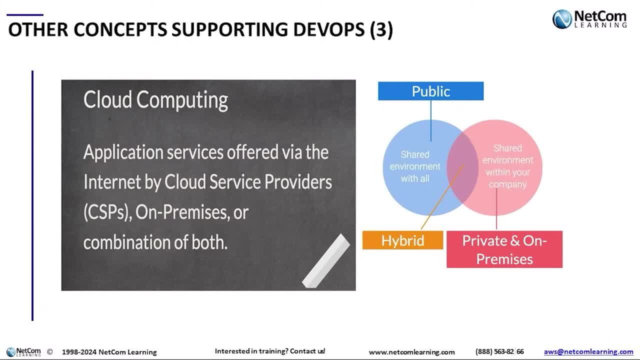 I have a network. It says, okay, we can recreate the same thing, Let's say, on AWS, But they're all going to be logical networks and logical servers, Right. So it's easy to make that transition from the physical to the virtual. 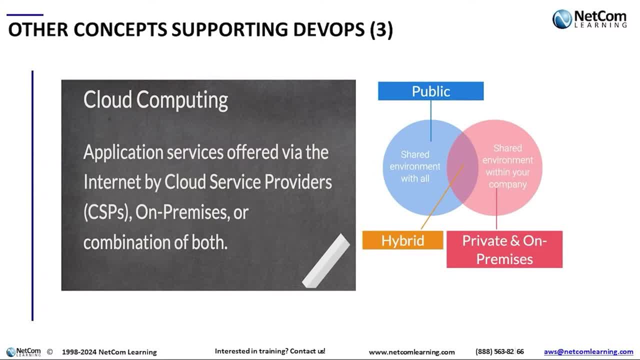 Okay, Using cloud computing, And obviously there are tons and tons of other benefits of moving into cloud computing. But there you go. So those are the three support technologies concepts that actually assist in DevOps. Okay, So here I want to kind of switch gears. 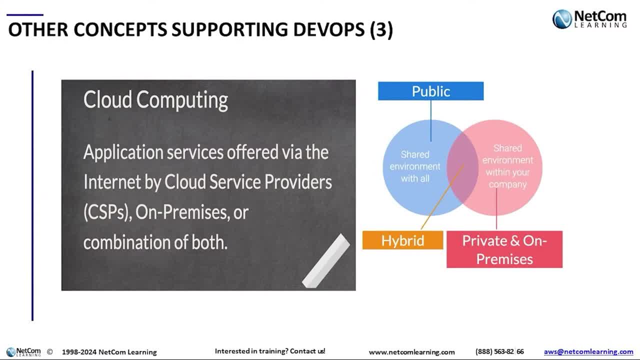 Okay, From here Now I would like to go in and start introducing you to how do we do all this stuff. I mean, sounds like DevOps, sounds like a great idea, But how do we do this in AWS And what are some of the services that are offered in AWS that's going to actually help? 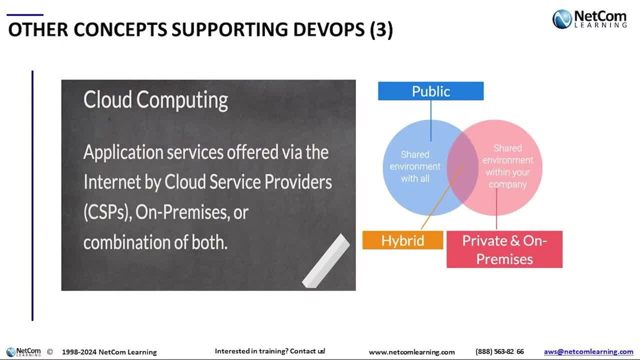 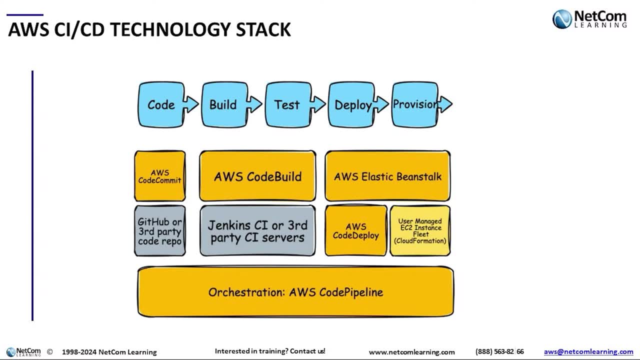 me do this, All righty. So let's go and take a look. So here I have titled AWS CI CD technology stack. Okay, So right on the top in blue you see the SDLC. Okay, So you see the code, the build, the test, deploy provision. 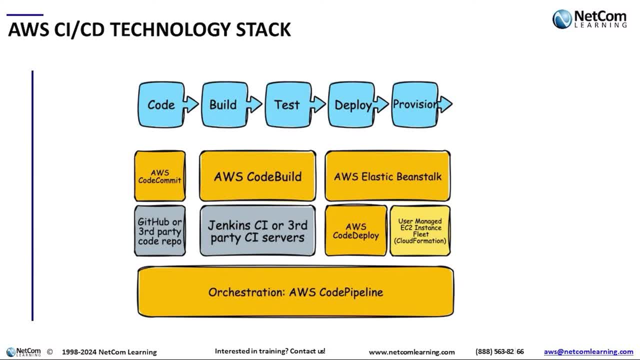 Okay, Once again, a little bit different. Okay, I've added a couple of things where it says deploy and provision. Okay, But and what underneath are some of the services, not all, Okay, Some of the services that you would map to AWS services. 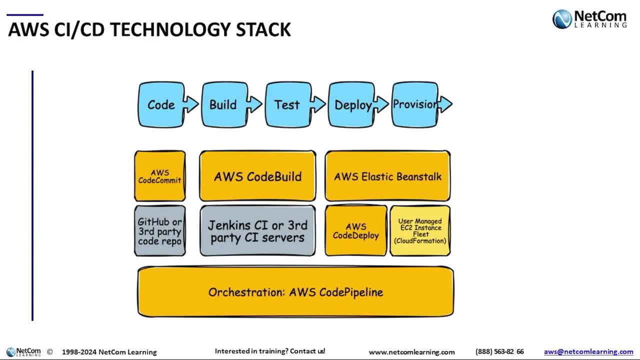 So let's go and take a look from left to right. Okay, So under code that would be called management, Okay, Or sometimes we call it, you know, version control, Okay, Where you're updating the code and making sure that everybody understands what version. 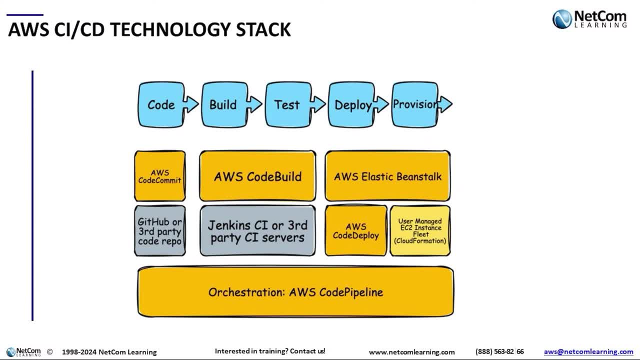 it is. Is it version one? Is it version 1.1? Is it version 1.1.2? You know? So for that, I'm going to go ahead and show you the code. Okay, So for that, a lot of companies will use something called GitHub. 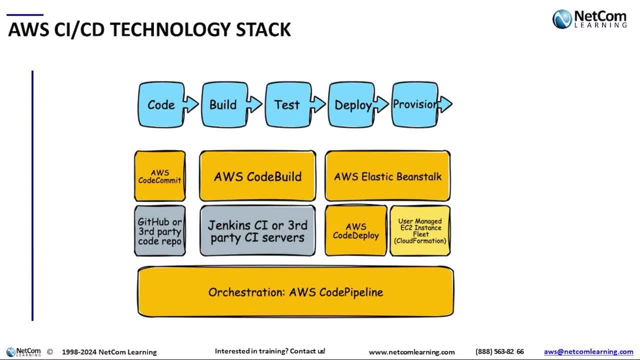 Okay. Well, the GitHub is a third party version management system and software, So something like it is provided in AWS. It's called a code commit. Okay, So code commit, So they kind of fit into the same genre. Okay As GitHub. 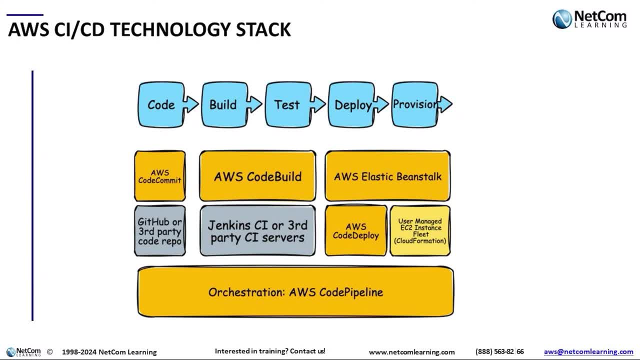 Now during the build and test phase, there are some very popular third party services and software. One of them that comes to mind is Jenkins, So if you're familiar with Jenkins, it's an open source, what's called a CI or continuous. 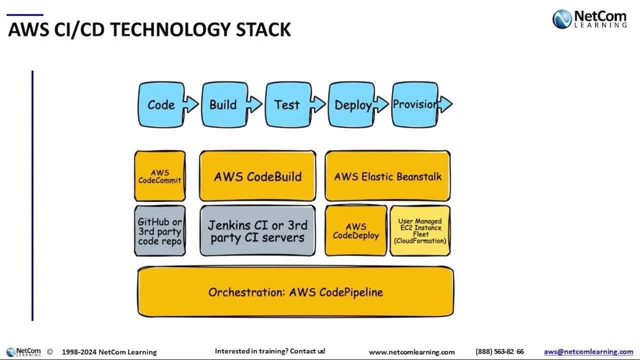 integration server that will help you in doing and automating the build phase. So the build phase usually, like you know, some doing some testing, compiling, creating packages, Okay, And at the end of the build you should actually get an artifact. 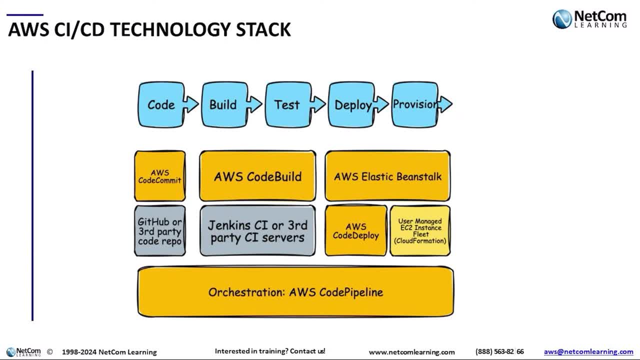 Remember the artifact: Ready to go, you know, in production, Right? So that piece of like an executable file? Well, AWS actually has this product or service, let's say, called AWS Code Build, Right. So Code Build will help you build. 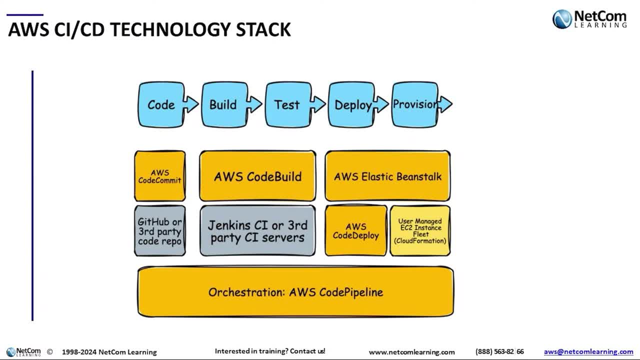 Okay, And also to help you test as well. So that's that piece Moving on deploying. So that's pretty important piece, right That you know. now you have the artifact, the artifact needs to be deployed. So, let's say, a server. 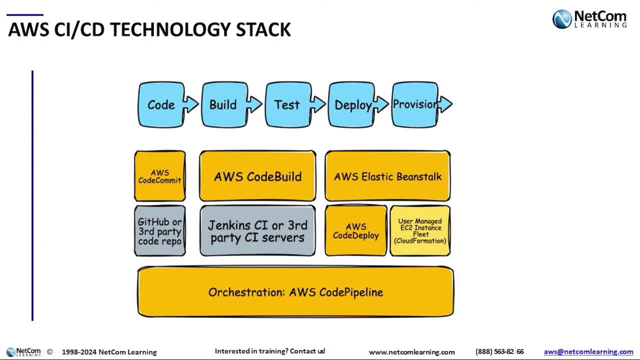 If you have, you know, Kubernetes or continuous integration Containers into containers, Or if you are using something called serverless- in AWS they're called lambdas. No, you're deploying to any type of an infrastructure or the platform where your end user are you. 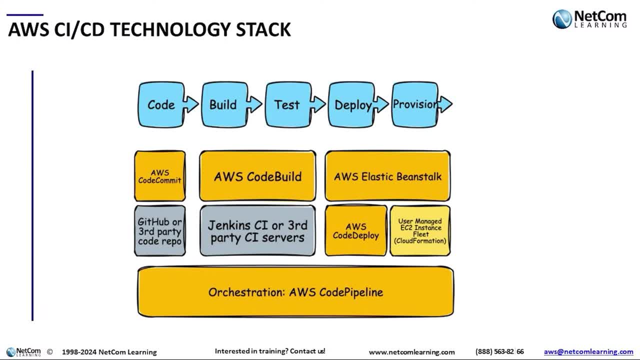 know users are going to be using it. Okay, So there is something called AWS Elastic Beanstalk. Now, Elastic Beanstalk is a service that assists you in deploying a web based application, Right? So let's say you have a three tiered traditional web based application with the front end, the middle tier and the back end. 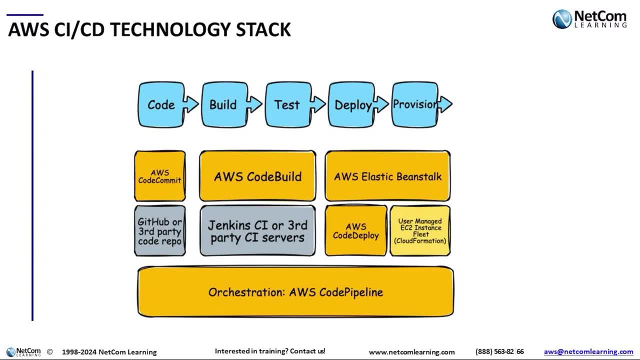 Elastic Beanstalk will make it really simple for you to deploy them, based on the AWS best practices. That has monitoring, It has logging, It has, you know, load balancing. It has all that features come in. So if that's what you want to do, Elastic Beanstalk will help you to deploy that. 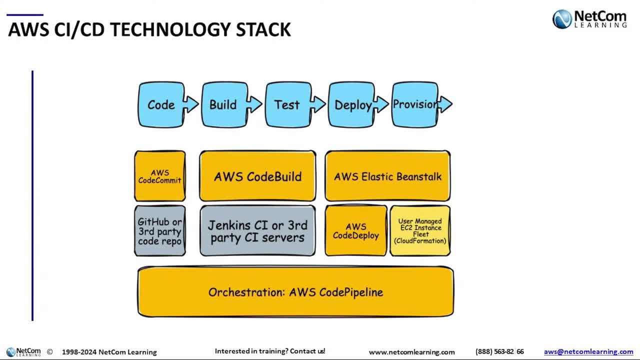 But if you want to be a little bit more free about the type of the design And the platform that you want to deploy into, there is something called the code deploy, As you see right under the Elastic Beanstalk. So code deploy is going to assist you in deploying that into production. 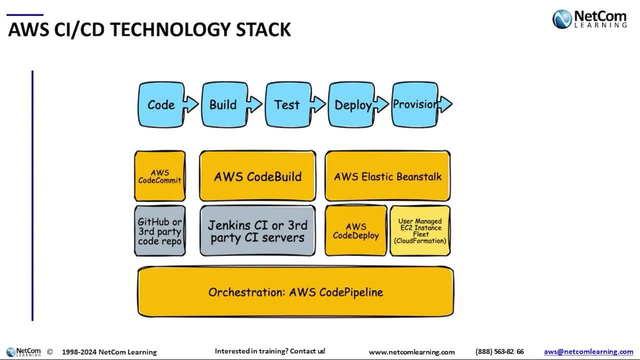 Now there are different platforms that you can have, So I have in there, you know, user managed EC2 instance fleet, So I have in there cloud formation. So there are many ways that you can deploy, So it gives you many options. 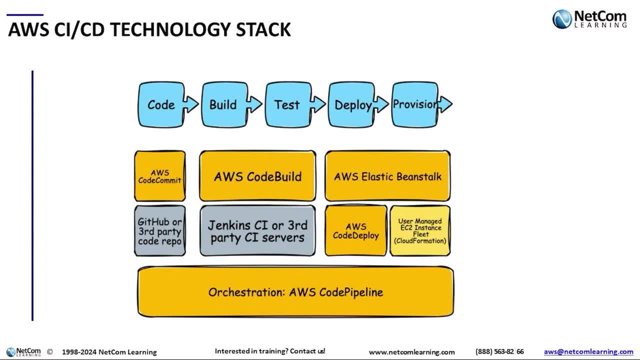 The one that you're going to be seeing is code deploy, But you know there are other ways. There are other ways of doing it today. Then remember, automation is so important in DevOps And all the tools like, you know code commit, code build, you know code deploy. 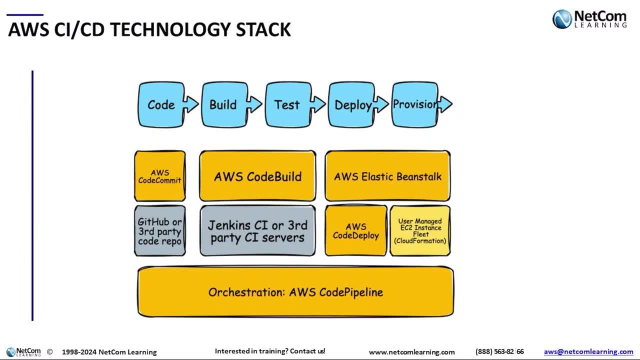 They're all individual services that will do their job all on its own, But the power of the DevOps comes in when you combine them all right To organize and orchestrate them all into one smooth process where artifacts- you know, your code- is moving from one to the other and to the other all the way to the end where it goes to production. 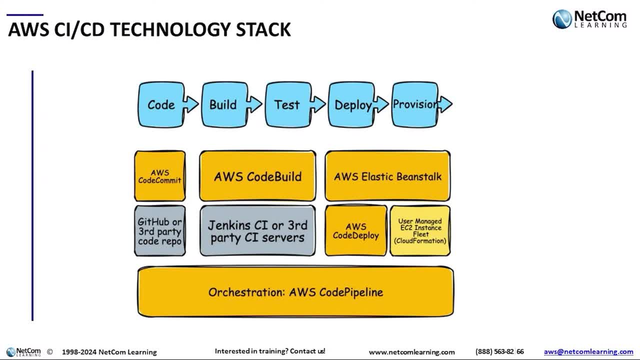 And that orchestration piece of service is called the code pipeline. So you see, underneath it all it kind of covers the entirety of the SDLC. So there you go. So these are the services. Now, if you are more interested in individually, you know what these services are. I'm going to kind of quickly go over. 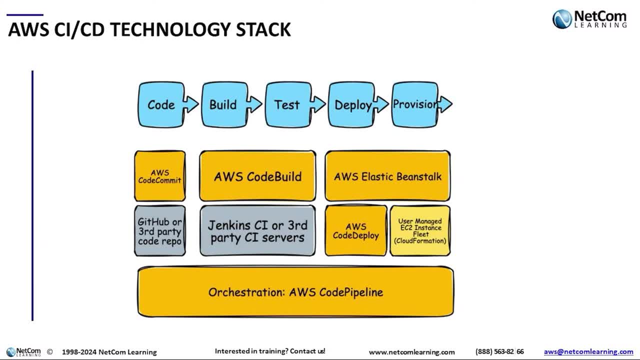 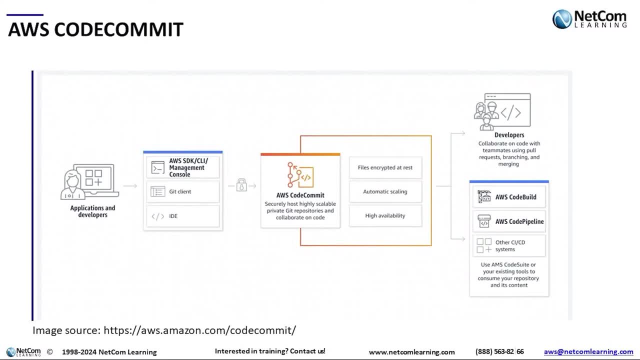 And show you what an AWS page looks like for each of those services. So first let's talk about code commit. Okay, So there it is. As you see, on the left, you see the application and developers And notice that they are using some kind of a client. 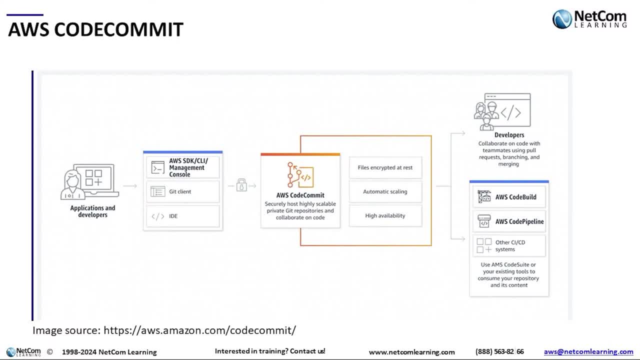 So in this case you could use something like a Git client or IDE integrated development environment. Then that code is committed to AWS code commit- Okay, And there files are encrypted- Okay, You know it will scale, That is, you'll have enough power to do whatever you need to do. 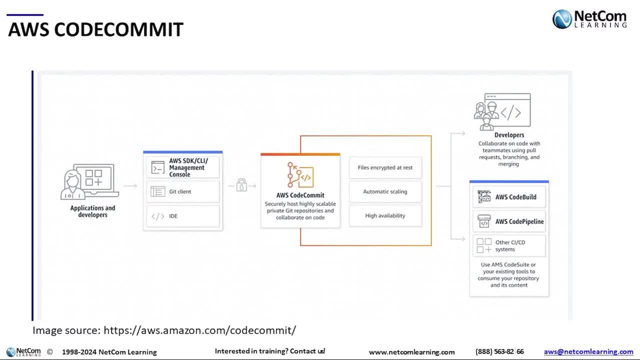 AWS. this is fully managed service by AWS, So you don't have to set up any servers, Right? And that's basically called code commit. Okay, And notice on the right-hand side, this is almost like a gateway right into the rest of the services. 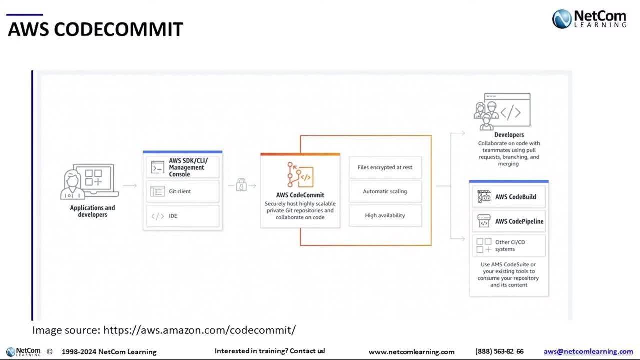 As you see, there you have code build, code, pipeline, other CI CD systems. Right, This is actually like a doorway into this whole the automation. let's call it pipeline, Okay, That we're going to be talking about, which is DevOps. 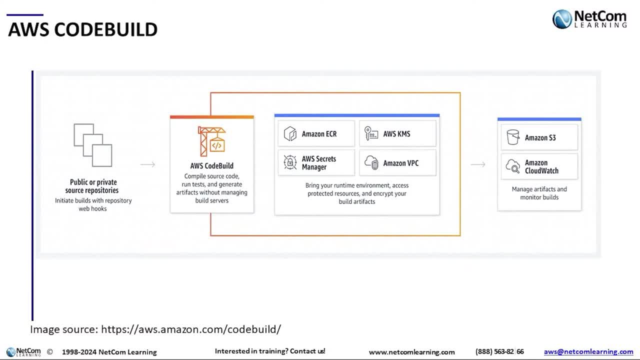 Next one here is code build. So code build. once again, you have code build which is going to be building, okay, your code Right, Building your artifact, And it says: you know, bring your runtime environment. So it's very flexible. 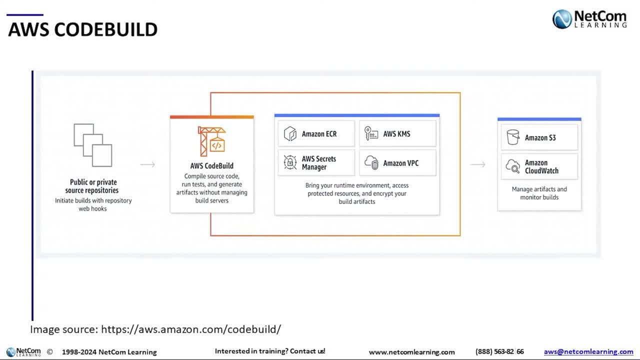 Basically, what this code build does is that. let's take, for example, something like Java Right. So you give source code to code build And you tell code build how to make it into an executable Right. That is, in case of Java. it's going to be called something called a bytecode, like a jar file, the war file. 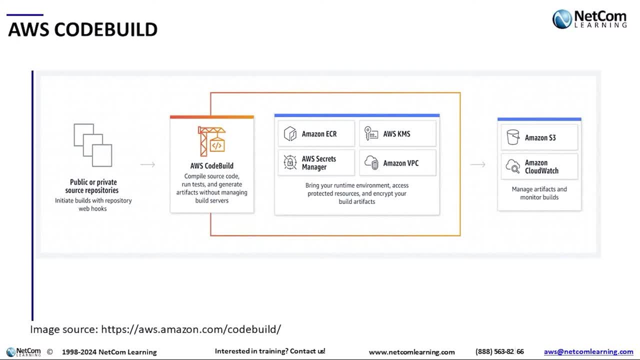 Right. So that's what you're talking about. You tell code build what commands they have to use- right, to create the jar file, for example. Right, What tools do they have to use And what code build will do is it will actually launch a container, Docker container- and then take your software, the source code. then it will do all that stuff that you tell it to do. 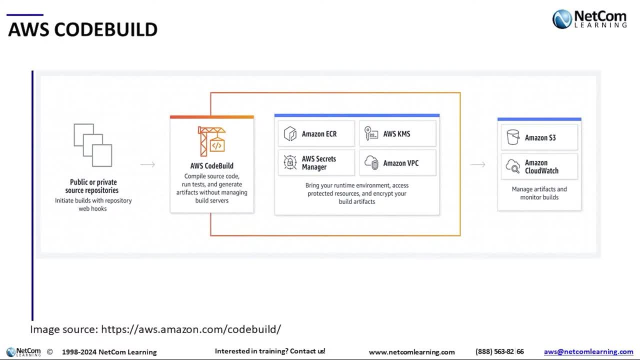 It will do linking, compiling. you know it will create a package, Right, That's basically what a code build will do At the end. now you have an artifact, remember, And you take the artifact and you store it someplace. 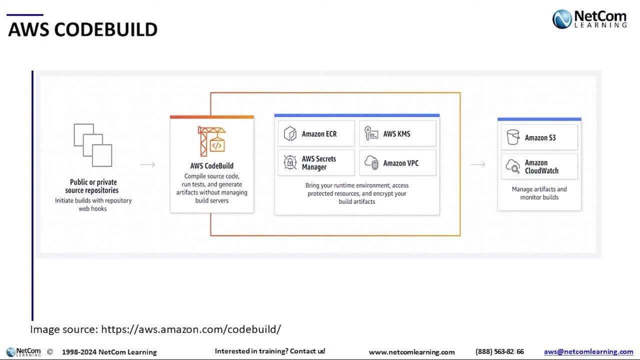 A very common place to store it in AWS is Amazon Linux. Right, AWS is Amazon S3.. Okay, So that's why you see way, on the right-hand side, you have Amazon S3 integrating with code build. All right, So the next service is code deploy. 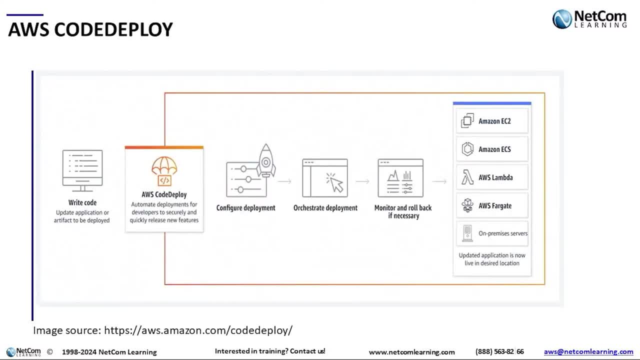 Once again, code deploy is just as the name said: it's going to deploy into staging area. It's going to deploy into testing area. It's going to deploy your application into production, Right. So that's its main job, Right. 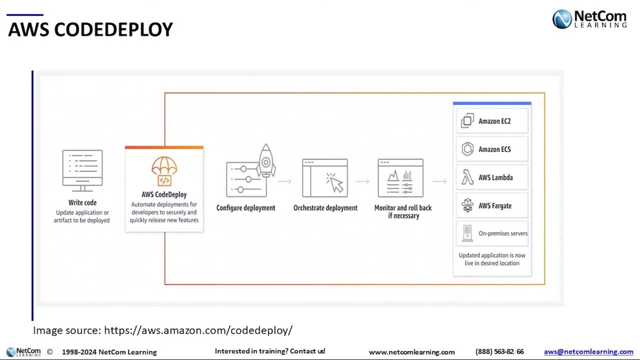 So, as you see, on the right-hand side, you see EC2.. So that's a virtual machine. ECS, So that is Elastic Container Service. So that would be, you know, your Docker containers. Lambda would be serverless, Okay. 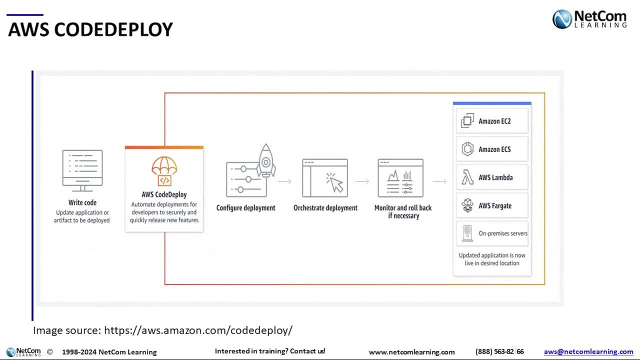 And other platform that you can take your artifact and deploy into, And code deploy will make it very simple for you to do that. It has options such as in-place deployment where you are updating your code. You know, maybe you have a. you know you already have 1.0 of your application running. 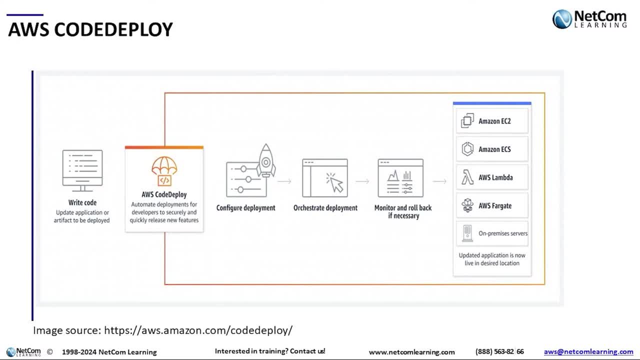 And you want to make change that over to 2.0. Code deploy will make it, you know, relatively safe for you Right To actually deploy the new version on top of, let's say, the old version, Or, if you feel that that's risky. 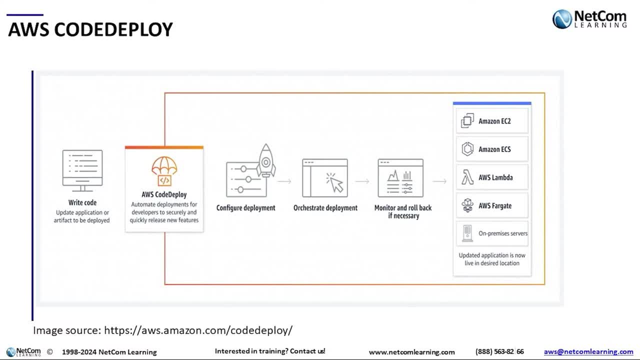 Right, Because you are changing the version, You're kind of overwriting it. You may say: ah, you know, I think. rather than doing that, I'd like to do something called blue-green deployment, Where you have two environments, The old and the new. 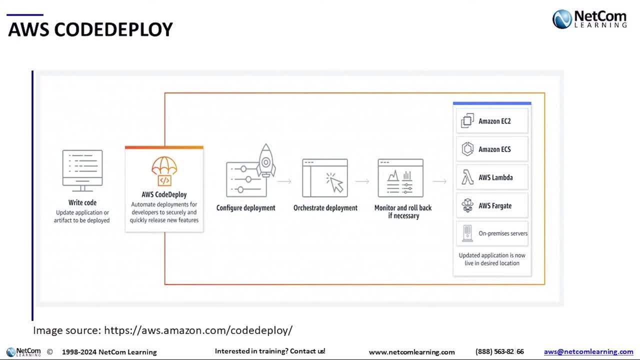 And then at some point you switch from one to the other. So that's much safer And you can actually tell code deploy to do that for you. Okay, So there you go. So that would be code deploy. Now there's one more service that we're going to be using. 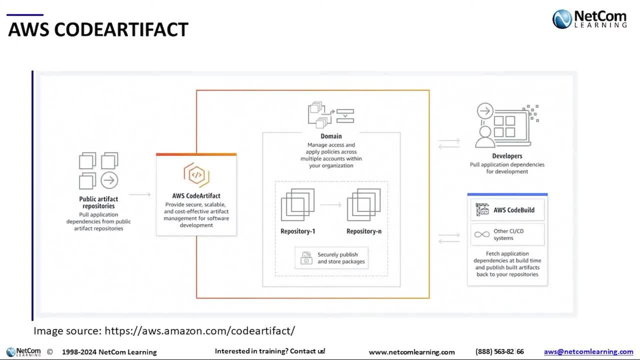 Something called code artifact. Now, code artifact is a service that you'll see in the demonstration as well- That actually allows you right, provides secure way to manage artifacts- Okay, But I'm not talking about the artifacts that you create. So these are the artifacts, or let's just say other people's programs that you need, let's say, for building stuff. 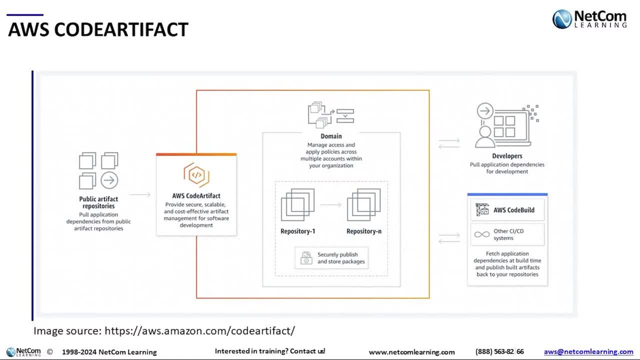 Okay, Now in our example, we have to compile a Java application, So we need a tool called Maven. Now, Maven is an open source tool, But what if you? what if that open source tool is not available when you need it? 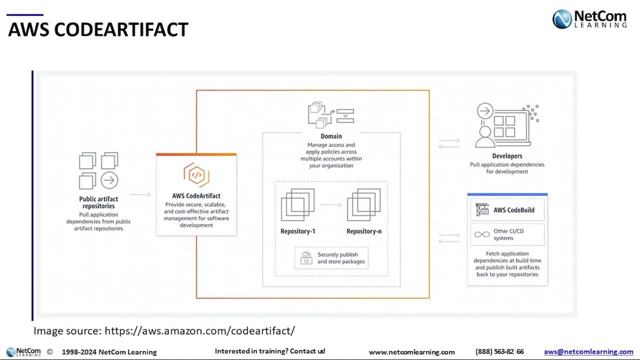 Right, Maybe there's an internet problem, You never know- Right? So if you want to maintain stability of your pipeline, okay, maybe you want to actually have those tools elsewhere, Like maybe somewhere inside AWS, Right, So that you don't have to mess with any kind of irregularities that you may have in the internet connecting to that external service, that you need to download a tool to actually do your building of your application. 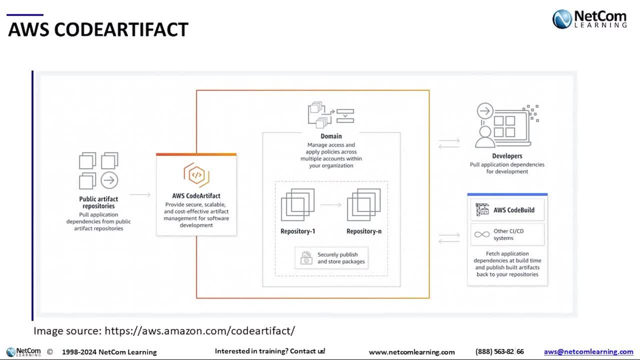 So we're going to be using it. It is called artifact in that way. That is, we're going to kind of, you know, put those external applications inside AWS so that you are you have a more stability in accessing those tools. 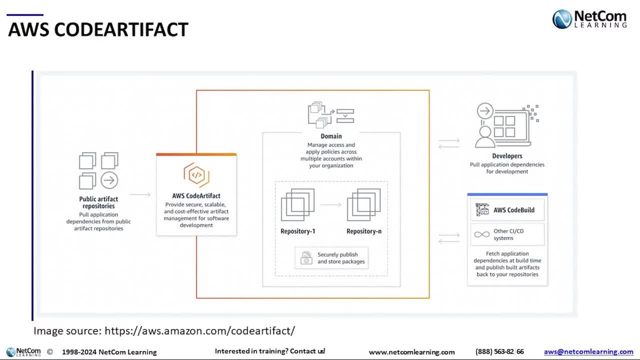 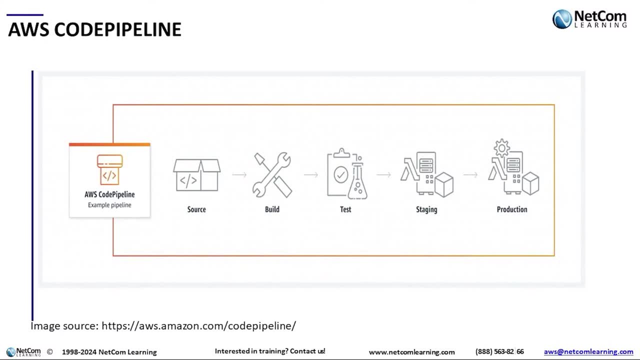 So that's called artifact. Okay, Notice, on the right-hand side, it actually integrates nicely with CodeBuild. Okay, And last but not least, CodePipeline Right. So this is like a conductor right in the orchestra. 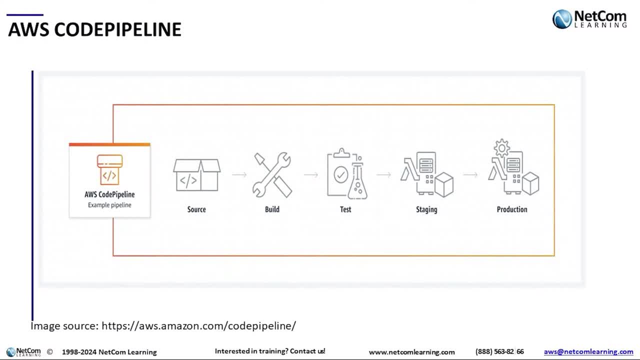 It will take all these tools that we just talked about, like CodeCommit, CodeBuild, CodeDeploy, and then orchestrate the whole thing so that you don't have to. Okay, So there you go. So CodePipeline. we'll see at the very end how it works. 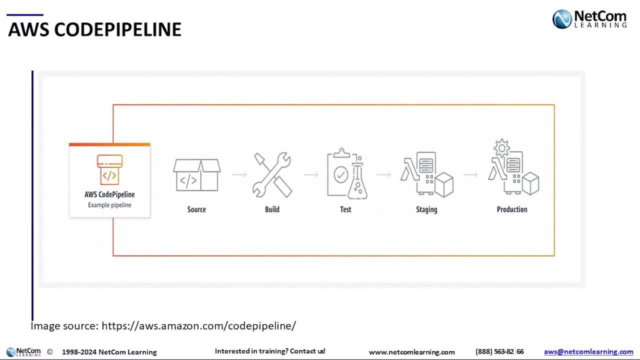 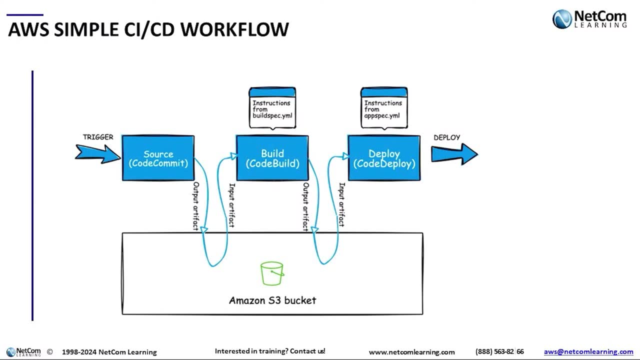 It will just bring everything together. Okay, Now here, I actually do want to give you a very simplified view, okay, of you. know what the CodePipeline does, what the workflow does, Right? So on the left-hand side you see something called the trigger. 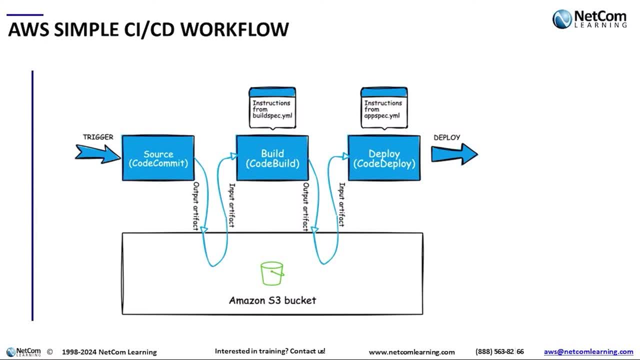 Okay. So the trigger is what kickstarts this whole automation process, That is, kickstarts the CI CD process. Okay, So what kickstarts it? Well, it's whenever there is something new to be deployed, Right. So whenever a developer says, okay, I'm done with this, I'm commit, I'm going to push it into, let's say, CodeCommit. 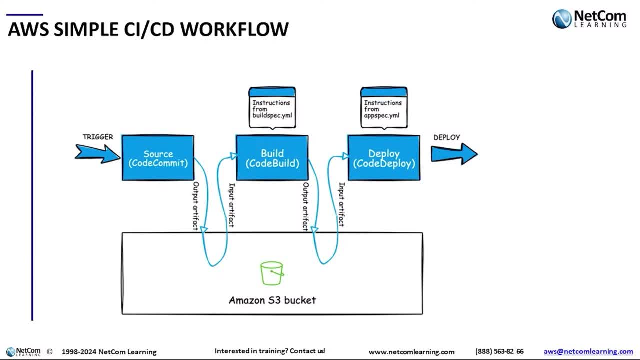 That triggers it Right. So that's why the trigger is starting at the source, the CodeCommit. So let's just assume: okay, we got a new piece of code in there and boom, the CI CD process. there's a new code inside the source in CodeCommit. 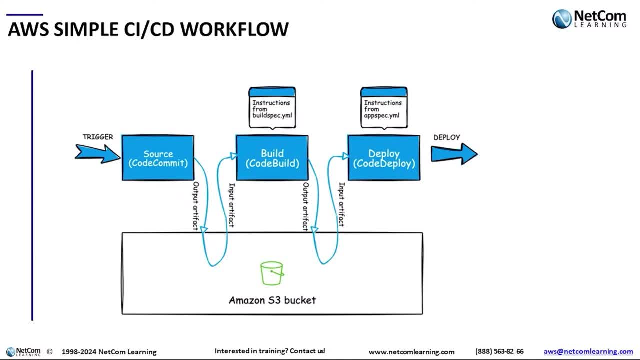 Got to get started. Okay, Then the source is stored someplace. Now it could be in S3.. It could be in CodeCommit, It could be in any places. By the way, just behind the scenes, CodeCommit actually uses S3 behind the scenes, so that you know. 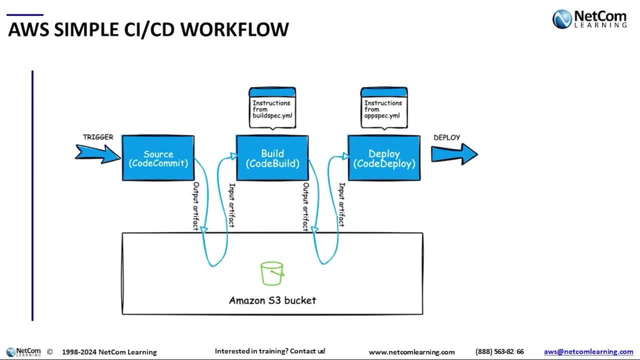 So you have an output artifact, that is, a source code from one, let's say from the source, inside some storage. Okay, So the next phase of that is then to build, isn't it? So the pipeline will trigger and say, hey, there's something ready to be built. 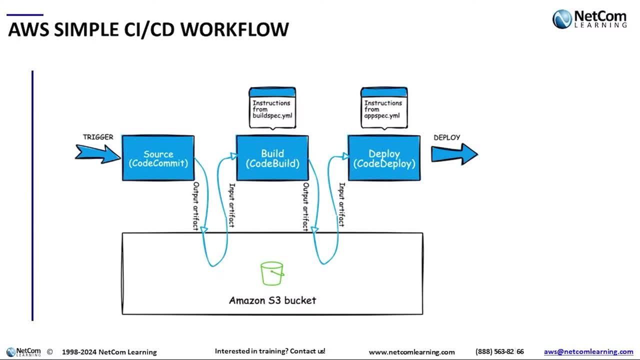 Okay, And notice I have a little kind of callout on the top. It says instructions, okay, on how to build stuff. Right, And it's in a file called buildspecyaml file. Okay, Buildspecyaml file. So buildspecyaml file tells CodeBuild what to do. 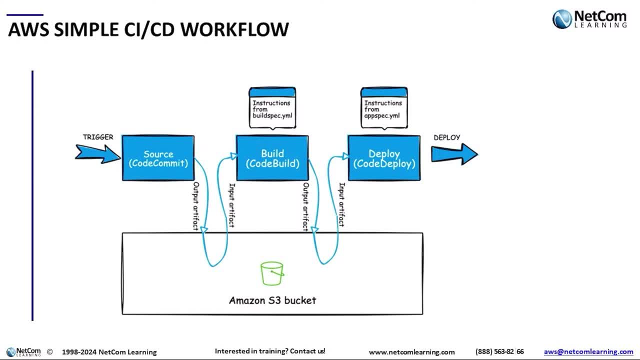 What command do I need? What am I building And where am I putting that after I'm done compiling it, let's say, or creating a package? So notice that on the right-hand side of the CodeBuild, the output artifact actually goes right into S3 as well. 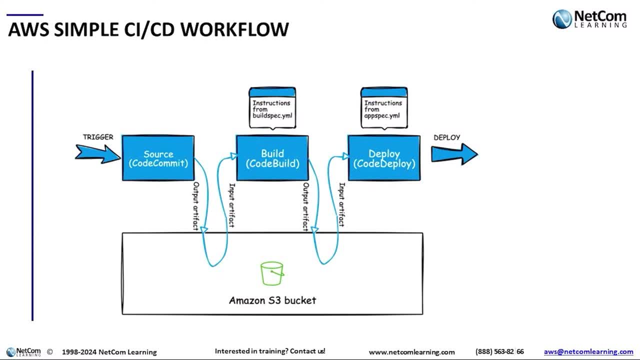 Right, Okay, So that's the output. So that is the artifact that I'm talking about. That is the program that's going to be deployed. Then CodeDeploy says, huh, look at this. CodeDeploy says, huh, look at that. 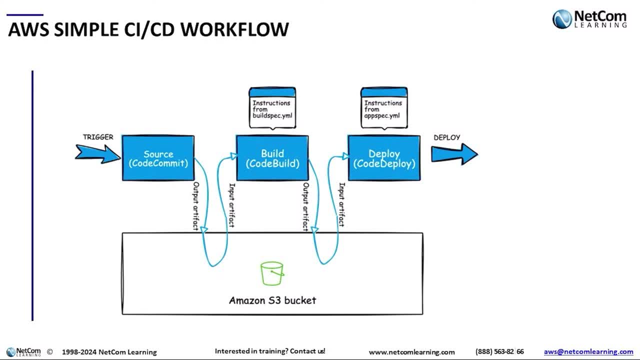 There's something to be deployed. There's a new artifact waiting for me to deploy, So CodeDeploy will grab that artifact right from, let's say, S3.. And notice another callout Instructions from appspecyaml file. 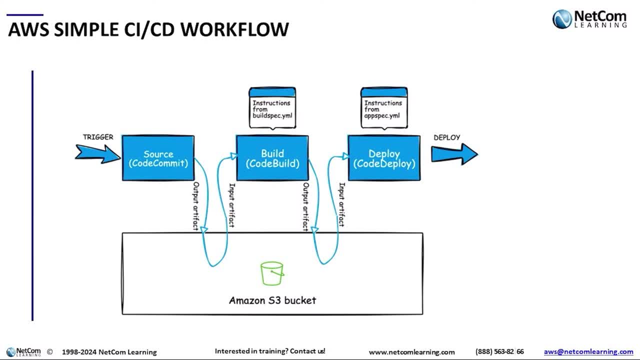 Yeah, it's a different name, But appspecyaml file is what CodeDeploy looks at and say, okay, so who do I deploy this to Which servers? Right, And do I have to run anything? you know when I deploy it. 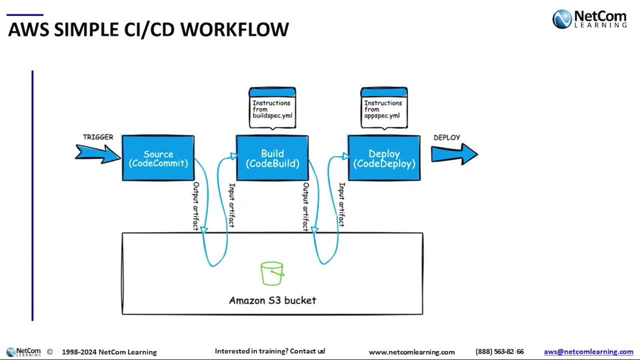 Do I do blue-green? Do I do in-place deployment? What do I do? So all those instructions are in the appspecyaml file, Then it gets deployed. Wow Okay. So it's very simplistic, but this is basically how a simple CI CD workflow works. 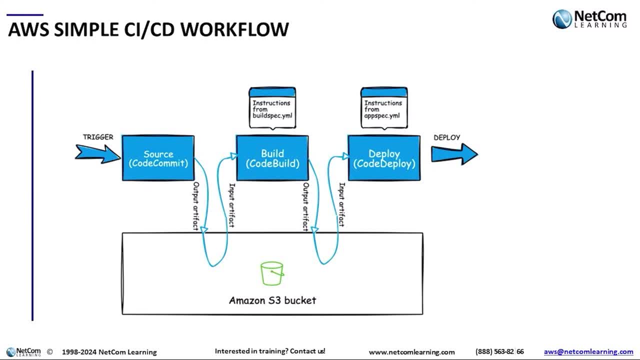 I hope that was clear. So this actually concludes my very first section of what is DevOps and what are the AWS DevOps services. If you have any questions, please do let me know. Okay, If not, let us go ahead and do a bit of an introduction of the sample that I'm going. 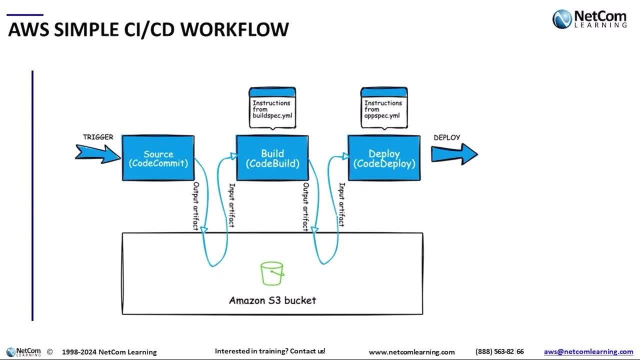 to be showing you right. So I figure these concepts- if you're brand new to it, you know you may say oh, it kind of sort of makes sense. But I think it's much better if you actually see it in action. 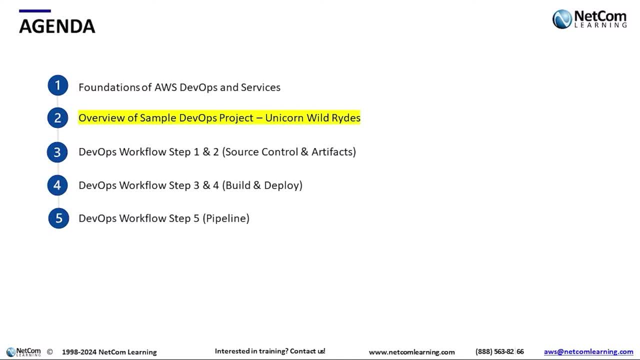 So here we go. So I'm going to go into the overview of this particular project that I'm going to show you. It's a full introduction to all the code services that I've just mentioned, And this is available online. AWS makes it available publicly online. 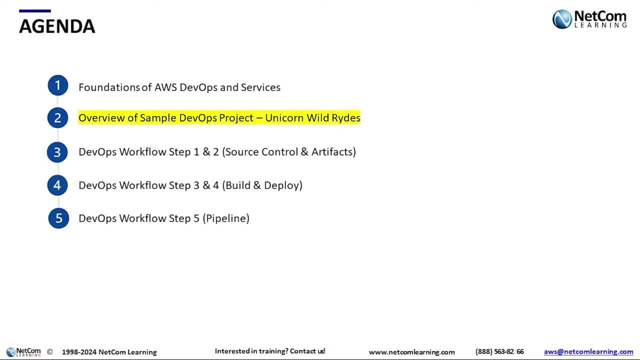 So, you know, after this webinar, you know you can go there to that site and I'll give you a link to it and you could try this out yourself. But I think that this particular tutorial right that AWS has available is, you know. 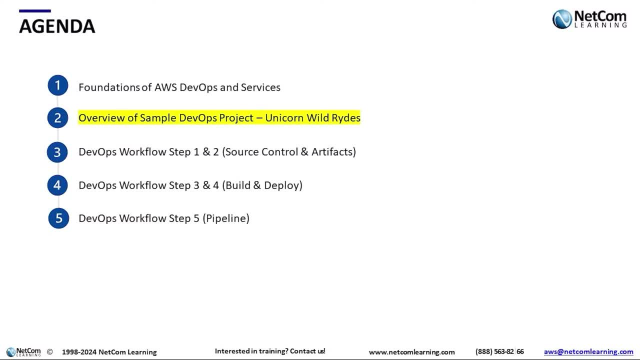 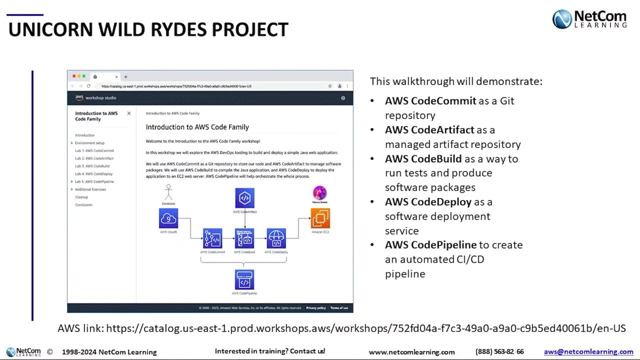 it's short enough And it's comprehensive enough. It's comprehensive enough to show you the DevOps process from the beginning to end. It's called the Unicorn WildRise. Here we go. So this is the site. By the way, I have the link, you know underneath. you know AWS link, you see at the bottom. 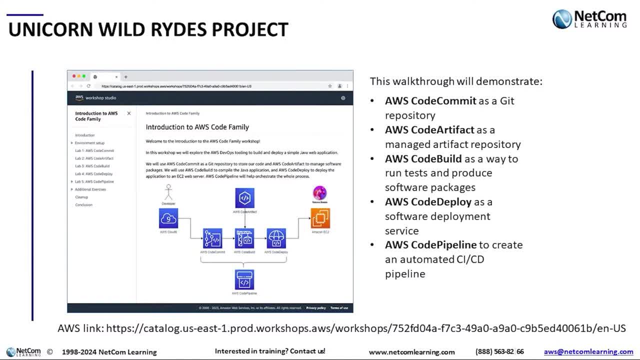 So it's called the Unicorn WildRise Project And there is a website to it. Like I said, it's freely available. Check it out. So I'm going to be walking you through this. So I actually did this. 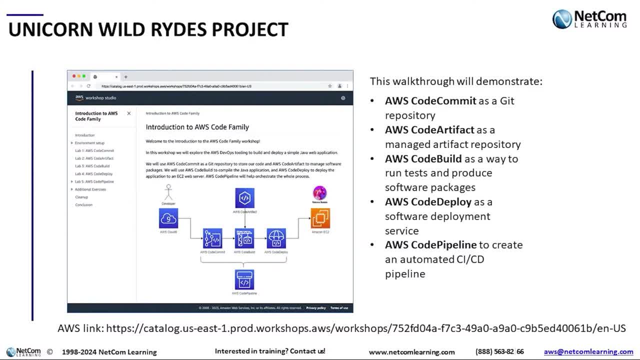 And I captured all the major screenshots while I was actually creating the WildRise project And we'll go more into detail, But it's actually a walkthrough of look: CodeCommit, CodeArtifact, CodeBuild, CodeDeploy and CodePipeline. 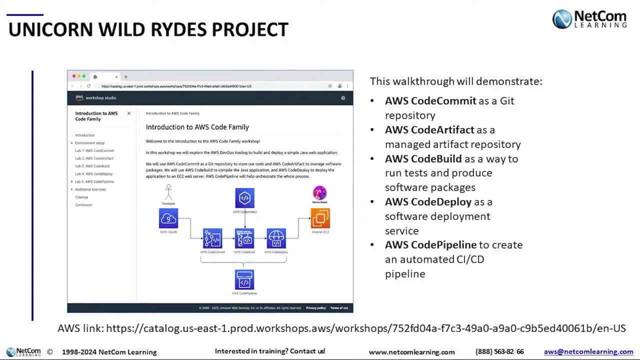 Look at that right. So that's the complete set of AWS DevOps tools that I introduced to you, Okay, So you're going to get to see the whole thing, Okay. But one thing to keep in mind, though, is that the way to approach AWS DevOps and its 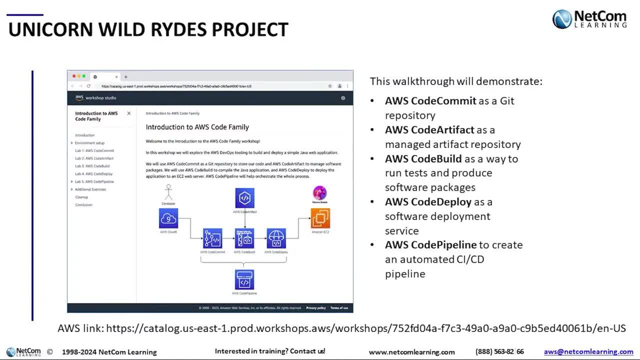 tools is to make sure that each of the components are working. Make sure that the CodeCommit is working. you know, Artifact is working, the Build is working, Deploy is working, And once you know individually they're all doing its job, then you put them together. 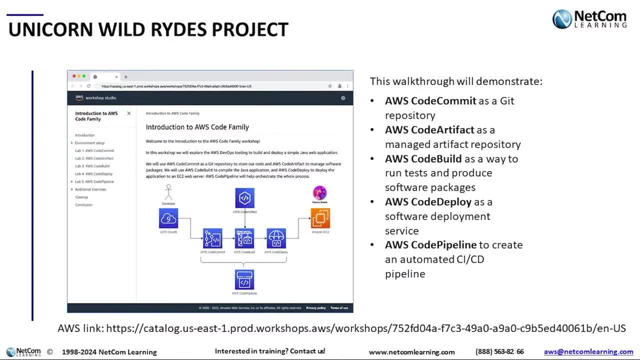 using CodePipeline. So you know, the entire automation from beginning to end comes into play. From beginning to end comes at the end. Okay, But once you have it all set up, then all you do is you know what they call it wash. 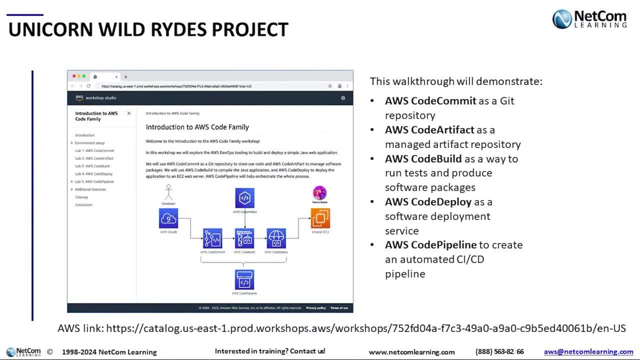 rinse, repeat, Right, Okay. So you go through that cycle right Once you have it created, Okay, But it does take, you know, a little effort to initially create it, And that's what we're going to go over right now. 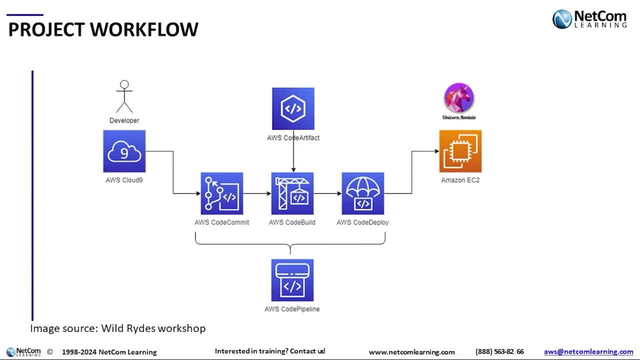 So the project workflow is going to look a little bit like this, So you probably noticed that way. on the right hand side, okay, you have something called Cloud9.. Now, that's new. I haven't really mentioned anything about Cloud9.. 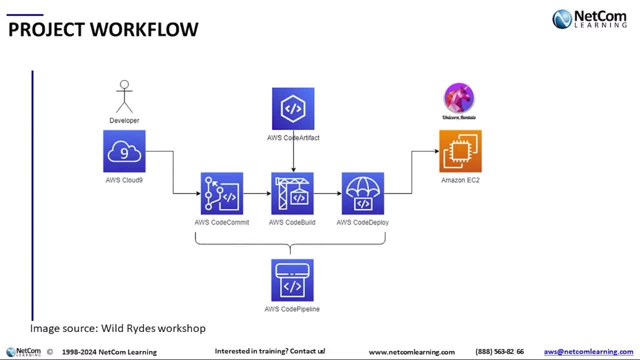 Cloud9 is an integrated development environment that AWS offers right from their service. right So you can have a full-fledged development environment, you know, with the editors, the debugger, the files, you know folder structures, even access to terminals. right that you. 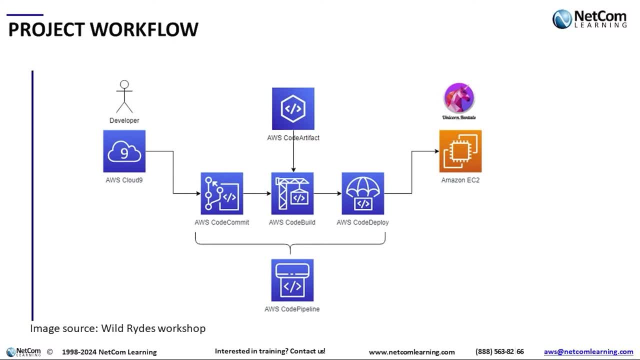 can run AWS command line interface commands with, So it's very, very convenient. So, Cloud9. We're going to pretend that this is where the developers are developing their code. Okay, So that's why they have their original source code. 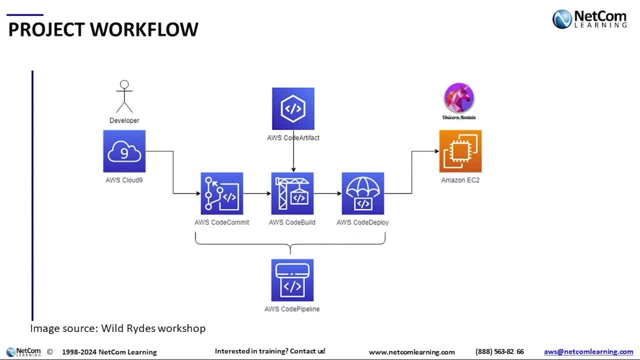 And that is going to be committed to CodeCommit right Source control version management software And that is going to kickstart the build process. By the way, it's going to be a Java application, Okay, And the Maven which is required for creating the package for Java is going to be in Code. 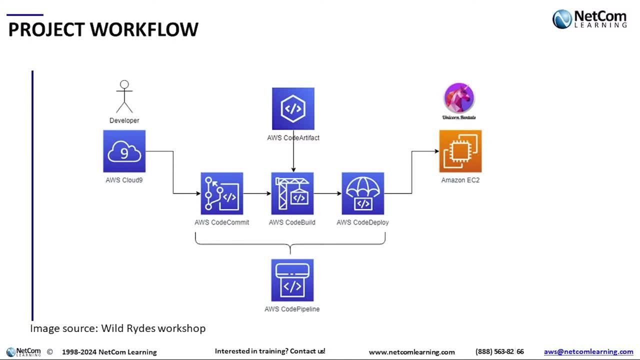 Artifact, Okay, And once the build is done, okay, then CodeDeploy is going to get kickstarted and that the Unicorn, the WildRise application, is going to be installed inside one single virtual machine, which is EC2.. Okay, Now, obviously you can have multiple, but in our example there's just going to be one. 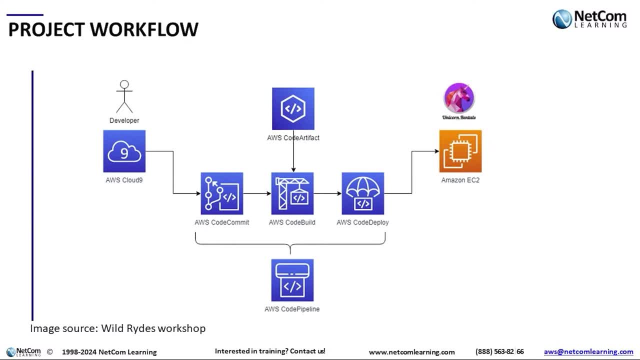 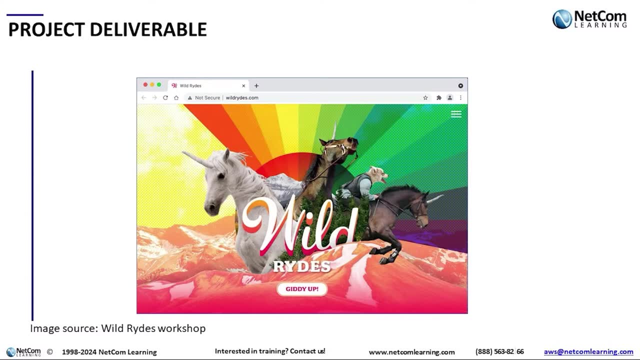 And this whole thing is going to be orchestrated using the CodePipeline, So the end product is going to look something like that. It's going to look pretty wild, Okay, So that's what we're going to do, But I think this probably is a good place to take a short break. 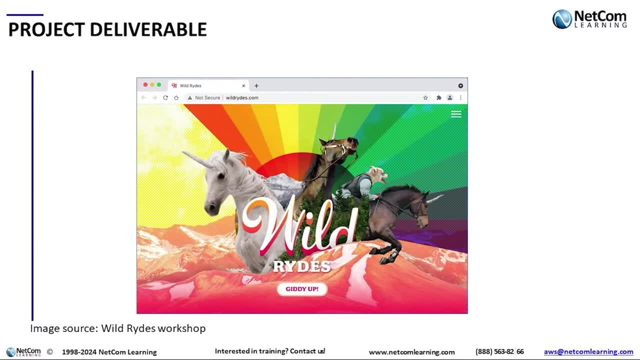 I think we've been talking probably close to an hour right now, So let's go and take a five-minute break And after five minutes we'll return and we'll get started right away. Thank you, Sure, We are now going to take a five-minute break. 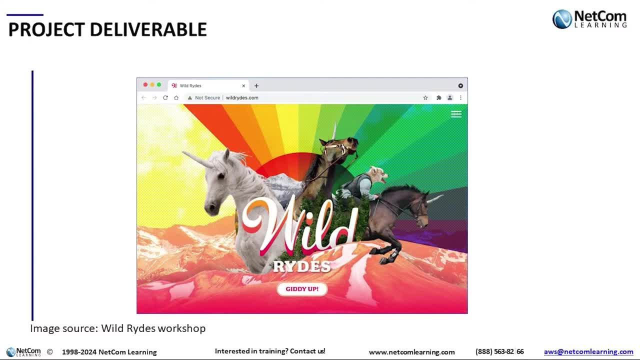 But before we do that, we are going to launch a quick poll that we want to invite you to participate in. Doing so helps us know how we can better serve you by telling us who might be interested in more information or in taking some additional training. 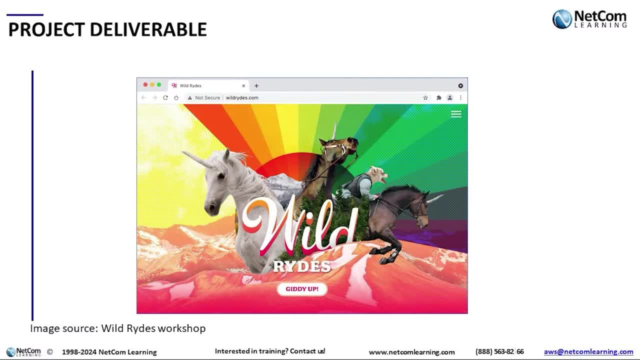 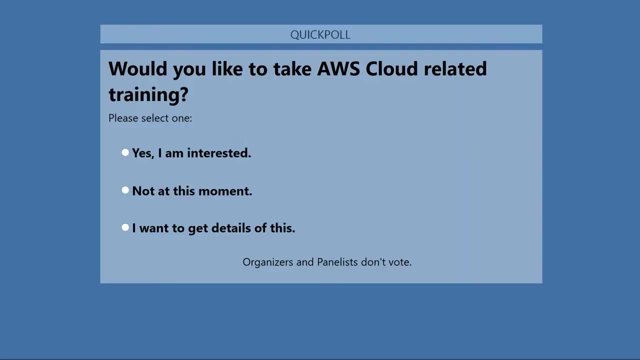 In addition, we have a lot more informative webinars coming up, So please go to netcomlearningcom backslash webinars in order to register. So now we're going to take a five-minute break. Have a great day. Bye. 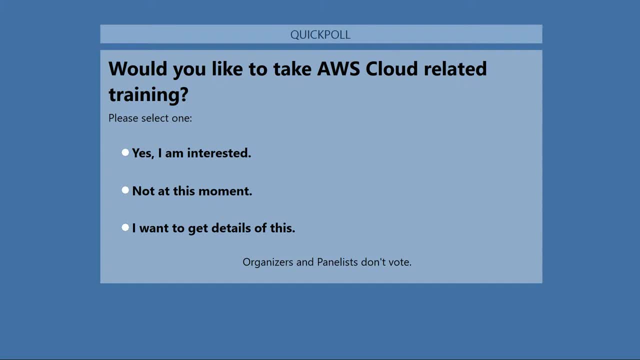 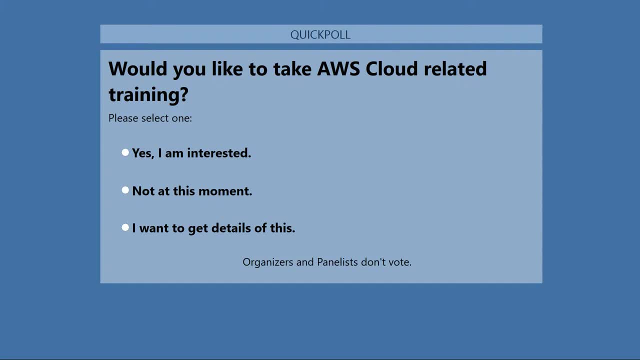 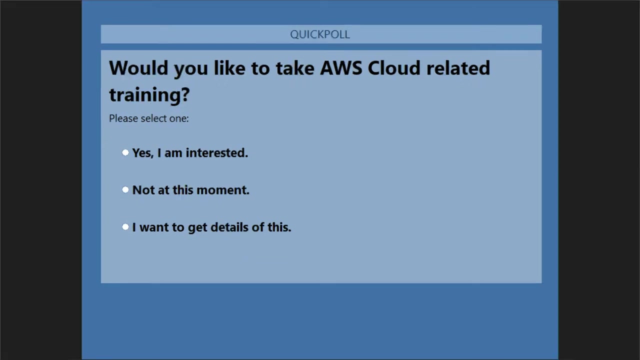 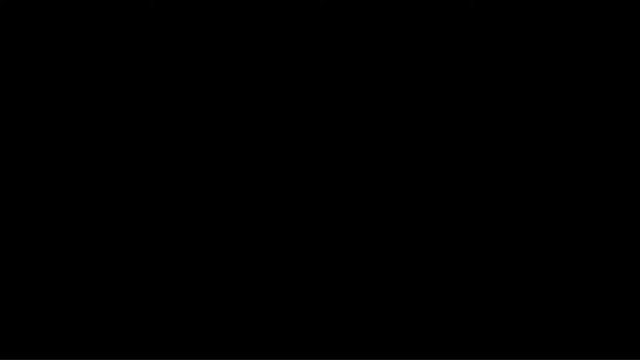 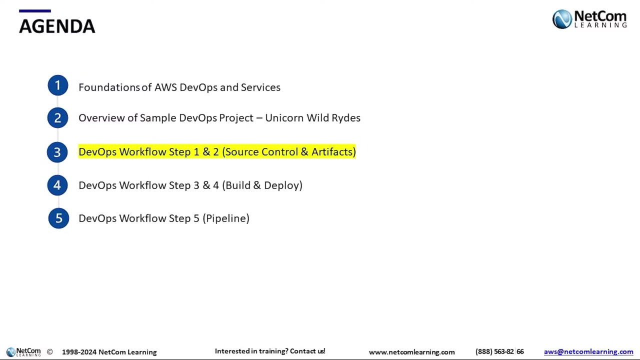 you, you, you, you, you, you, you. all right, everyone, welcome back. okay, so let us get to the actual hands-on part of it. okay, um, so, as i mentioned earlier, um, i have taken a screenshot, okay, of the actual um, the, the tutorials as i was going through it. okay, so, uh, so, don't consider this to be like the. 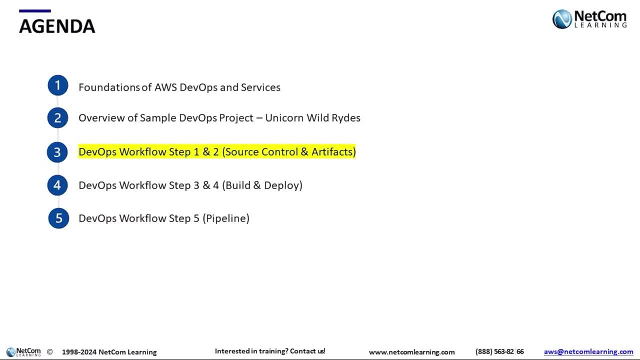 entire. like you know, from the beginning to the end, i'm going to be having a little bit of a. i have to actually skip some details, but if you're interested in doing that, like i said, you could go to that website. uh, the aws workshops, uh, that they offer publicly is very, very detailed. 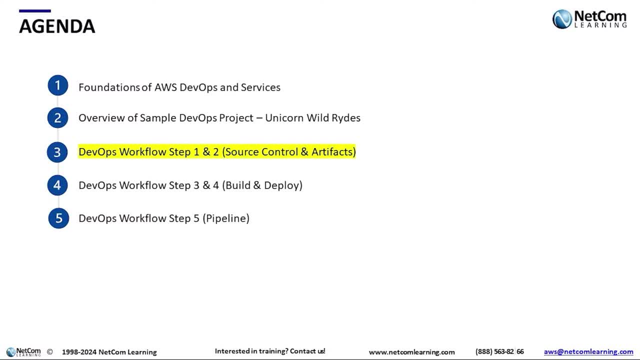 and it's very good, so give it a try when you have a chance, okay. so, um, the the entire process of getting this wild rides right, uh, live, um, usually takes around three hours, okay, but i'm going to do that in 30 minutes, okay, all right, so so let's go ahead and start the first step. 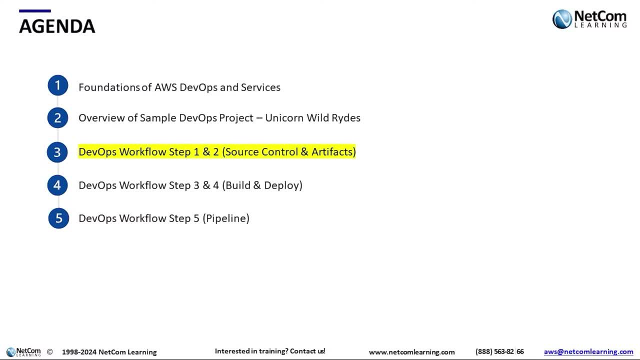 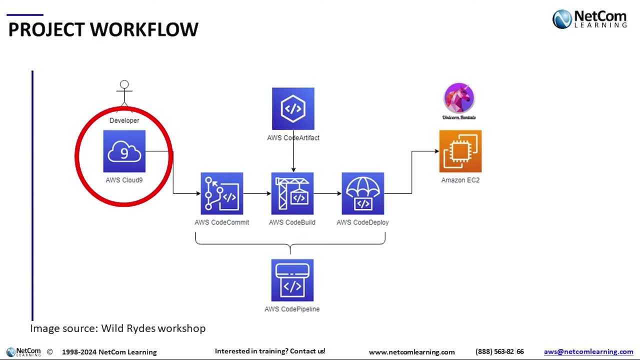 is the source, control and the artifacts. so here we go. if we were to look at the, the workflow, um, this is basically what they have in there, right. so, right now, uh, the initial thing is step zero, okay, which is to set up my cloud9 environment. okay, that's basically what i'm going to do. so here we are. 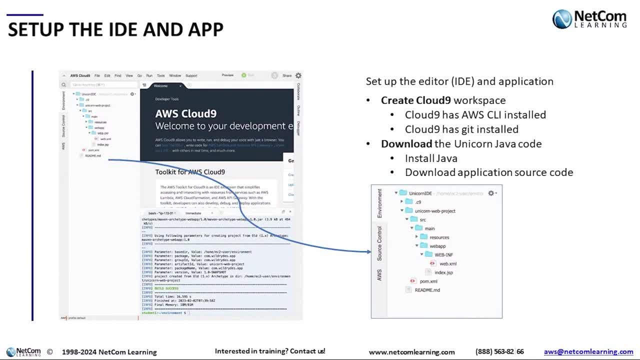 um, on the left-hand side it's kind of small, but this is cloud9, okay. so cloud9 actually has, on the very left-hand side has the file manager, and then on the right-hand side it has the file manager and then it has the file explorer. so this is where you know you can just go and download files, upload. 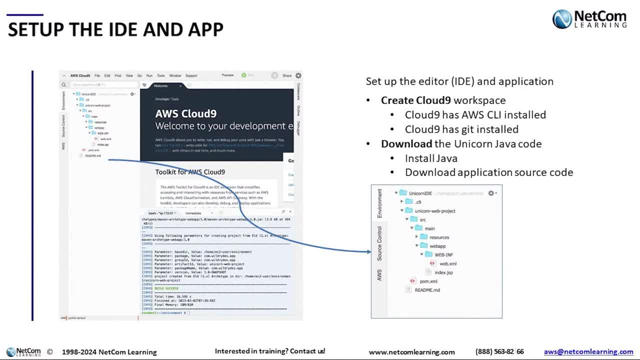 file, create files, you know, do whatever you want with management. now files. then in the right-hand side it's broken down into top and bottom. the top part is the editor page, right where you see, you know, adobe's cloud9. welcome to your development environment. that's basically where the? uh, the. 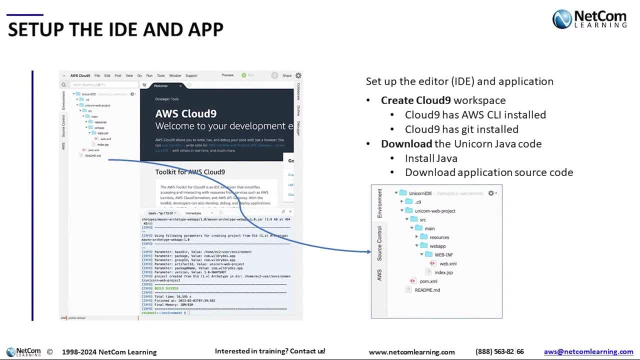 editors are, so you could write your java application, python application. what have you then on the bottom part, which kind of looks kind of a little grayish, bluish? that's the terminal where i'm going to be working with git, right, uh, to the clone, the, the repository, uh, that has the, the. 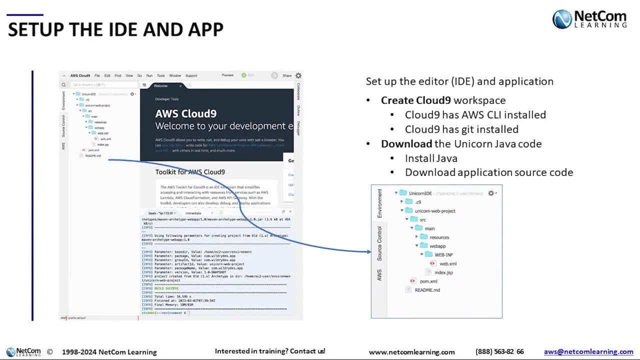 wild ride source code and i'm going to be making changes into them and pushing it back into the repository and um on, on the right hand side of the, the presentation at the bottom, i've kind of given you an idea that, yes, i've actually downloaded the- uh, the wild ride source code. that's why you see. 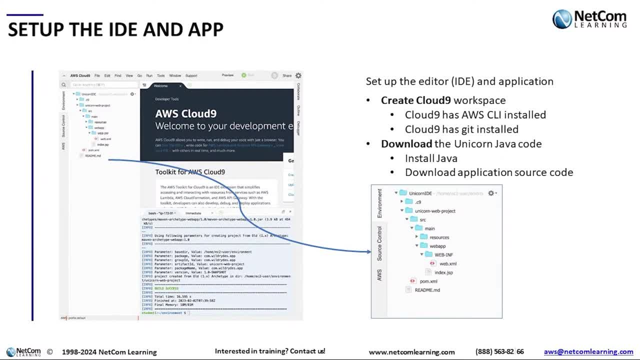 the, uh, the file structure there, okay, uh, where you have the source, the main, the resources, the web app, and then you see this thing called indexjsv. so that's going to be the top page, right, uh, initially. then you have, you know, palmxml and all that stuff, okay, so so i've already done that, i've already downloaded the. 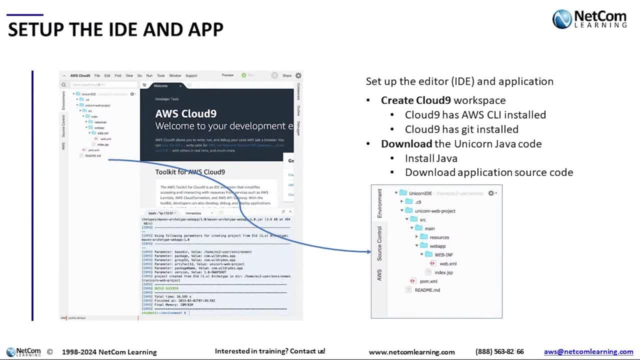 unicorn java code. um, i've already installed java in my environment and i've already downloaded all the source code that i need, and if you were to go to the workshop, they'll give you a clear link as to where you need to do that. okay, so that's the the step-by-step. 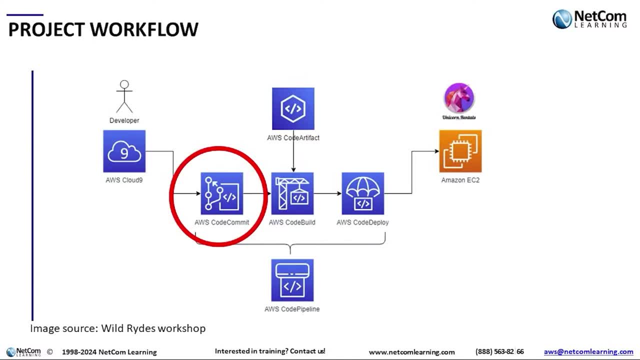 zero. all done, all right. so next one. now we're going to go into codecommit now that i have. so you have to kind of imagine that cloud 9 is my own personal environment. so, um, i'm working on the mac right now, so it's as if i'm working. you know, i have an ide: integrated development. 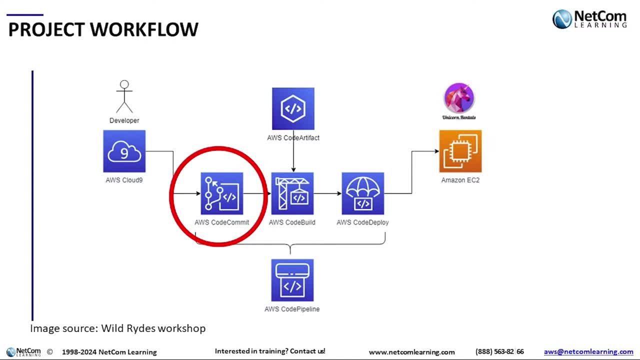 environment inside my mac and i have my code on in my mac, but in order for me to deploy it i have to upload that on to aws. so the place where i'm going to synchronize all my source code is codecommit. so if you know how to use codecommit, you can just click codecommit and it will show you. 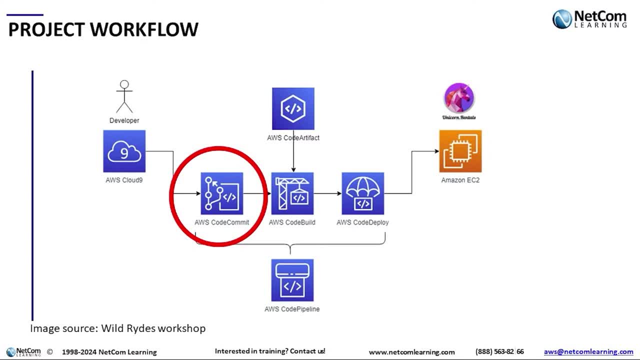 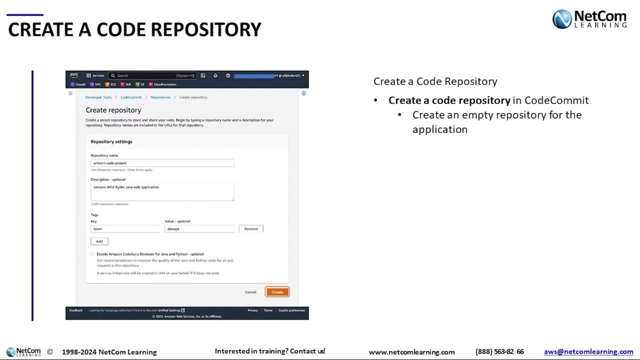 GitHub. pretty much like GitHub. Here we go. Just like GitHub: if you've used it, you have to create something called a repository. The repository is where all your source code, the stuff that you uploaded, you updated, is going to be shared with all the rest of your team. We have to create 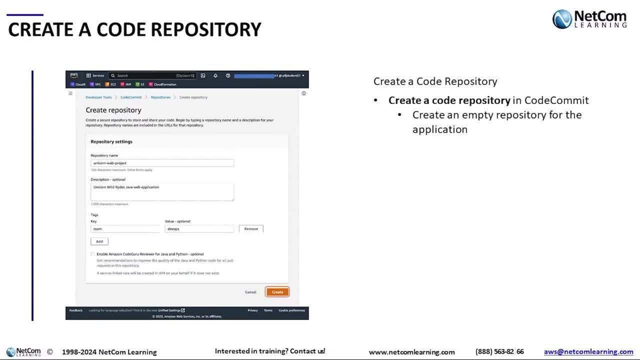 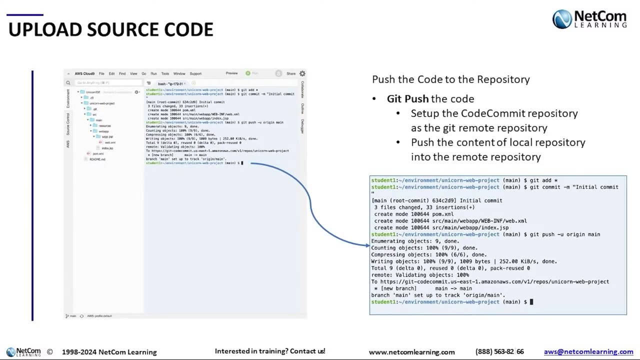 a code repository. Here I'm creating a unicorn web project repository. Initially it's going to be empty. Then, after I created this, I'm going to go back to my Cloud9, because that's where my local source code is. I'm going to be committing and pushing all the code into CodeCommit. 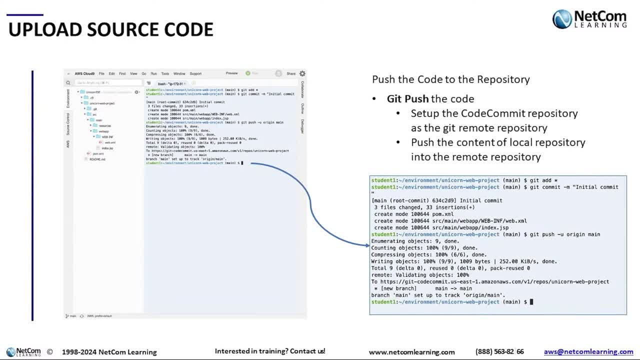 Although you don't see too much detail here. you may be able to zoom into my slide here, but what I'm doing is I'm going to set up the CodeCommit repository on the Git and say, okay, I'm in Cloud9.. I'm on the local repository here for Git and my remote repository is going to. 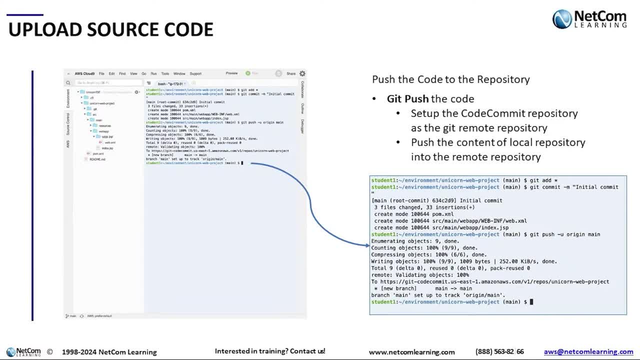 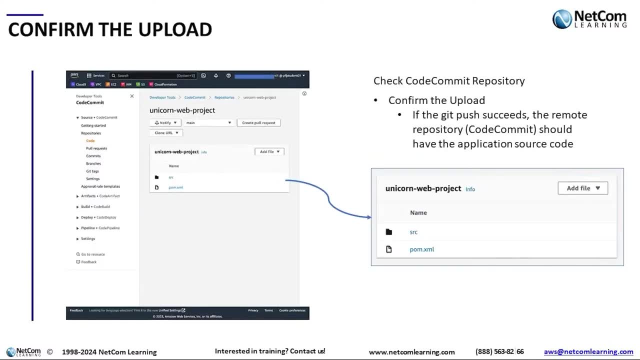 be in CodeCommit. I need to do that kind of setup and then I'm going to push the content up into CodeCommit. That's basically what I did. After I do that, I'm going to confirm that. yes, indeed. 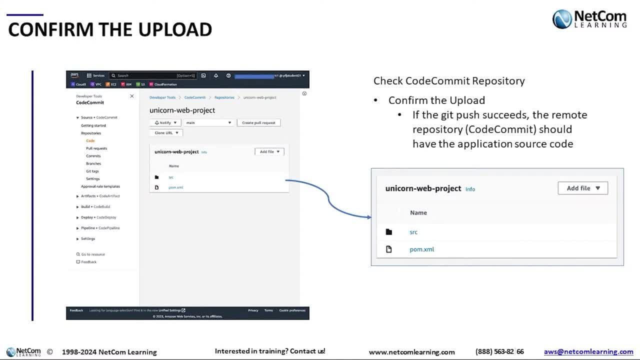 my repository on CodeCommit actually has all my files that are important to me. As you see, there I have the source subdirectory, I have the palmxml. so that tells me that, yes, I was successfully able to push the content back in. 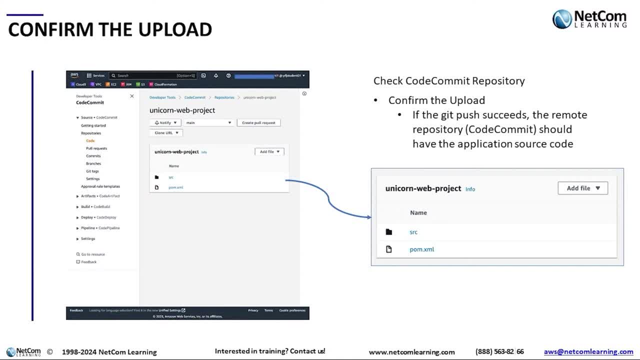 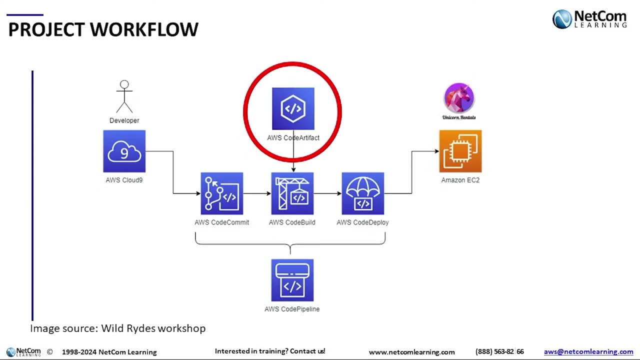 Also keep in mind that this is a process which is going to trigger the rest of the process. Remember, triggering the pipeline starts with the source code and CodeCommit is going to be that trigger, Moving on next one After I have the source code synchronized in CodeCommit, the natural thing to do. 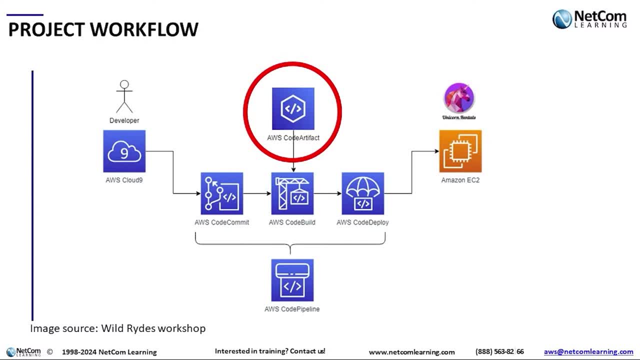 is to build, But in order to build- because this is a Java program- it needs some tools like Maven, and this is where CodeArtifact is going to come in. I explained earlier what CodeArtifact would do is give me a more stable access to these external tools that I may need in the process of building. 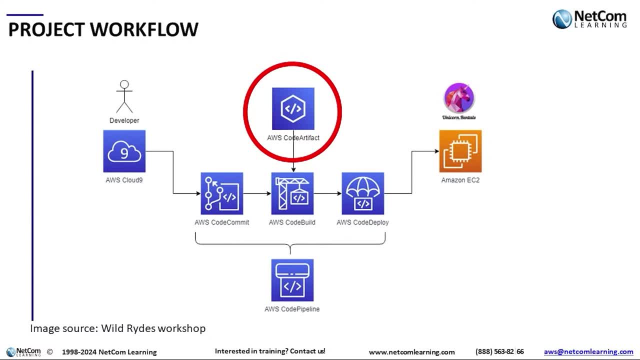 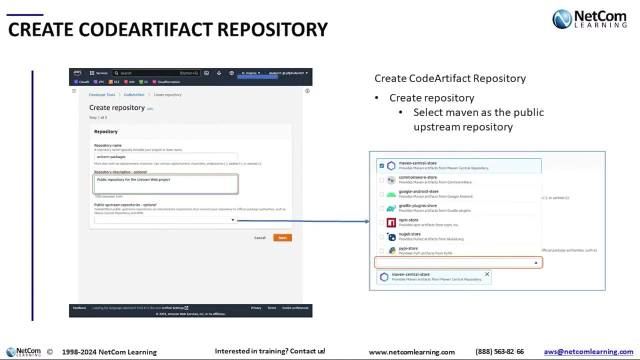 I'm going to specify Maven because that's a major tool in CodeArtifact. so let's take a look and see how we do that. Initially, I'm going to specify Maven because that's a major tool in CodeArtifact. What we'll do is we'll create something called the CodeArtifact repository. 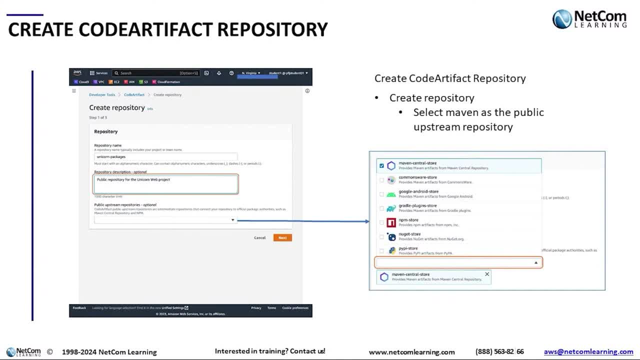 So we'll actually create a repository. I have a Unicorn package repository just created and I get to select. all right, so which external tools do you need to actually have in here? There is a pop-up screen that kind of comes in like a list. 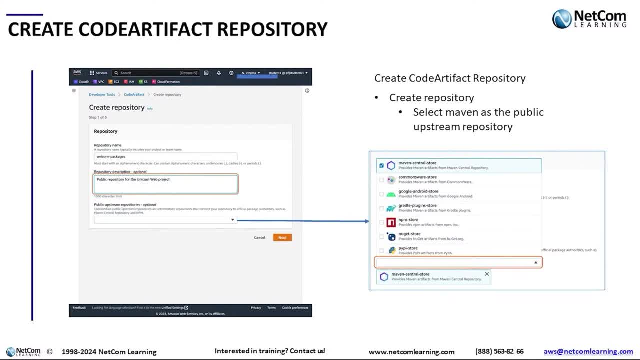 and then at the very top there is Maven. There it is Maven Central Store. That's where the Maven is going to be stored for me, so that my code build when it needs it is not going to- doesn't have to go to the internet. All it has to do is access the CodeArtifact repository. 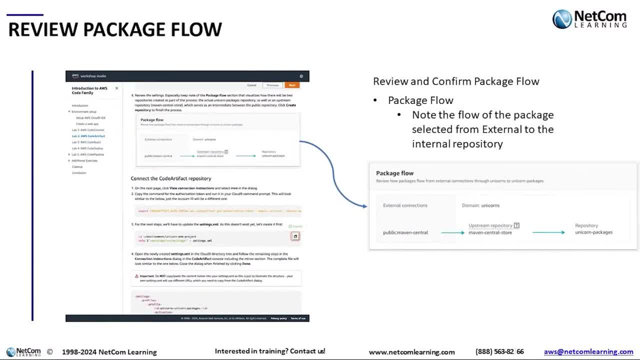 There you go And the package flow- so this is after it's all been set up- is telling you: hey, you know. so now your CodeArtifact repository is ready to go. So whenever you want to use Maven, it's there for you. okay, Now one thing we have to do is we need to be able to access that. 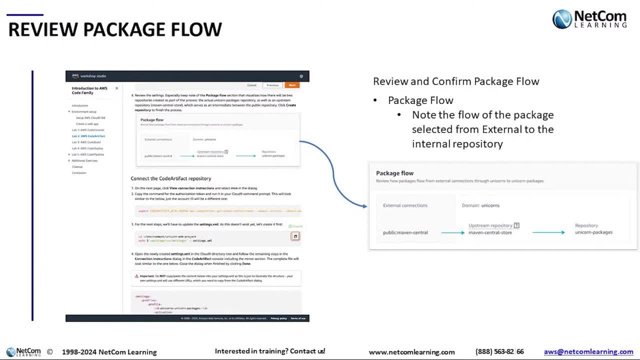 right. One thing to remember about AWS is that for anything that you do, even the services like code build, if it needs to access CodeArtifact, you have to give permission. So we'll talk about those permissions and when we do, you know, I'll kind of you know. 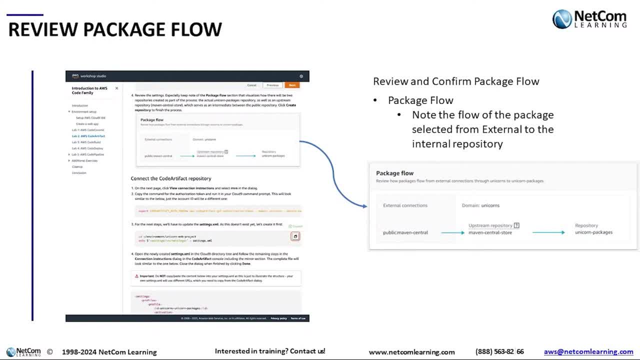 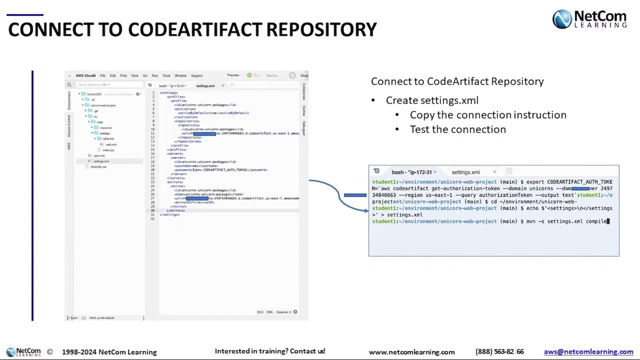 point out once again: hey, you know, this is making sure that, now that we've created all these things, that the code pipeline, the code build, whatever we need to access, will have access. One thing that CodeArtifact gives you is, once you create a repository, it's going to give you a way. 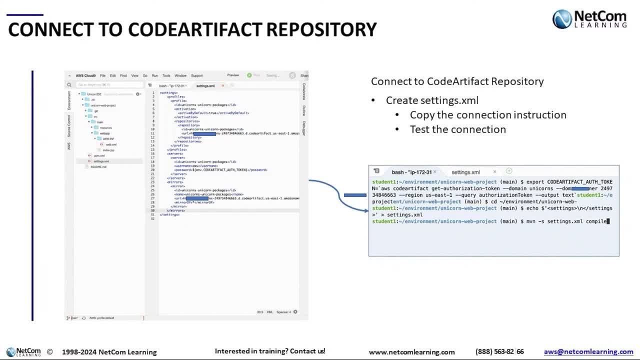 to access the repository you just created, Not just you as a person, but a program that you may be using right, such as code build. So here you know, there is a way for you to connect to CodeArtifact repository, and it's a very simple you know: copy and paste into a file called. 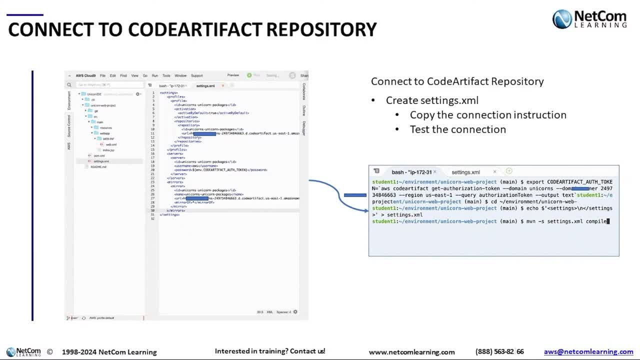 settingsxml file. So I actually created settingsxml and then I copied the connection instructions right from the CodeArtifact and then all I did was test the connection, just make sure it's working right. So right from the terminal, you see, on the lower right-hand side, I actually 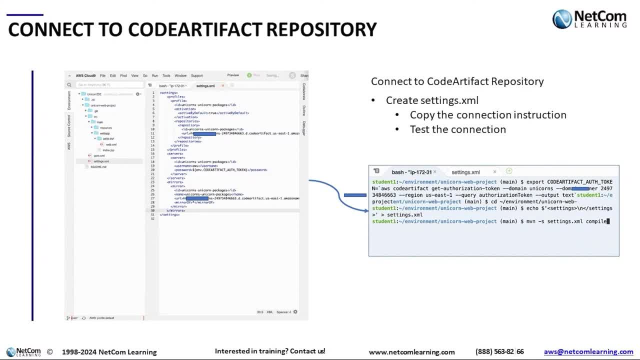 have this slide for you. So there, right from the terminal. you know I have the maven, I'm running maven mdn. space minus s- space settingsxml- space compile. just to make sure that you know, as from a command line, that I can access these things. Okay, And it worked, by the way. Okay, All right. 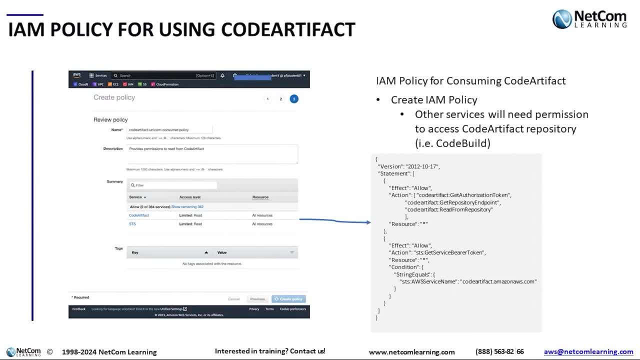 So now I'm setting up the IAM policy. So IAM policy is identity and access management Policy is about permission. Okay, So remember I told you that, hey, you know, code build is going to be accessing maven, but the code build must be given permission to access. 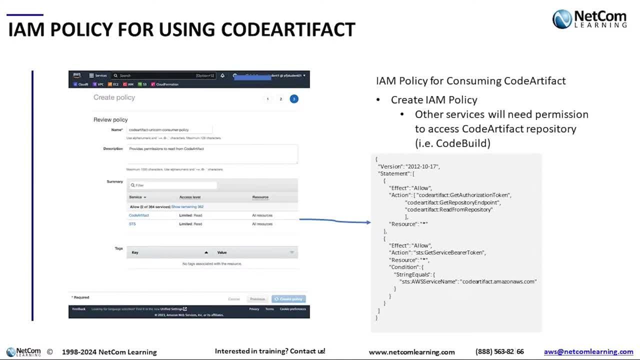 that maven. you know files that I just created inside the CodeArtifact repository. That's basically what I'm doing here. I'm creating IAM policy for consuming the CodeArtifact right. So I created IAM policy And, by the way, the tutorial gives you all the instructions on how. 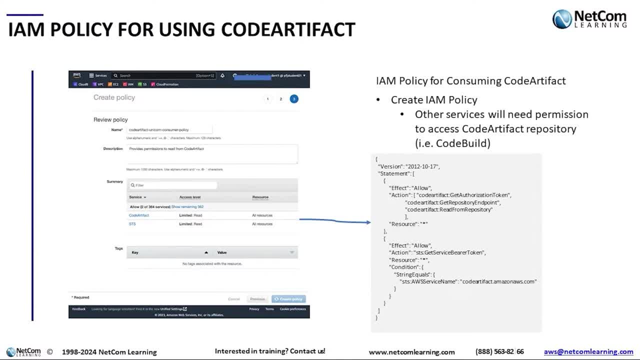 to do this right. All I was doing was just following instructions here. Anyway, just without going too much detail about what the policy looks like, you know. take a look at it in the tutorial if you need more. you know information about that, Anyway. so that actually completes this part. 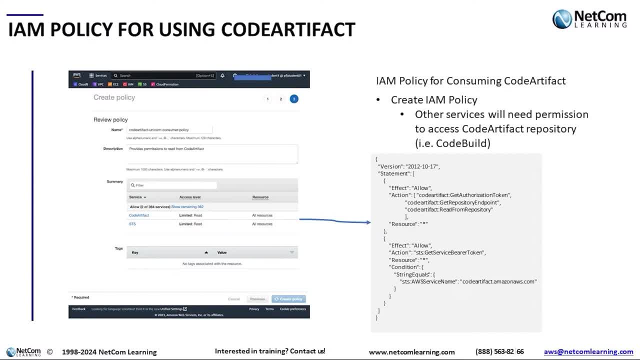 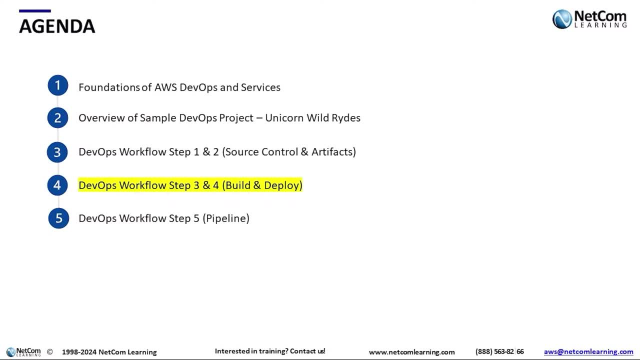 which is the CodeArtifact. Okay, Moving on, Now we're going to go into the very- you know, very- exciting stage of building and deploying, because this is where all everything kind of comes together, right, Okay. So let's go and take a look at that. 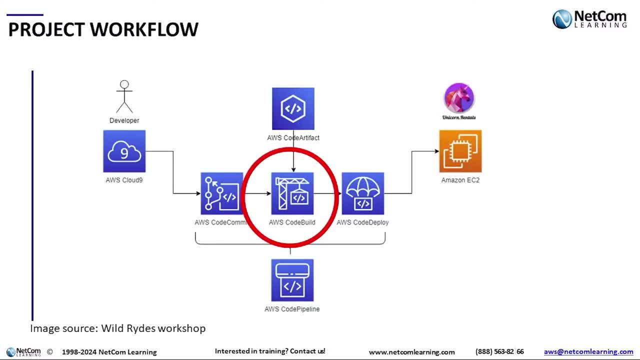 Okay, So looking from the project workflow, now we're right in the middle. the code build part of it, As I mentioned, not automation yet, right. As you see, everything is kind of manual, right, Because in order for you to automate, you have to have each and every piece working before you put. 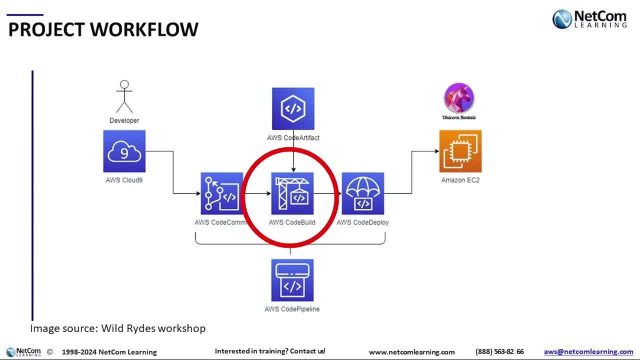 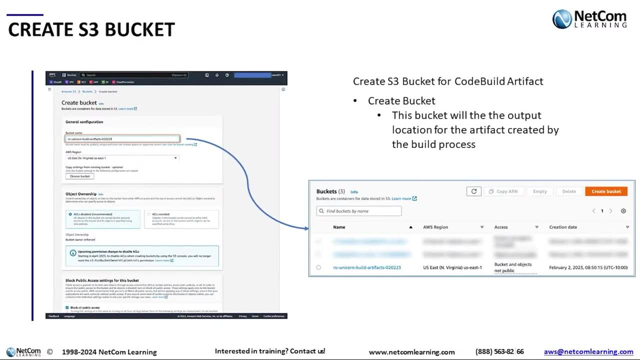 them all together and to do the automation right. So that's what we're doing. So now it's just going to be building. That's it. Okay, If you recall in my earlier discussion about all these pipelines is that there is some place where you store your artifacts right After every step. 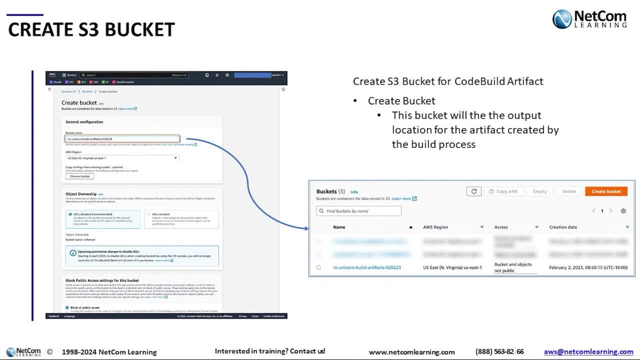 you're going to be outputting your, you know, whatever the result that you have right. So, in building, yeah, you're going to have an artifact which is the executable file. That's the most important part, isn't it? Because that's what you're going to be deploying. 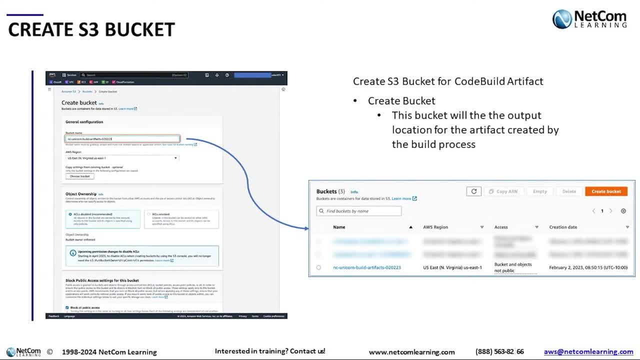 So here, code build will naturally want to save into S3. So we're going to be creating an S3 bucket. By the way, for those of you that don't know what an S3 is, it's an object storage service for AWS, So you could store like massive amounts of data you know in files inside. 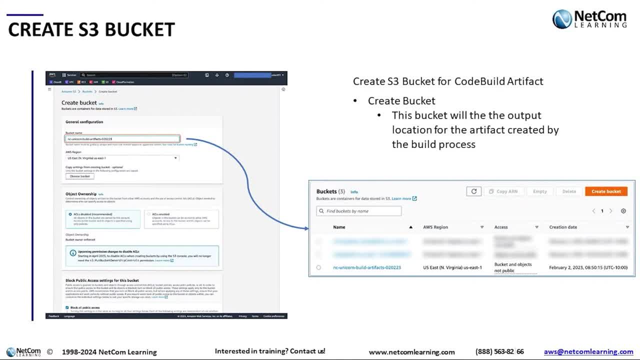 this thing called a bucket. So I've just created a bucket. right At the very end, I ran this thing, created this thing called the unicorn build artifacts bucket. Okay, So that's what I did: create S3 for code. build artifacts. create a bucket, as you see there at the very bottom. Okay. 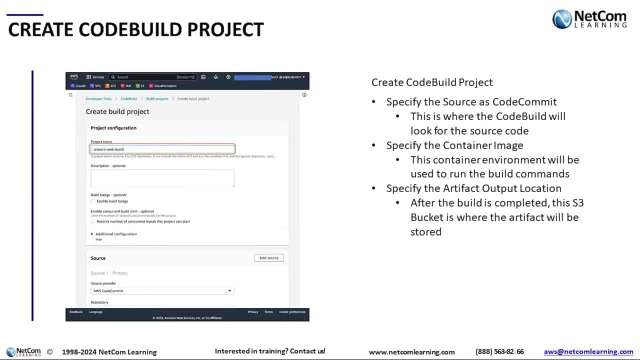 So the next one here, then, is now that I have the bucket ready to go. now I'm going to create something called a project. Okay, So I'm going to create a project. So I'm going to create a project project. So code build requires you to create a project statement. Okay, So what is a code build? 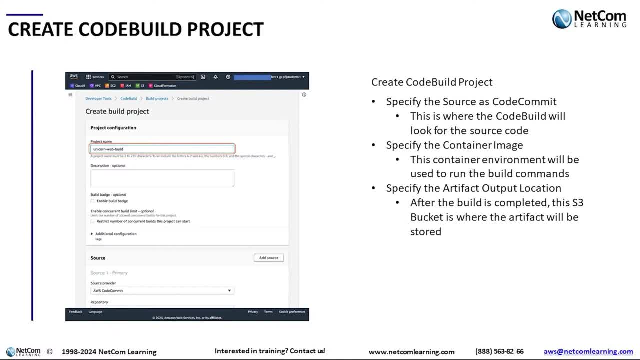 project. Well, you specify all of these components that you need to run your build. Okay, So specify the source as a code commit. that tells you: hey, you know where do I get my source code to do all this building? So I say, yeah, that's from code commit. Then I have to specify: okay, So once we 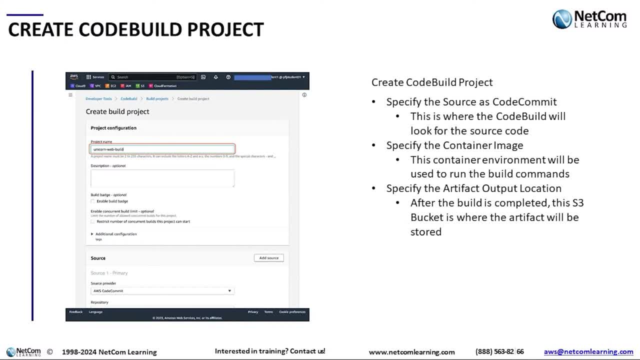 have the source code. we're going to be doing all this work and we're going to be linking, compiling, creating packages and stuff. So what environment that is. if it were a server, what kind of server would you like so that you could run all these things? So code build actually creates a container. 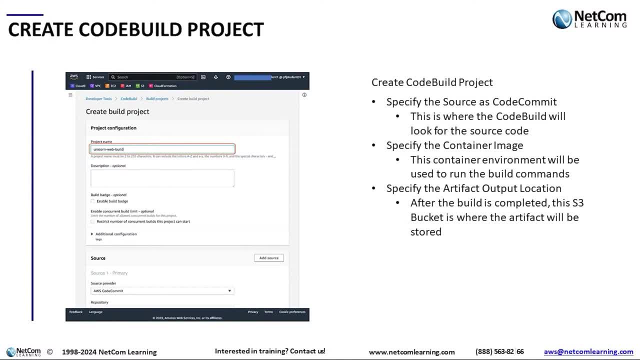 image based on the instruction that you give it right here. So you specify the container image, what kind of environment to run and build your build commands. Okay, So that's where you specify it. Then where do you output, right, your artifacts? So we just kind of created the bucket. 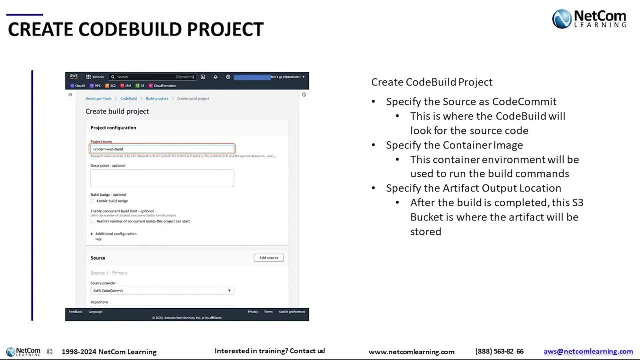 So here in this project, you're going to specify: yeah, it's that bucket that I just created, you know, the unicorn bucket. Okay, So that's where we're going to be outputting the end product from this whole process. All right, So that's what I did. I created the code build project here. 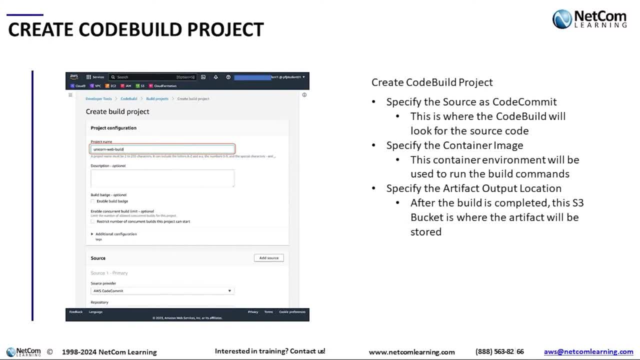 But this is not enough yet, because you know if you are a code build, it says okay. so you told me that. you know you wanted a Linux, you know image and you know this is where I get. 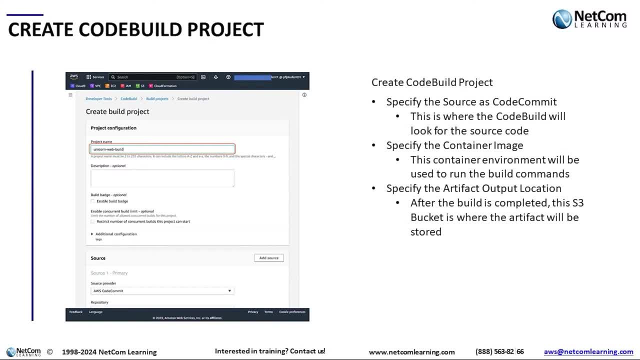 the file, and this is where I'll put the file. But what is it Like? what is it Python, Is it Java? Like what kind of command? Like what kind of tools, Like? what do you want me to do? All right, So. 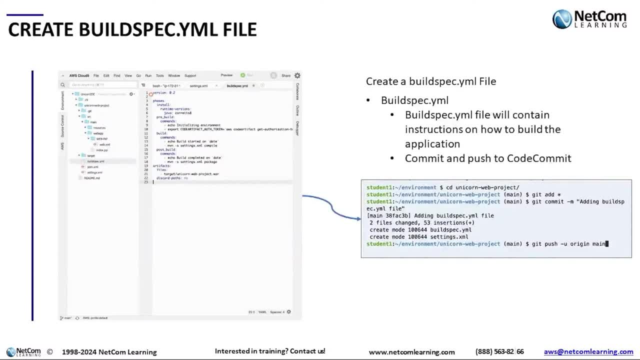 that's the next step. Okay, So code build is going to be looking for a file- By the way, it's all lower characters- a build spec, that YAML file. Okay, So the build spec YAML file are the actual build commands, right, that you're going to be running. So it's a separate file. 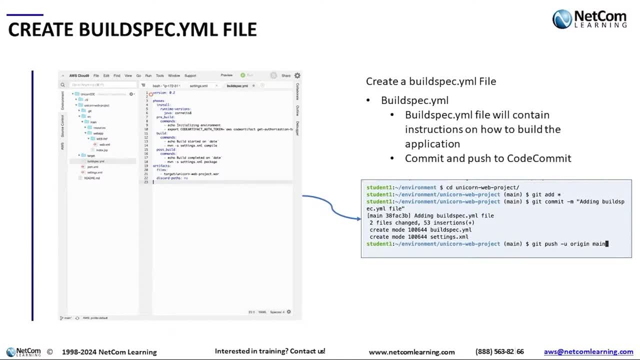 and it has to be in the root directory. you know wherever code build is going to be looking at it. So you create a build spec file here. It contains instructions on how to build the application itself. Okay, So in this case it'll be like Maven: right commands and. 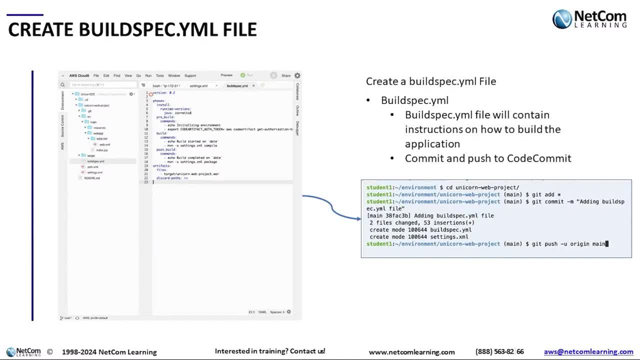 stuff. And then, once you're done with creating a build spec YAML file, right, I'm still changing this in Cloud9.. That has to be reflected back to that thing that I saved in the code commit, right? So I'm going to be committing and pushing this new file into. 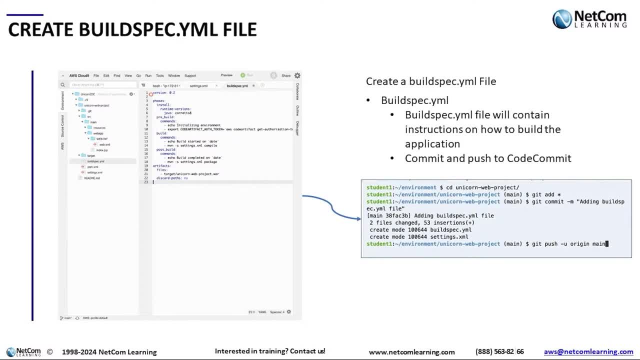 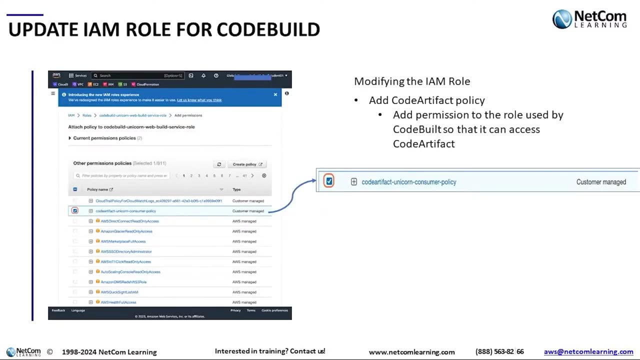 code commit. Okay, So that's what I did. I kind of pushed it over. As you see, at the bottom I have git push right back into the main branch in the remote origin, Next one here, Then right. so when you create a code, build, code build in the process. 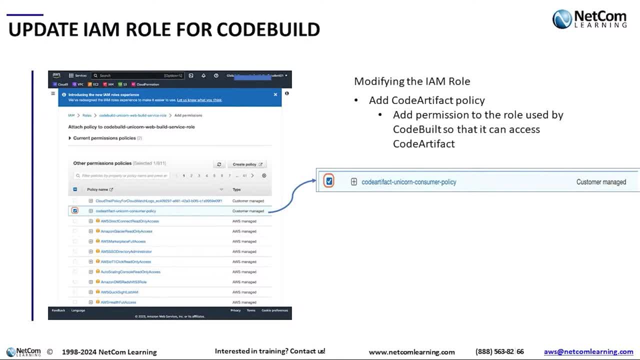 is going to ask you: hey, you know what permission are you going to give me? Okay, And there is a default permission that code build is going to assign itself if you don't do anything. But remember, in our whole process, code build in addition to doing all the rest of the stuff that they need to do. 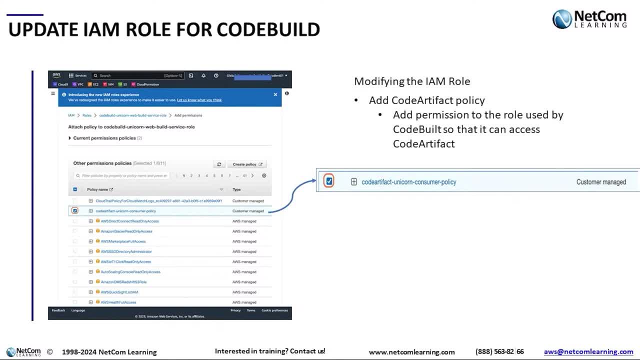 they also need to access code artifacts, right? So, remember, we created the IAM policy, right I think, the access management policy for code artifact, Okay, So we have to add that code artifact policy onto the existing code build policy. That's all I did here. All I did was I. 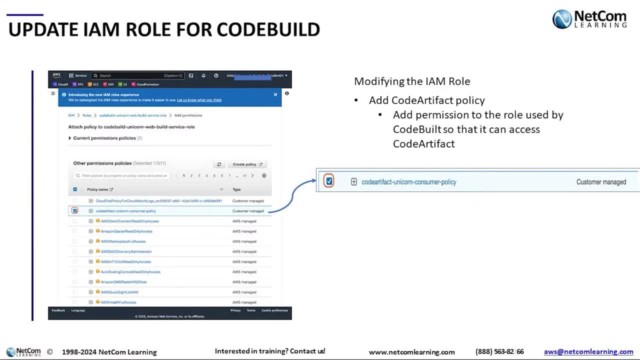 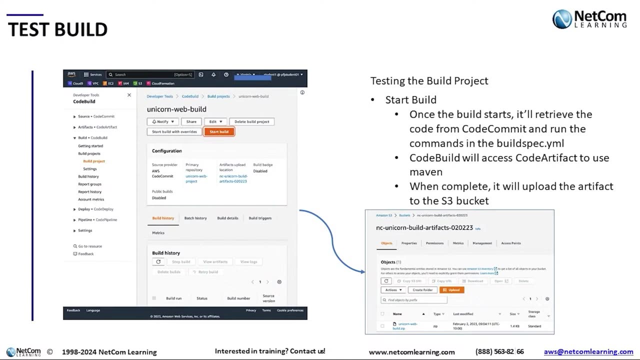 just kind of added one policy, the one that I just created- onto the existing code- build IAM policy. Then let's test it. Okay, So we're going to be testing this, We're going to test build. So there is a button right. You go to the project and you click on that button that says start build. 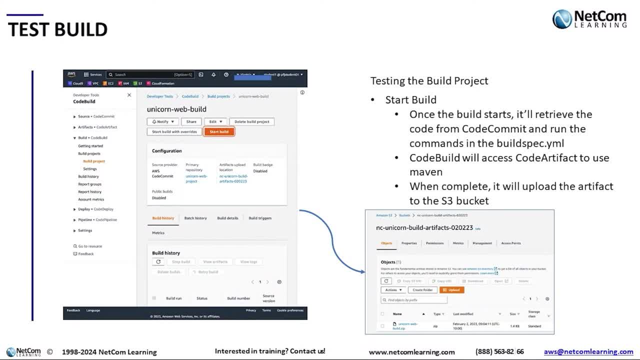 That's it, Okay. And but what you know if it, if everything worked, okay, how would I know? right? So there'll be two indications whether the build completed or not. I mean, there are others too. You can look in the log file, obviously, But one is going to the code. build is going to visually tell me: I'm done. 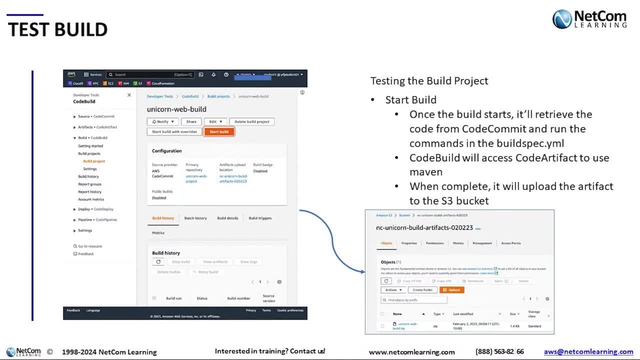 Okay. So if it errors out, it'll give you a bright red message that says error, Okay, And if it's successful, it says yep, I think everything's successful. But there's a second place that I'm going to look for, which is my bucket. right, Because if the build is successful in my bucket, 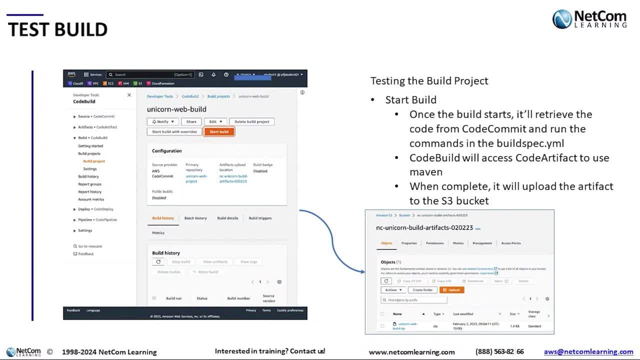 right, the output bucket, right. There should be a zip file, in this case, Okay, Which is going to have a war file inside, Okay, So if I don't see anything in the bucket, then I know something, and the artifact is supposed to be copied to that bucket. So that's what I'm looking for. 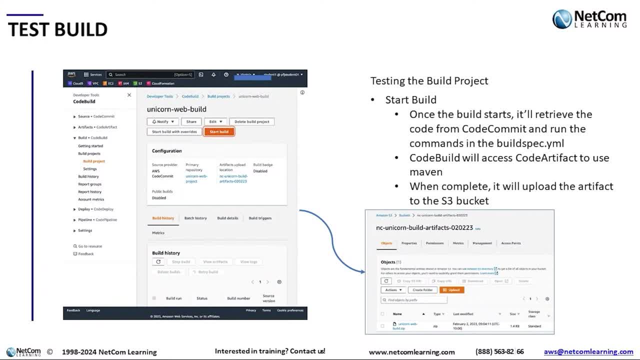 I'm going to look into the bucket And in fact, on the screen on the left, so that is the build right, But what you see underneath my words on the right-hand side, so that's actually the S3 bucket. Okay, And kind of hard to see maybe, but at the very bottom of that. 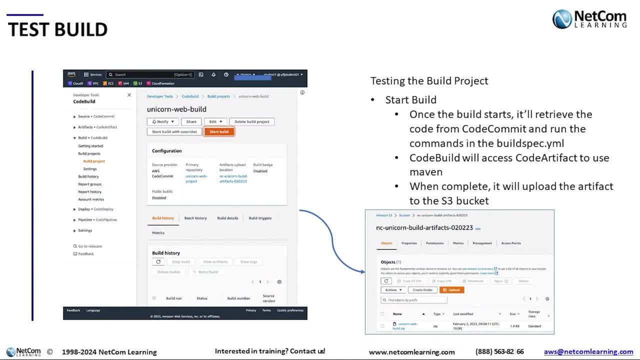 there is indeed a zip file. All right, So yeah, succeeded. Good to go, Okay. By the way, one thing to make sure that you do okay is that I got to tell you right, I actually failed the first time, mainly because I forgot to commit and push my settingsxml file. 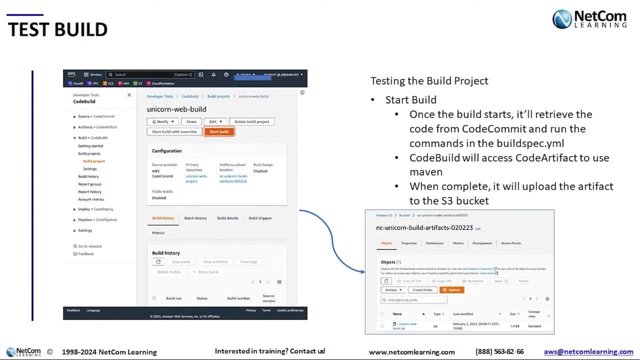 right. So, and that's the- oh, my goodness, I didn't put that in there- Commit, you know, commit and then push and make sure that goes into the code. commit so that when code build looks for it, it sees all those, you know, all the other files that it needs to connect to, you know. 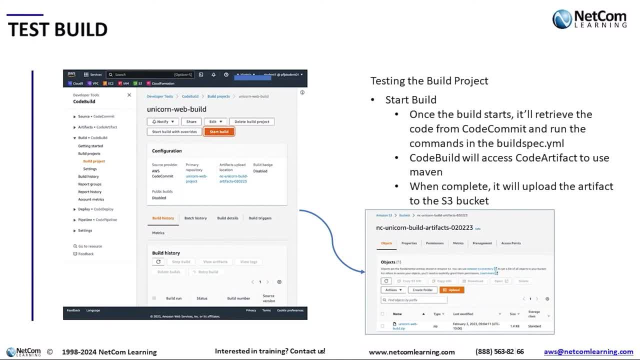 code, artifacts and stuff like that. Okay, So once we start to automate everything, we don't have to worry about it, about, you know, missing those steps. okay, like I did, But we're not automating yet, are we right? So individual steps, they're all manual. So I can't. 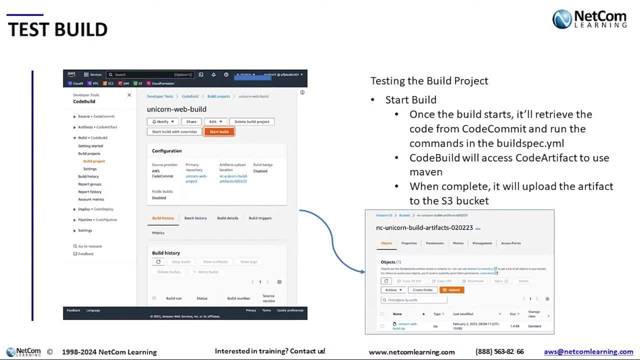 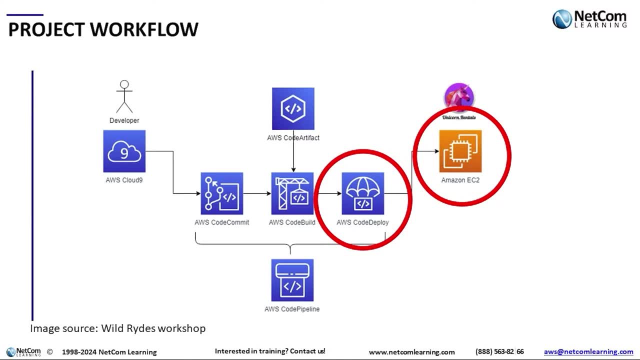 I have to remember to do that. All right then. So, now that we have the build working correctly, the next step is: yay, deploy. Okay, So deploy. then I have circles on two places, Because actually we don't have a virtual machine yet, right? So virtual machine. 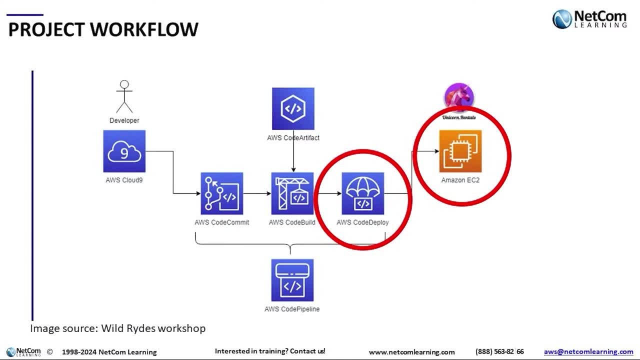 this time we're going to be installing this, you know, fantastic WildRise application. So we'll create the platform, which is EC2, and then we'll use code deploy to deploy the artifact, you know, the executable file or the jar file that's inside waiting right to be deployed on. 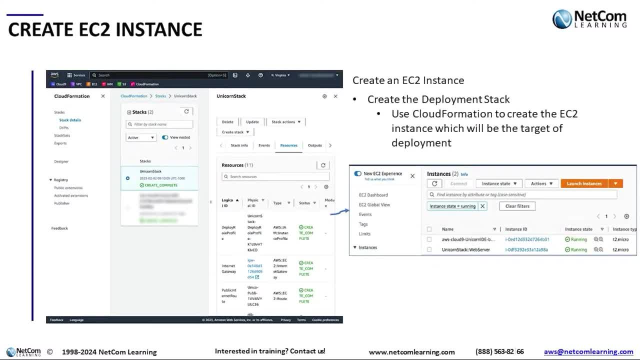 inside S3.. All right, So the first thing we did in the tutorial was to create. in this step is to create the EC2 instance. Okay, Remember the infrastructure's code? right? And in this case, the tutorial actually gives you a piece of YAML file that will create for you. 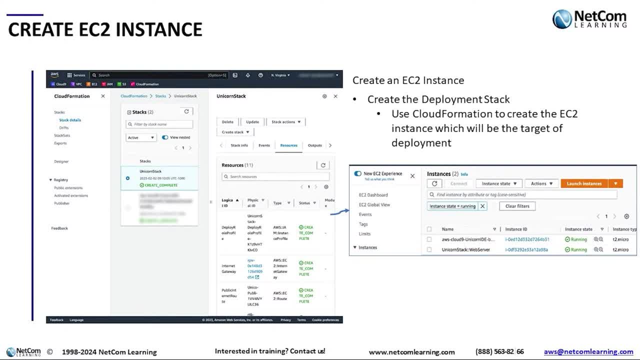 a VPC- virtual private network- and put in there one EC2 instance so that you can deploy into it. Okay, So the infrastructure's code is something called CloudFormation inside AWS, So it's an AWS CloudFormation template. So template is a you know YAML file And then I'm going to execute. 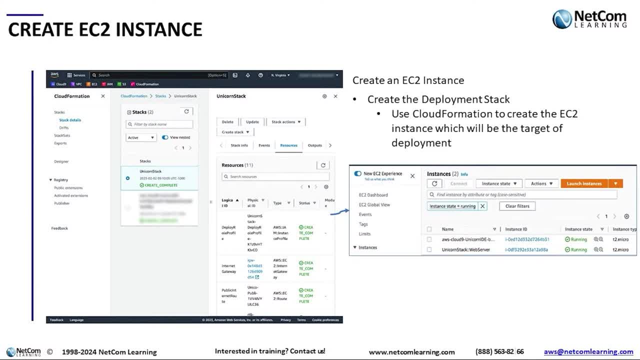 that And in the end I should see in the EC2 one server right that is ready to go. And it took maybe about- I don't know about- five minutes for the CloudFormation to kind of get everything you know working. But in the end, yes, indeed, everything succeeded, As you see on my screen. 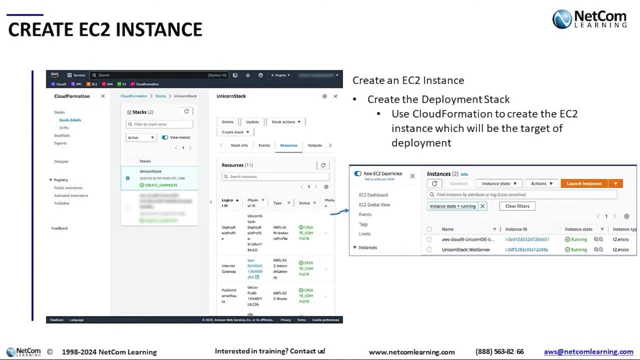 here I have all the green messages. That's what I want to see. Greens are all successful. I created it in the end, the EC2.. But you know, the proof is in the pudding right. So I went to EC2 and I 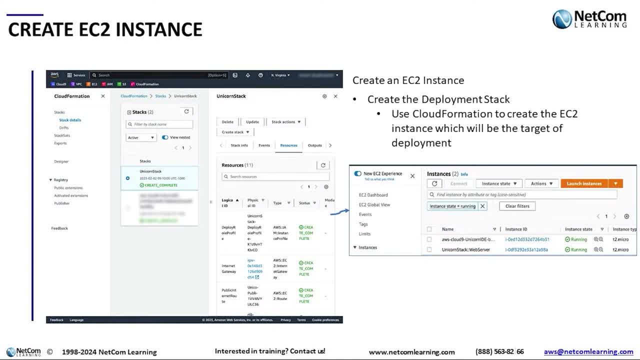 looked and made sure that there was actually a server right, And indeed there was. There was something called the unicorn stack, colon colon web server. So there we go. So now the ground is set Okay. So we have the server, We have the artifact. All we have to do is deploy it, That is to 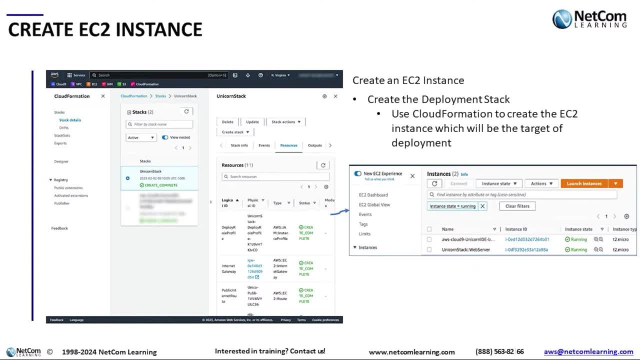 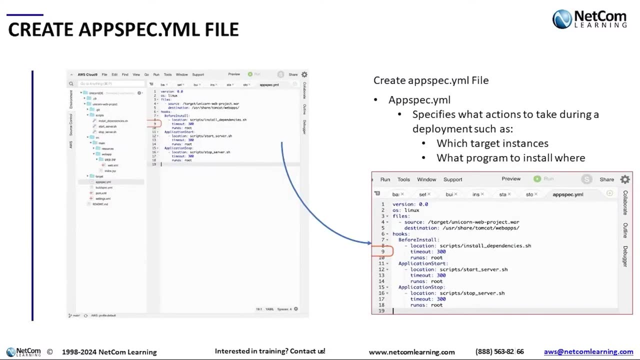 install it right inside the server And that's what cold deploy will do for us. Okay, So cold deploy, just like cold build, requires a, like a configuration file. Okay, And that is called the app spec YAML file, Right, Remember the code build took. you know, build spec YAML file In the 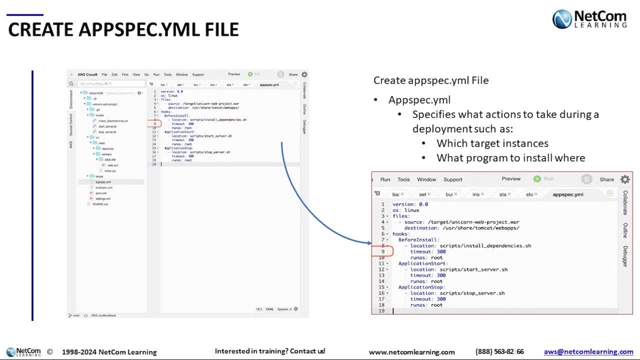 cold deploy, it will take something called app spec YAML file. Now, app spec YAML file specifies the action to take during a deployment, such as: hey, where do I install this in? Do you want it in containers? Do you want the EC2, like in the server? Do you want the AC? Do you want it in the? 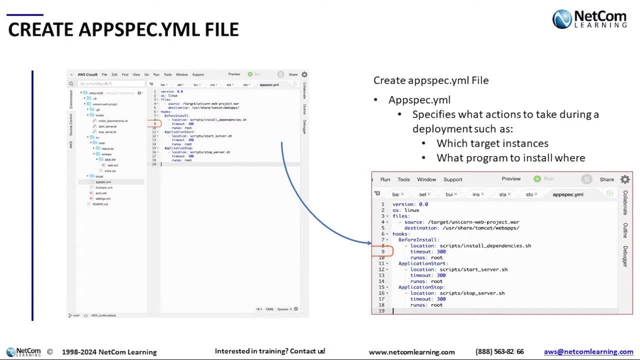 server. Do you want the EC2?? Do you want the EC2, like in the server? So then you can do that like what. okay, so that right Then which program to install and where. okay, So in the tutorial this web server's gonna have. 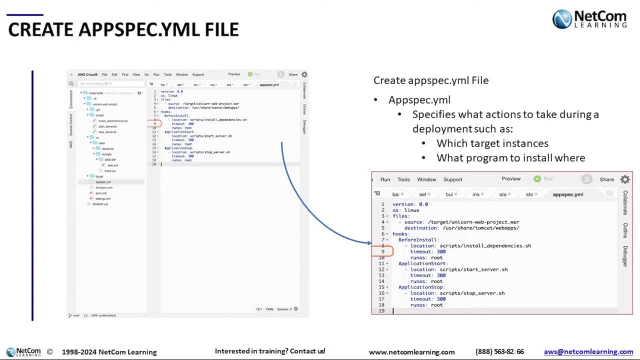 several starting a server, stopping a server type of a script, as well as AppSpec YAML file, And once again I forgot to commit and push. So I'm putting in here: you have to commit and build right, That is to push it. 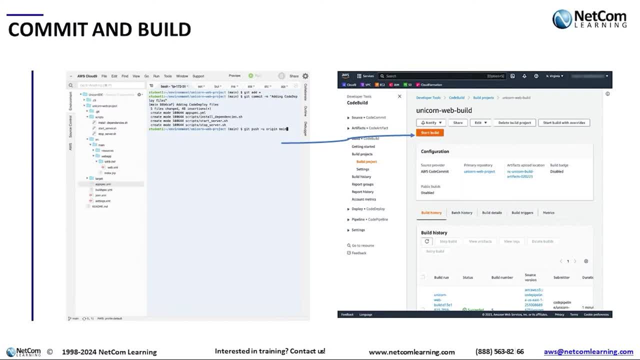 And once you you know, because I've added some files here, right? So you know, AppSpec YAML file is an addition to that. I'm still in Cloud9 working on it, So I have to commit that and push it to CodeCommand okay. 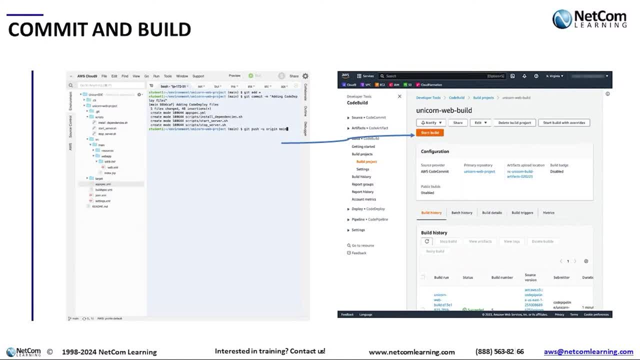 And that is gonna be used to. once again, you have to build it too, right? Okay, yes, we are in the deploy stage, but the deploy will take what was built previously, right, And because I've added the file to the source. 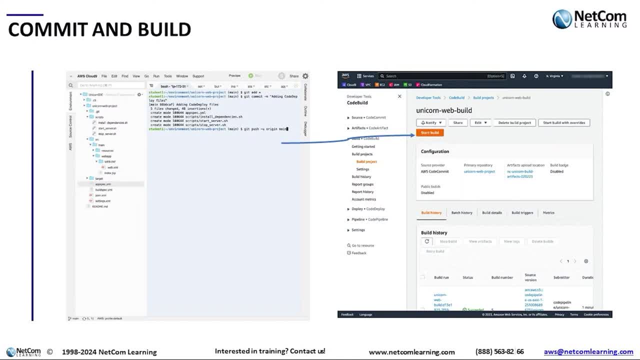 now I have to go ahead and commit, push, then build, so that now I have a brand new zip file with those brand new files in there, So that the code deploy can go ahead and take that and deploy it. So remember right to do all those things. 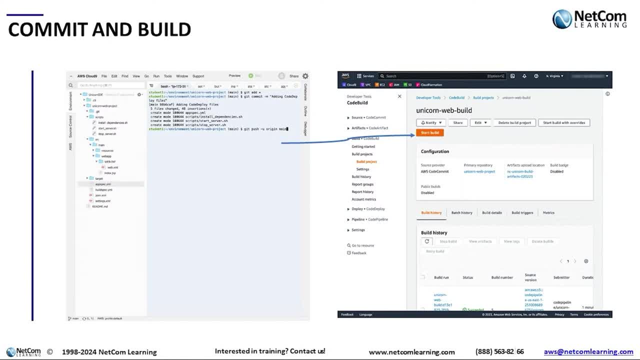 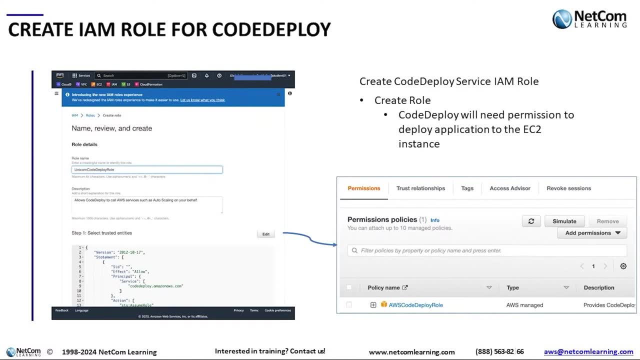 So that's why I have a screen here for you: Commit, push and then build. okay, Still manual, but that's fine. Now CodeDeploy, right, needs permissions. Yes, right, Because what's CodeDeploy doing? 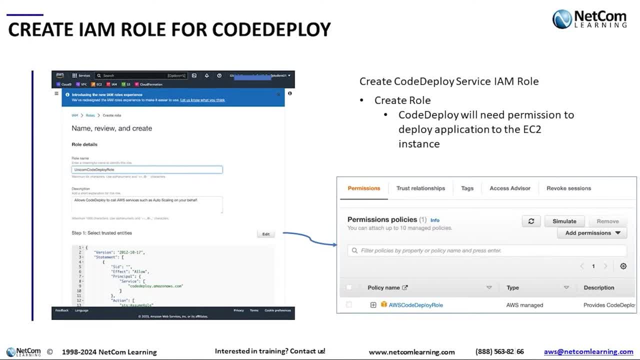 Well, it's gonna access it, right, It's an EC2, and it's going to be installing stuff. Well, that's kind of scary, right. So you want to make sure that you know CodeDeploy actually do, indeed are permitted to do that. 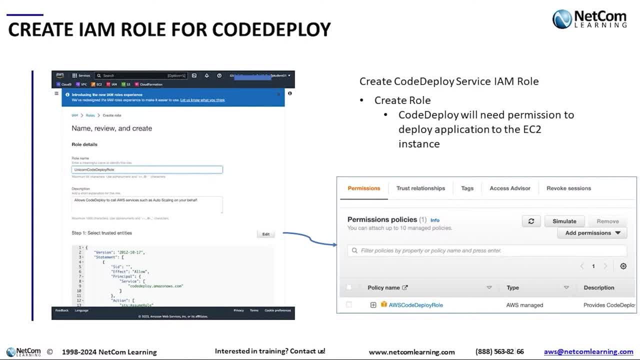 and you do that by creating a IAM role, right for CodeDeploy, right? So we're gonna be creating a CodeDeploy service IAM role and you know it's gonna be assigned to CodeDeploy. okay, As simple as that, yeah. 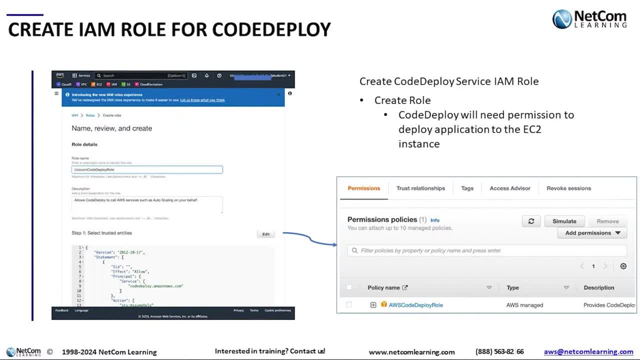 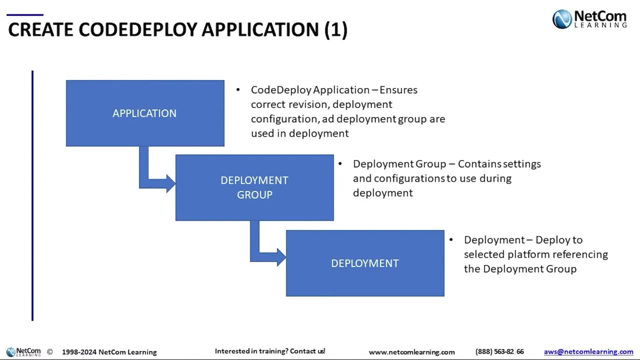 Now when we do deploy, it's a little bit more, a little involved. at least the user interface part is a little bit involved in the code I would say build. So I've kind of broken out a slide for you here. 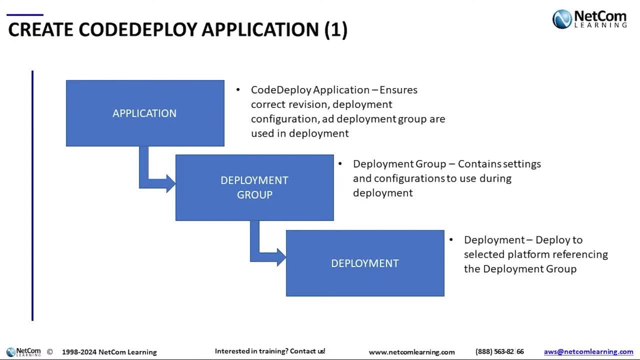 So initially you have to create something called the CodeDeploy application, right, So right at the top on the left-hand side, right CodeDeploy application. So it allows to make sure that you have this you know nice package that says you know. 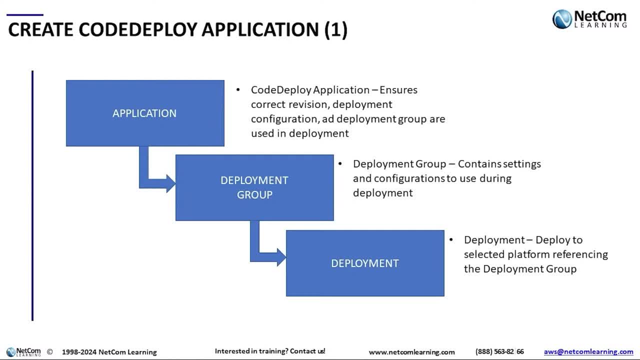 unicorn application deployment and it's gonna have all the configuration, all the deployment information. that's all in one place That you know you don't misplace. Then, inside that application that you create, you have to specify something called a deployment group. 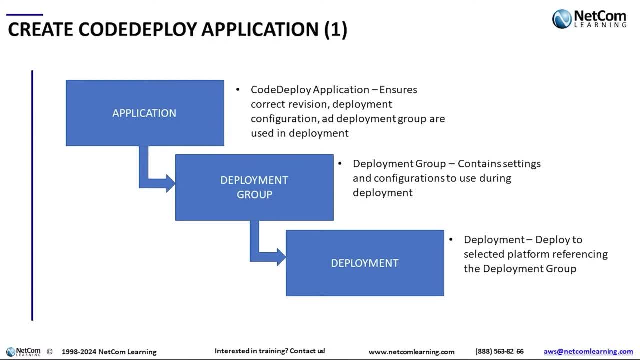 okay. So here deployment group contains settings, configuration during deployment right And then within the deployment group you can do multiple deployments. So here I'm gonna be creating one deployment deploys to select the platform EC2 in our case. 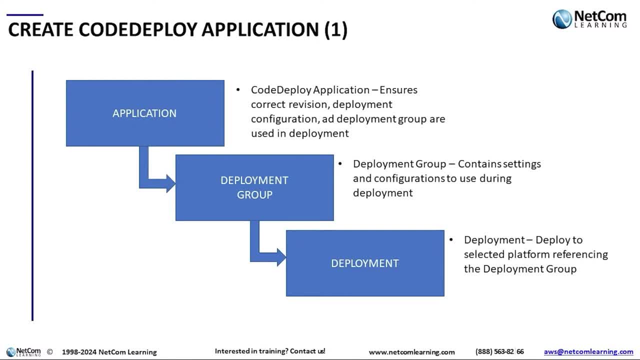 that is specified in the deployment group. So that's kind of. this is how they all kind of relate together. You know settings, okay, But no worries, right, When you are setting it up using CodeDeploy, it's going to guide you through one by one in that order. 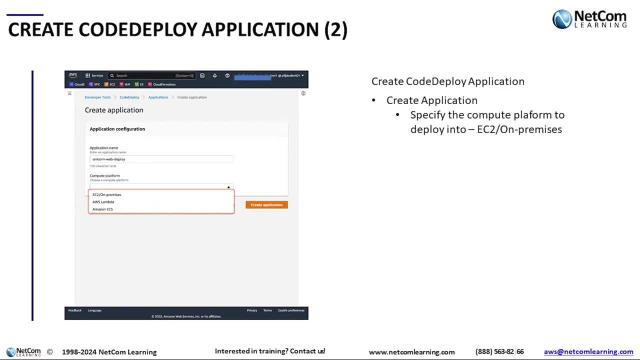 So here I'm gonna create a CodeDeploy application. I created, you know, unicorn web deploy application there, okay, And that's all there is right there. So, and then you have to specify: okay, so is it in containers? 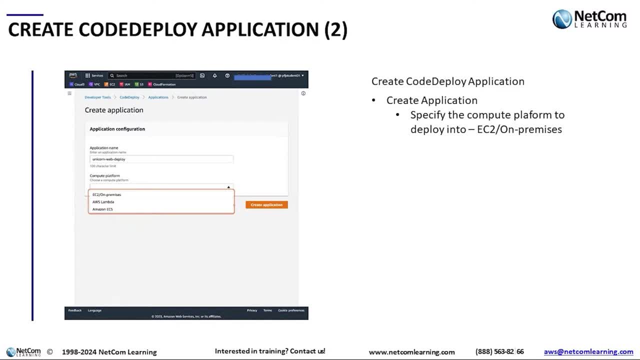 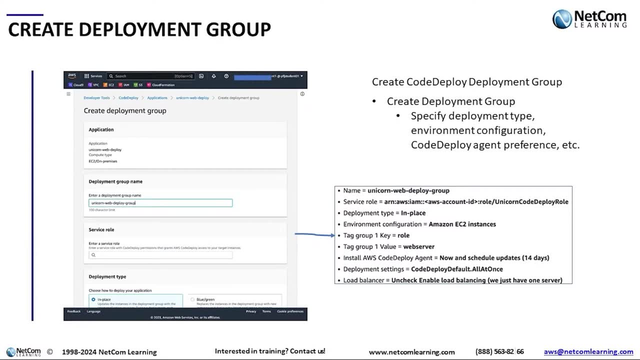 Is it in EC2?? So I select EC2. on-premises: Yeah, you can actually install stuff in on-premises too, If you are able to install a CodeDeploy agent inside your on-premises server, for example. 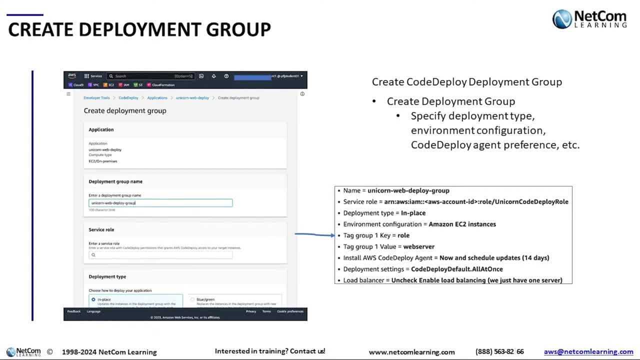 Yeah, just on the side. Then the next thing: once you create the application, it's gonna say: hey, you know, you wanna create a deployment group. Say yeah, So you know creating deployment group. specify deployment type. 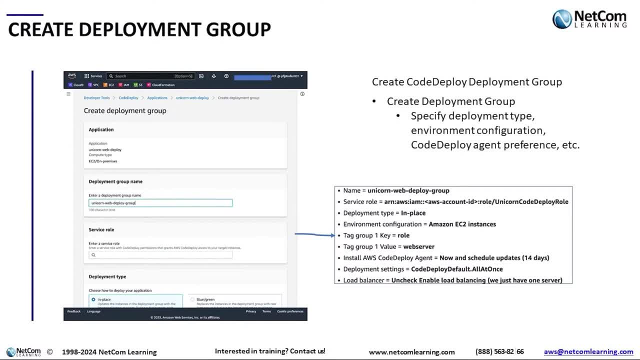 That is, is it in-place deployment, Is it blue-green deployment? Remember, I told you right, Those two different types of deployment strategies: Environment configuration. you know what is the rule, you know, and so you'll see right on the details. 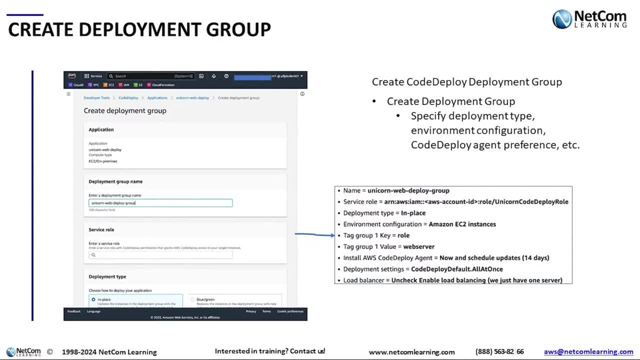 on the lower right-hand side. okay, So those are some of the questions that you have to add in there. If you wanna tag something, do you want a load balancer? So in our case, we're not gonna have load balancer. 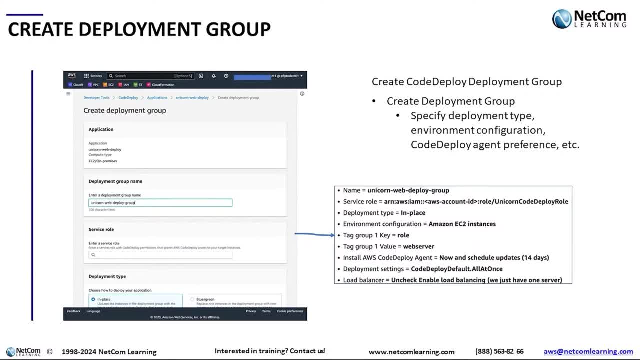 because we only have one server, right. But that's basically what you specify Anyway. so agent preferences. By the way, agent can be installed automatically for you when the CodeDeploy is initiated. The CodeDeploy is initially trying to contact the server. 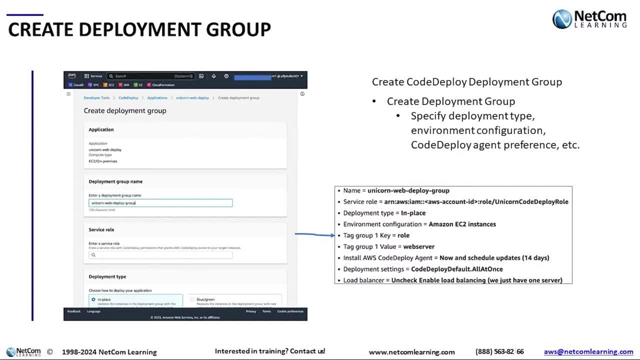 But in order to do that, the server has to be ready to accept that command to have the agent installed. So, but that I didn't actually have any problems with the Amazon Linux 2 that we're using on the EC2.. All right then. so next one here. 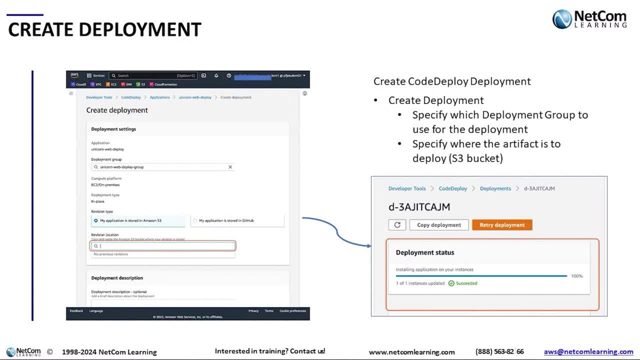 Now we're gonna create a deployment. Yeah, we're getting pretty close to the end here. So create deployment, specify which deployment group you're going to be using, And then from that place you can just click on, say deploy- All right, or you could do multiple deploy. 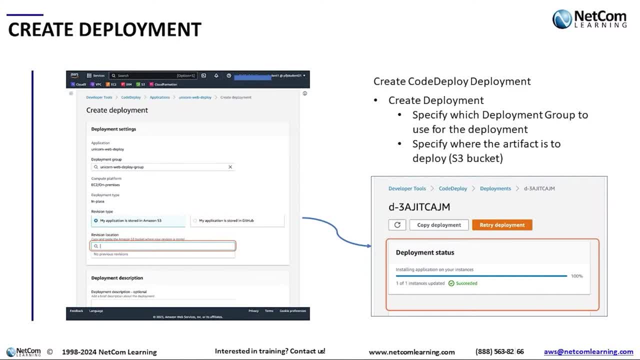 So you see on the right hand side the orange button that says retry deployment. Yeah, you just go in and take that deployment and, like, redeploy it if you wanted to. And once again, you know there are two ways that you can check whether your deployment succeeded. 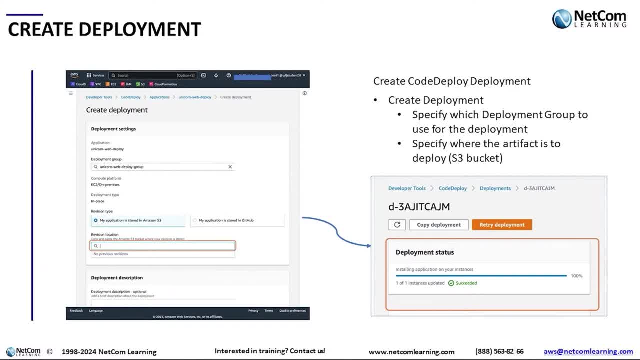 One visually. as you see there it says succeeded: 101 instances updated. succeed. Wow, great, okay, But how do you know it's really succeeded? Yeah right, once again, proof is in the pudding. Go to the website and see if you could see. you know. 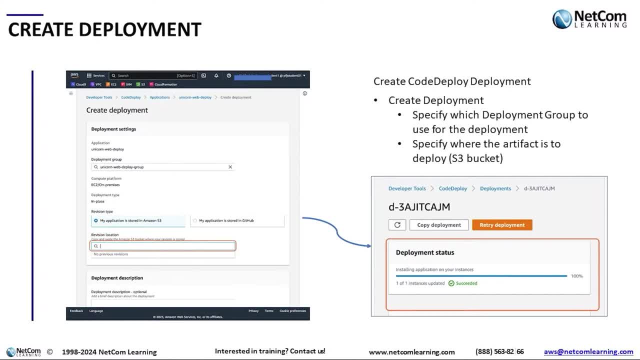 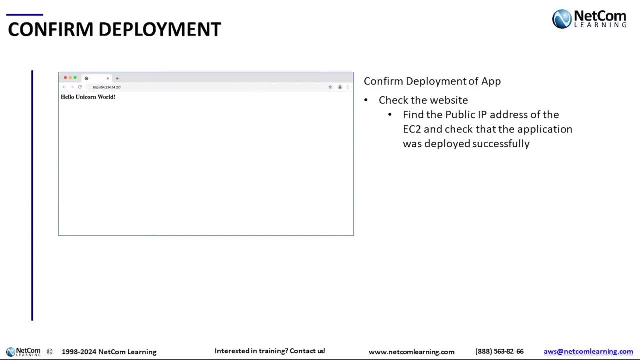 see this wild ride. you know website. So that's what I did. I took that EC2 that they created and there is a public IP address. So I put that in the tab and then, sure enough, not too exciting, but it says: hello Unicorn World. 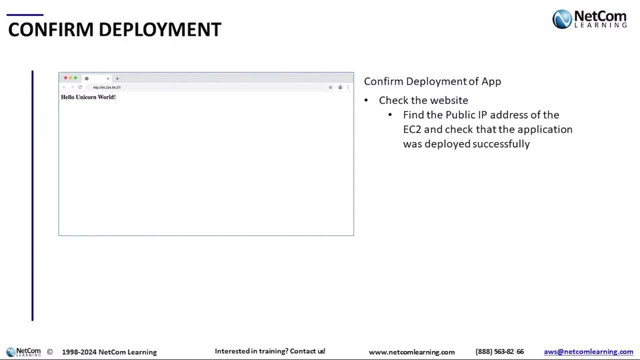 There it is okay. So now my web server is at least beginning right to show you that, hey, it's a Unicorn Wild Ride website. There you go Now. last but not least, let's now automate the whole thing. 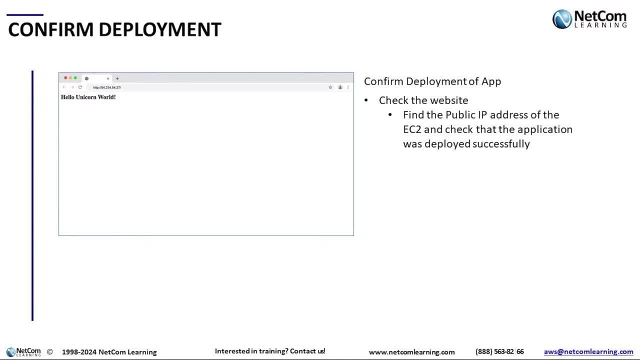 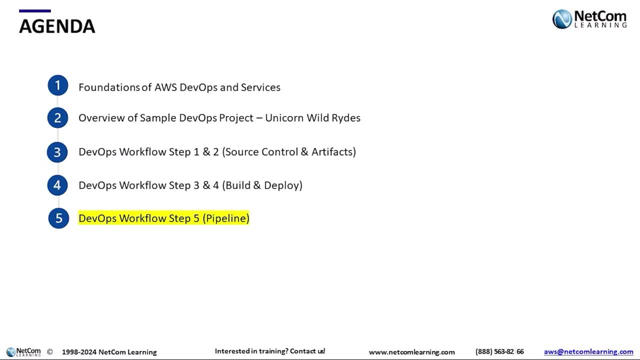 Now we know the integration visually. everything's working. Let's put it all together, okay. So here we're going to be working on the DevOps workflow, step five, which is the cold pipeline- okay, By the way, whenever I explain cold pipeline, okay. 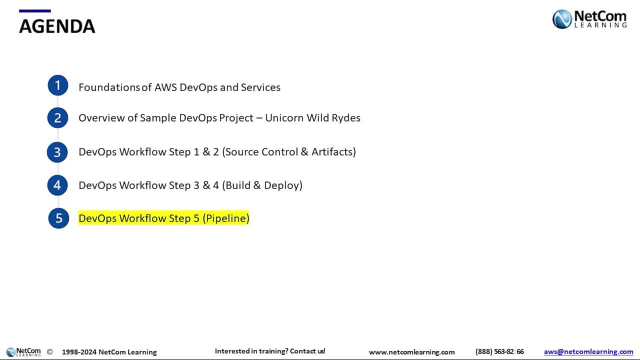 in my other courses. I kind of explain it like an oil pipeline. okay, So we have an oil pipeline. you have a physical structure which looks like a pipe, a humongous pipe, and then you have an oil that's flowed through it. okay, 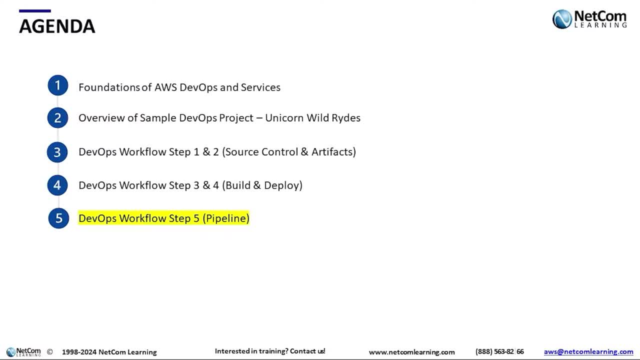 So cold pipeline is like that. Cold pipeline is an infrastructure. It's a logical virtual infrastructure and your program runs through it. okay, And the cold pipeline is what helps move it forward. right? It says: oh, you got it on source. 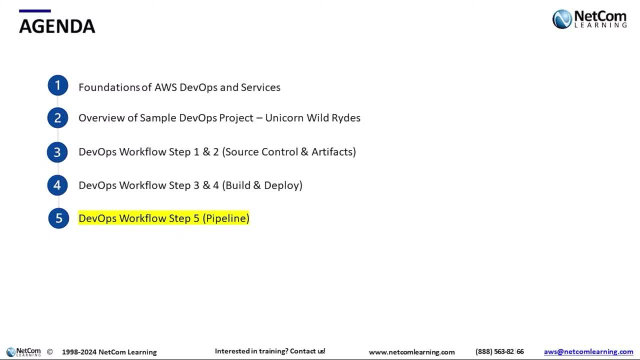 Boom, let's move it to. you know, cold build, Boom, now it's done building, Let's move the next process to cold deploy. Oh great, now it's all over, right, So it helps to move things forward. 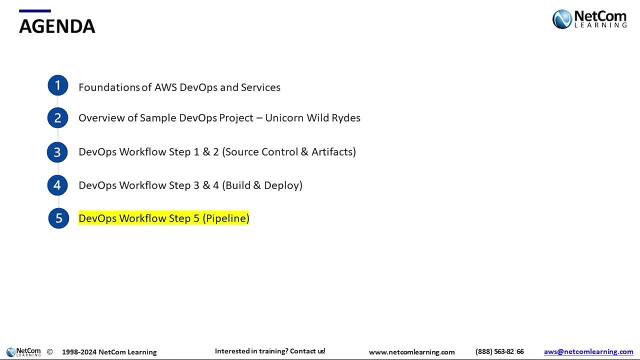 And you know if there's a hiccup somewhere, it's cold pipeline- actually have a way to, you know, to contact the developer and say, hey, you know there was a major problem here, so please go ahead and fix it, type of stuff. 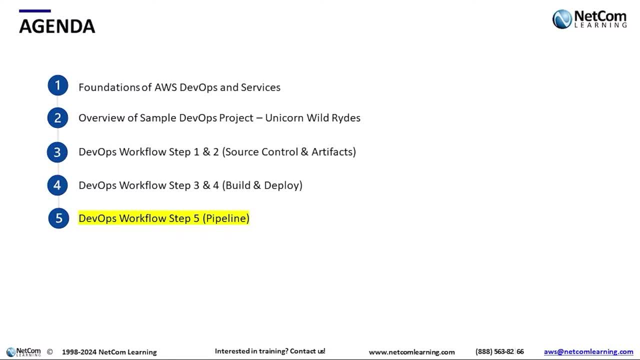 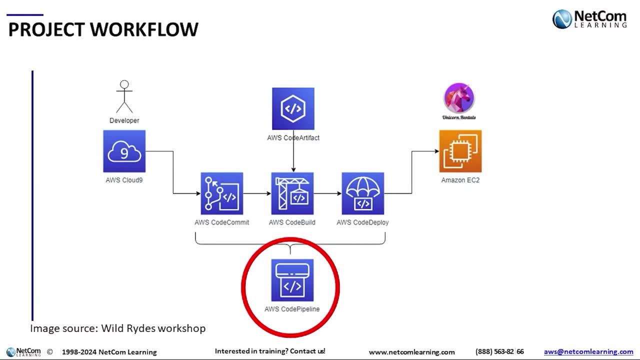 So it has a nice feature to orchestrate things like that. Okay, So from the workflow perspective, that's where we're at right now. We got the individual parts, now it's time to put it together. So cold pipeline is known as a orchestrator, right? 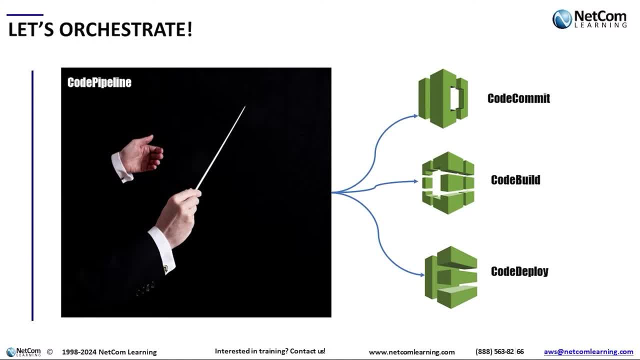 It's an orchestrator, So it's going to orchestrate, cold commit, cold build and cold deploy all together. So that's the job, okay. Now, because it's a pipeline, it's going to look like a little pipe, okay. 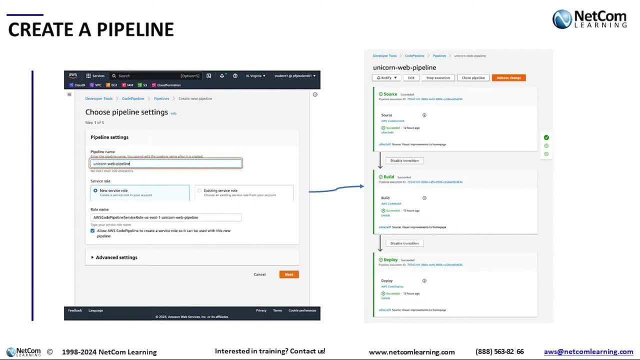 So if you see, on the right hand side there I've created three stages, okay, in a cold pipeline And it's very visually very pleasing. You know, it's almost like, yeah, I'm creating a pipeline here, okay. 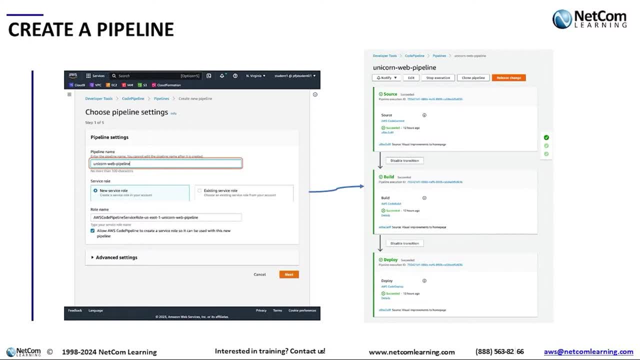 So the first phase is the source phase, The second phase is the build phase- right, And the third one is a deploy phase- right. So you can see they're kind of all green okay, Because as soon as you finish creating the pipeline, 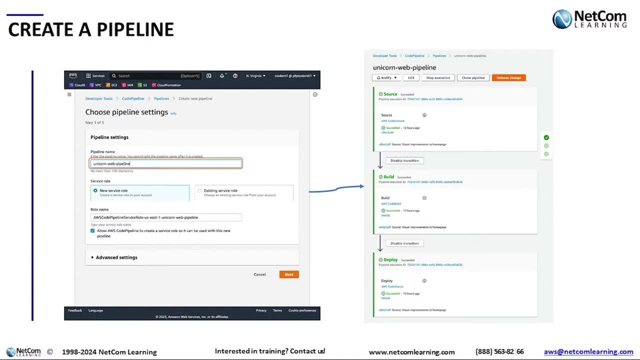 it's going to run, I know right, Okay And but I don't have anything new, but that's okay. Cold pipeline says that's okay, I'm just going to run this thing And you have to make sure when you create the 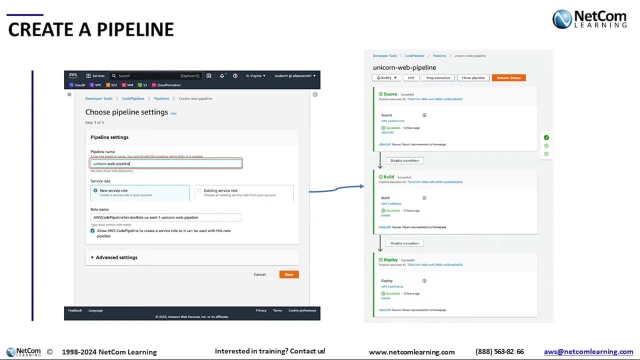 each of the pipeline components. that all you're doing is you're pointing to the stuff that you've already checked. So the source, I'm pointing to cold commit On the build stage, I'm pointing to cold build stuff. You know, remember the project that I created, right? 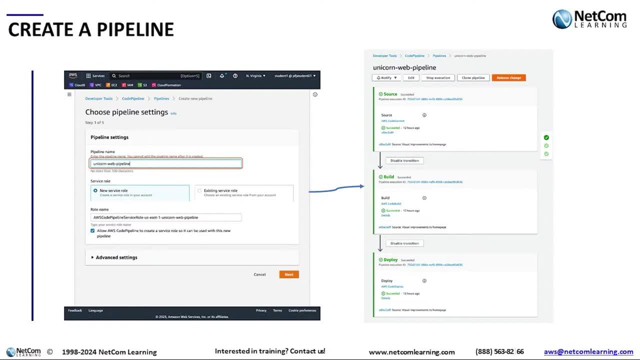 Using build spec YAML file. And then, on the deploy, I'm just pointing to the application. Remember the deployment application that I created with the app spec YAML file. That's all I'm doing, right? So then it ran okay. So now, what are we going to do is okay. 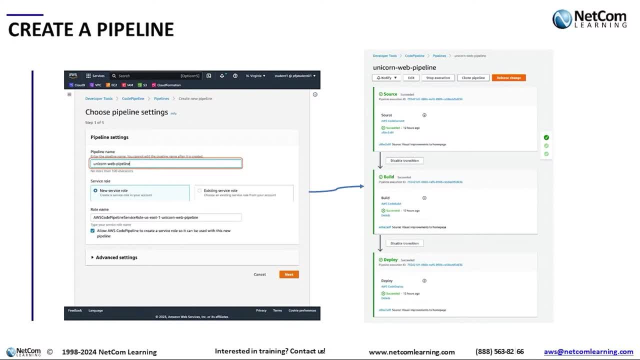 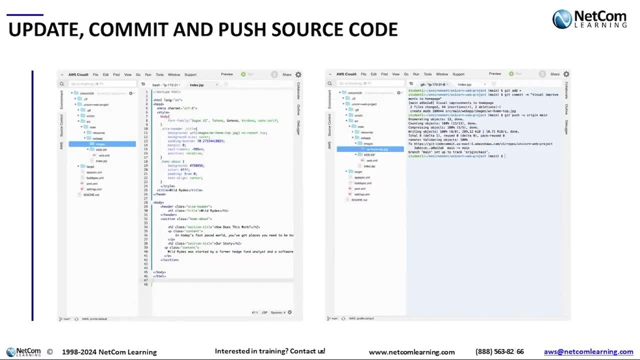 So you saw that website. you know it wasn't too exciting. So now we're going to make it into the very colorful, the real stuff. So I'm going to make changes in my Cloud9 into the indexjsp file, right? 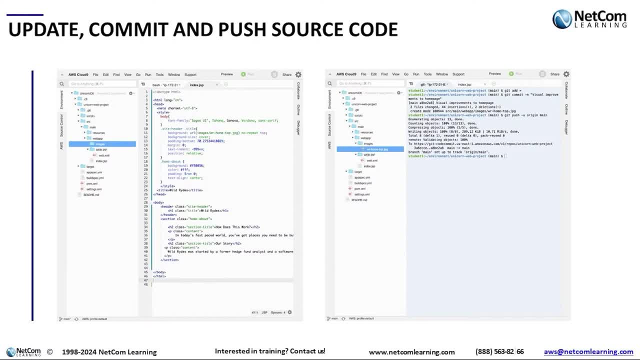 So then you know, then I'm going to commit, push okay. What happens now is this: When I commit and push okay, The cold pipeline says: oh hey, there's something new in the cold commit, I have to move it forward to. you know, cold build. 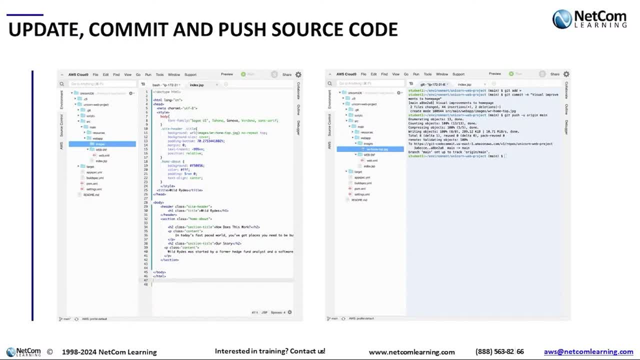 Boom. And then next it goes cold build. When it's done, that's done, It says, oh, I'm going to have to move it over to cold deploy. And once that's done, it says, okay, I'm all done. 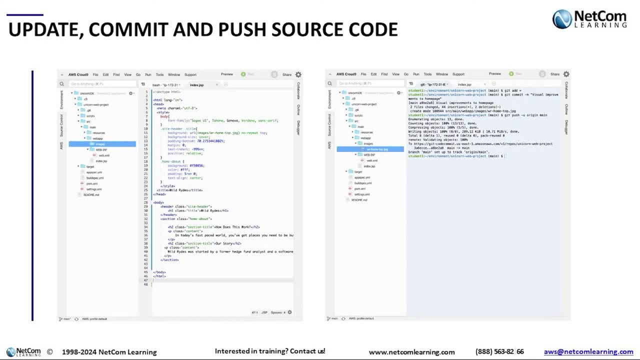 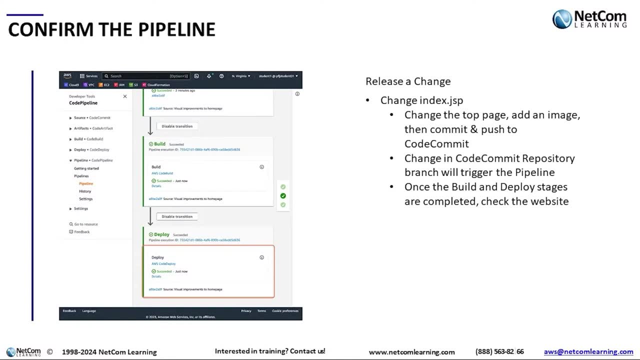 That's what's going to happen. This is the beauty of the automation. okay, So here I'm checking to see, confirming the pipeline. okay, So I quickly, right, As soon as I commit and push, I quickly go to cold pipeline, because I, you know, 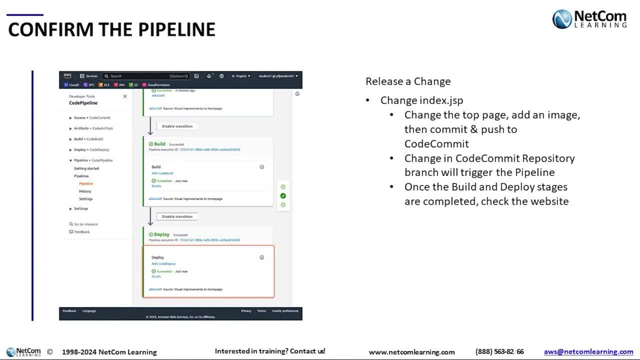 I'm kind of I'm pretty excited about you know whether, if everything's going to work okay, Then you can see visually as it goes through the pipeline it says: okay, I'm working on the source right now, Good to go. 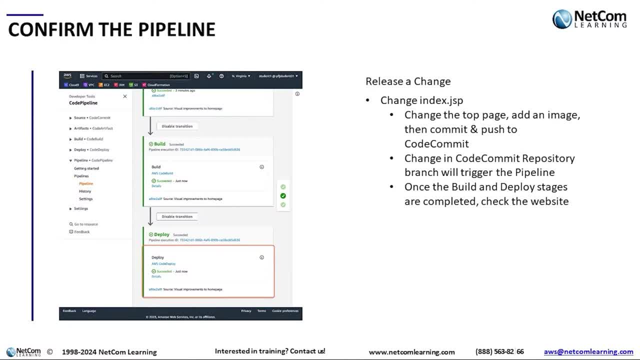 I'm working on the cold build right now- Good to go. I'm going to go to cold deploy right now- Good to go, Okay. So this is an example where I was kind of like watching it and everything deployed okay. But once again, right. 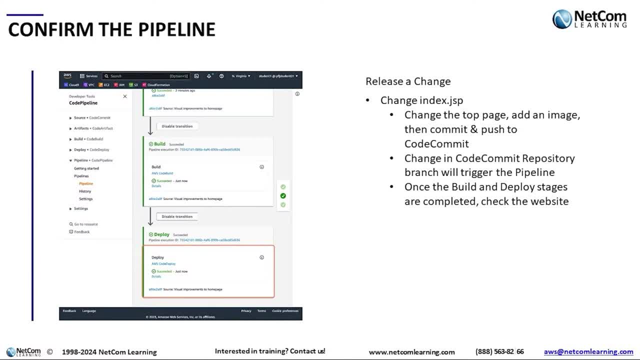 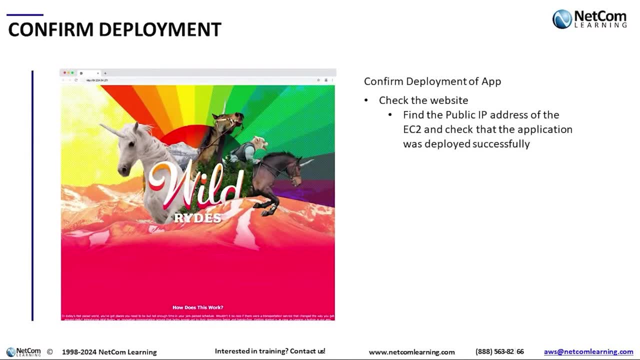 Now I'm going to go back to my website and I'm going to refresh the screen, Okay. So let's see what happened. Okay, And this is basically what happened. Yeah, Brand new. Oh, by the way, I had to upload an image too, right? 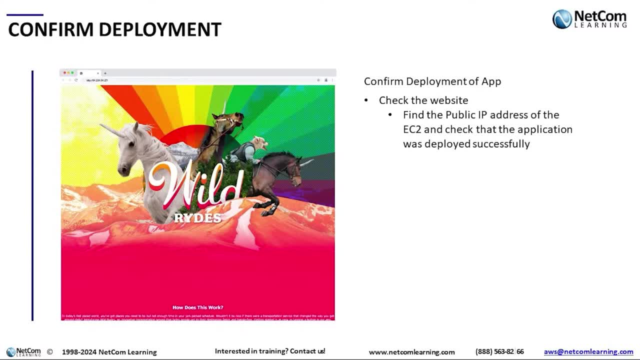 So the image was inside the. you know everything was committed and pushed and built and stuff. So there you go And it feels so good right After you work all these components and once you automate it. Now, if I made other changes, it's going to reflect. 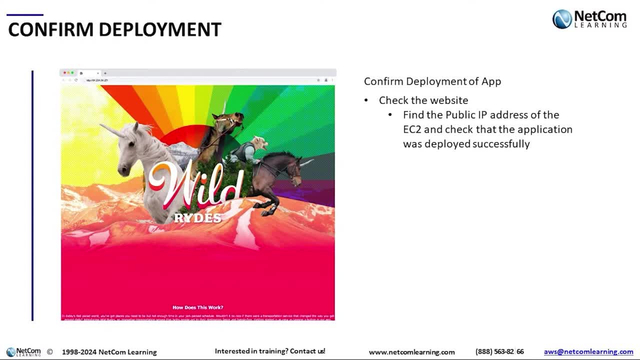 The whole process. it took maybe about- I don't know, maybe about six, seven minutes. Okay, Because, remember, you know, nothing is really instantaneous, because the there are some times that you have to kind of take into account right. 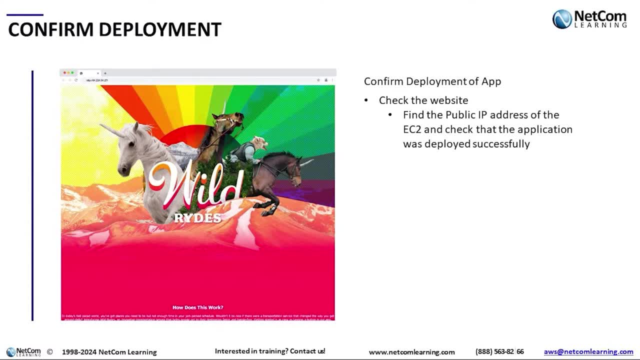 Because as soon as you commit to co-commit, there's going to be some time- not a long time, you know, probably, like you know, not even a minute- but for the cold pipeline to realize: oh, there's something new. 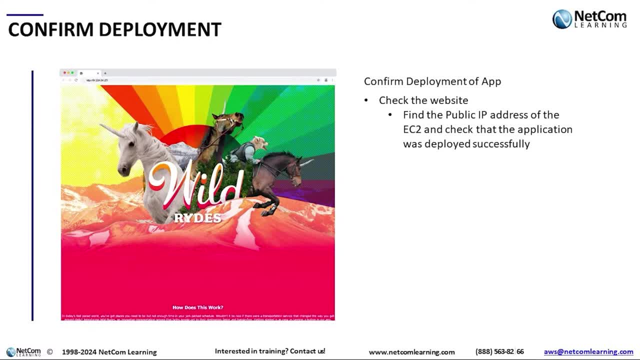 Then remember the cold build. it took like five minutes, Okay, And cold deploy also took, like I think it took like three, two, three minutes. I don't quite remember how long it took, So you have to put those all together. 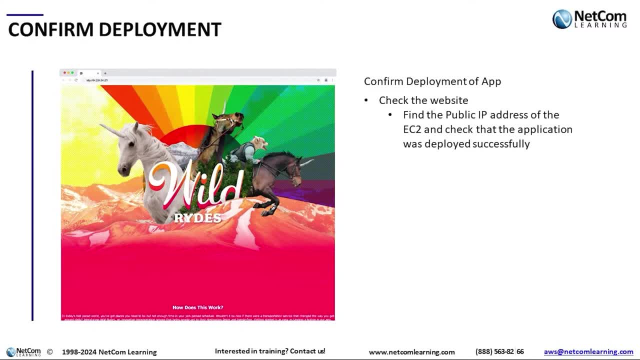 So, but it's automated, right, And you know I could have done this like all day, everything right. So every every hour I could be making changes and you know every hour there'll be like changes on the website. 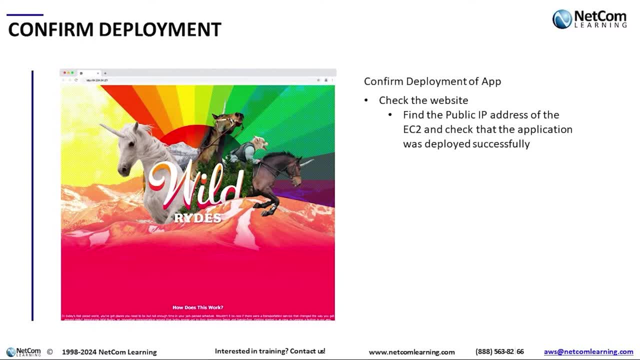 Anyway. so I hope you you enjoyed that walkthrough to actually see the, the AWS, various DevOps tools in action. Okay, And that's basically what I have for you. Okay, And, as I mentioned, you know, try it out, right. 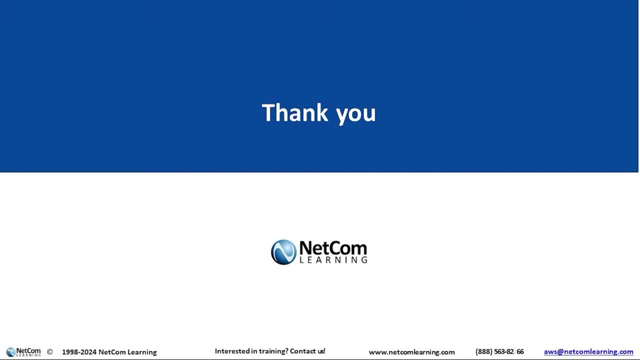 So if you, you would need your own AWS account to do this, but the instructions are pretty clear about that. Okay, All right, So now that I'm finished with my the main content part, I'll be open to answering any questions that you may have. 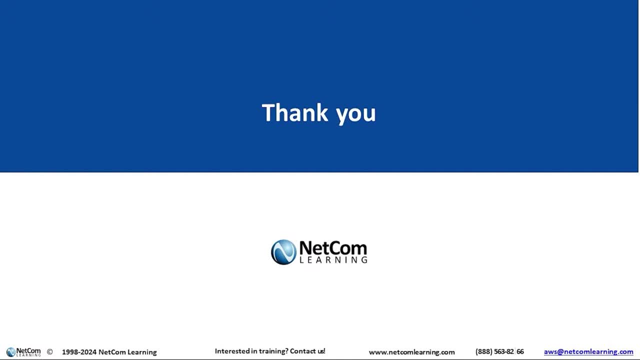 Thank you, Tarumi. That was very informative. I know everyone is looking at it, Looking forward to the Q and A session, So go ahead and start putting your questions into the questions panel. And now I'd like to give the presentation rights over to. 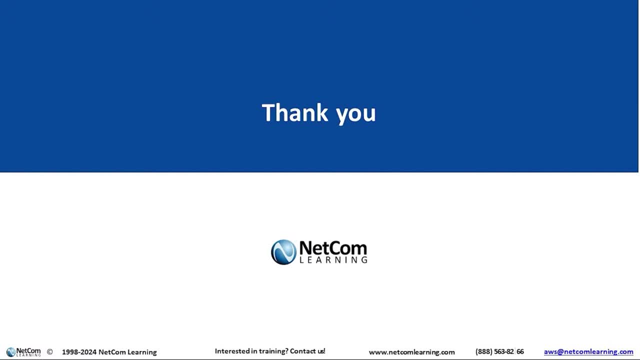 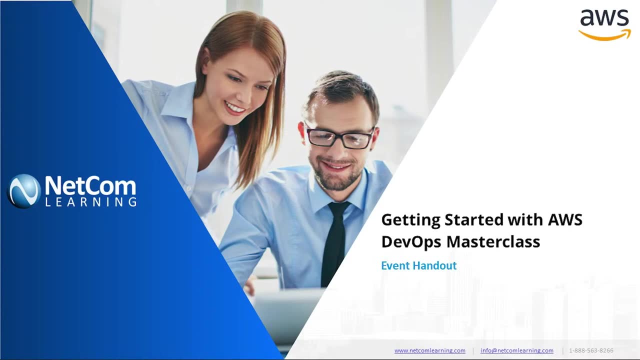 Remy, our vendor manager, to introduce our promotions and webinar related courses. Thank you, Tracey, And thank you, Tarumi, for this insightful session. I believe everyone must have learned something new today or would have been able to brush up their skills around the 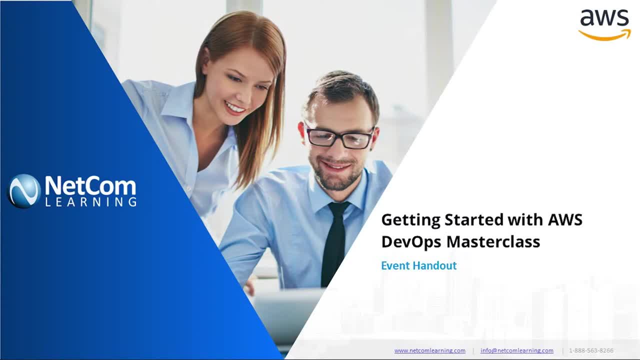 fundamentals of AWS cloud. I would quickly like to take you through some of our handpicked resources which we think will immensely help in accelerating your AWS cloud scaling journey. Well, this document here I've I've sharing on my screen. This has been shared with you all. 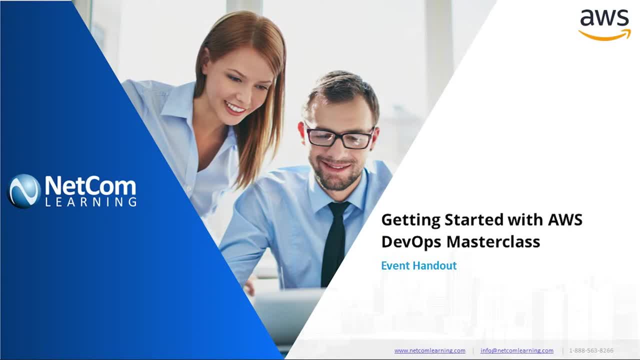 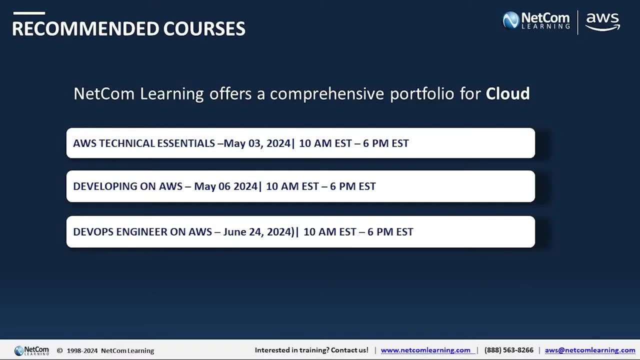 in the handout section of GoToWebinarPanel, You can download this document and access all the resources and browse all the offerings we have curated for you. So first step here is the list of our recommended courses, which we found again. this is the list on the right. 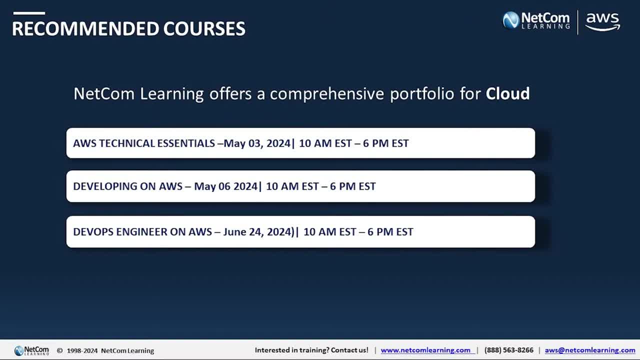 It's free. It's free to use it feel will best suit your learning journey after attending our masterclass. All these courses are hyperlinked. Feel free to go through them post-event and check out the course descriptions, prerequisites and the value it can add to you and your team's skill sets. Additionally, we have 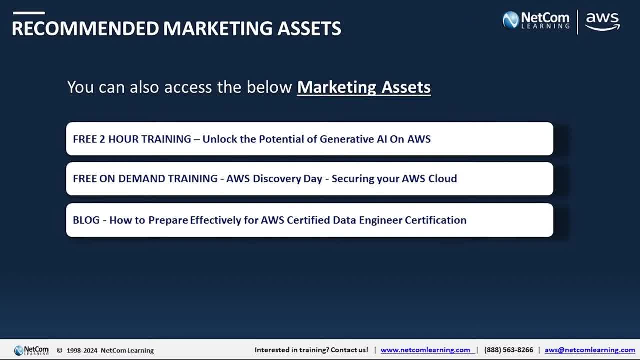 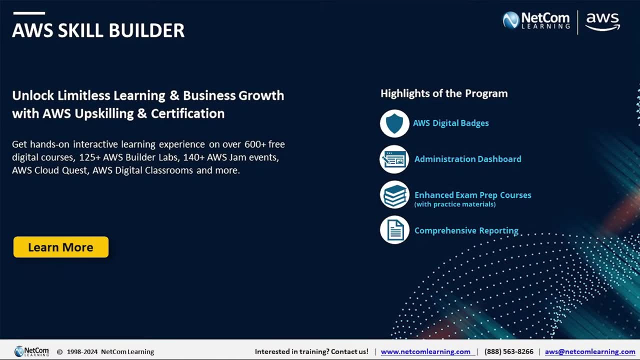 curated a blend of resources, including our upcoming and on-demand events, as well as informative and educational blogs. You can make the most of these resources to gain extensive knowledge on the AWS topics they cover. Next up, I am thrilled to introduce the AWS Skill Builder. 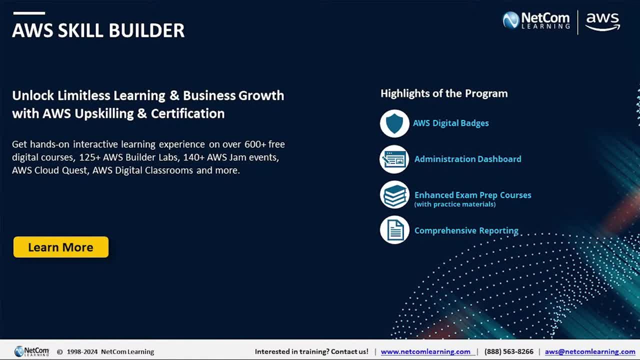 a dynamic learning center featuring over 600 digital courses crafted by AWS experts. I'm sure most of you must be aware of AWS Skill Builder. What is unique about this platform are the engaging game-based learning experiences. So through AWS Cloud Quest and team-based competitions on AWS Jam events- If you're hearing these terms. 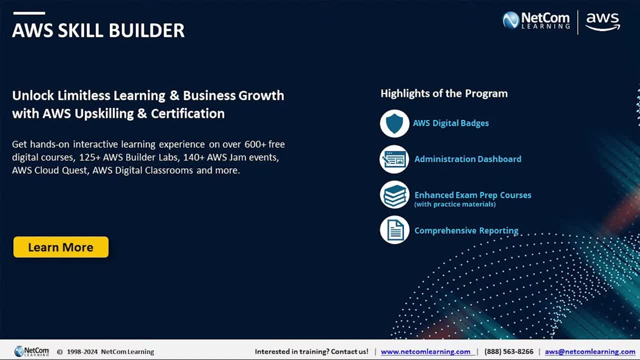 Cloud Quest and Jam events for the first time. I would highly recommend you click on this button and you go to our AWS Skill Builder page. I'm sure you will be amazed to see what all the Skill Builder has to offer. They have set off these gaming experiences in practical real-world. 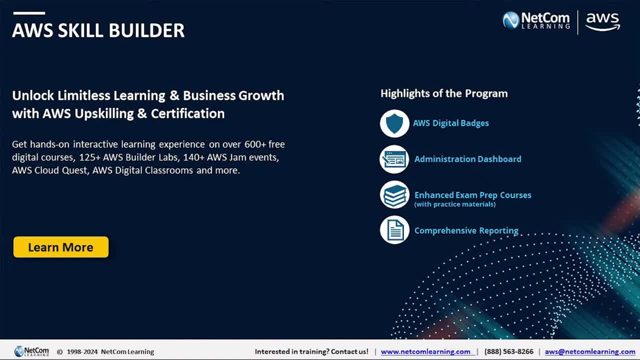 scenarios, which makes it so easy to understand concepts, technology and processes and it makes it so interesting for the learner And for organizations. it saves a lot of time on employee skilling and ultimately enhancing the efficiency and productivity. As someone at Netcom, 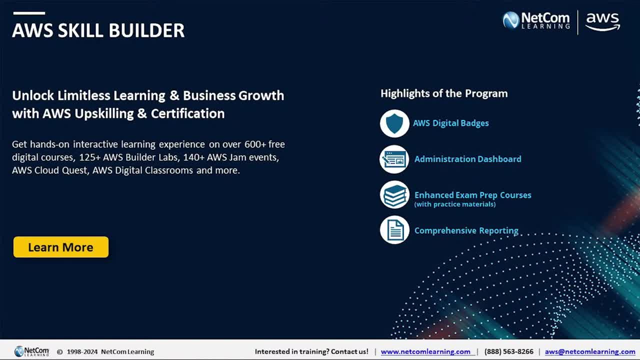 who values continuous learning. I'm confident that AWS Skill Builder will be a game changer for any organization looking to upskill their workforce on AWS technologies. I encourage you to explore the diverse range of digital courses and experiences it offers. You can simply click on the. 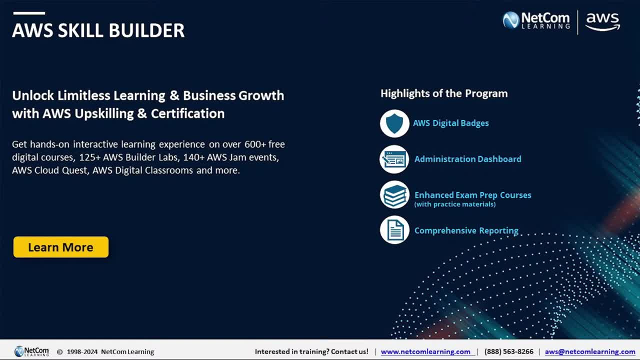 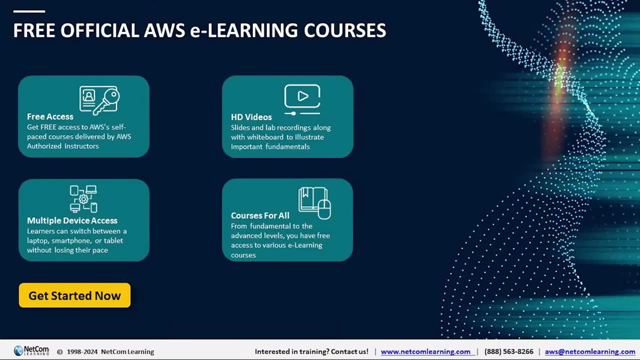 simply, as I said, click on this button right here, learn more, and you can explore more about the skill builder and the pricing aspect of this. Moving on to the next offering, our free AWS e-learning courses follow a self-paced training model wherein you get the liberty of: 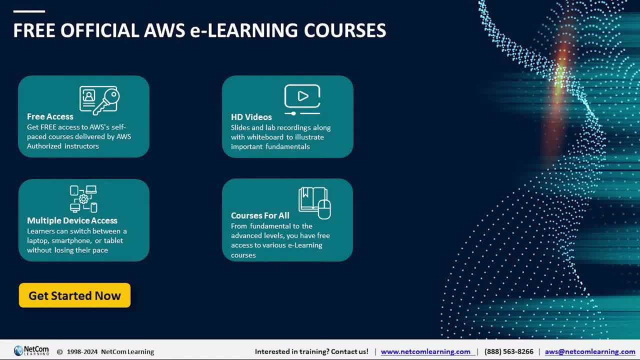 accessing extensive course related videos that are delivered by the AWS subject matter experts on the go. So these videos cover the availability on the device of your choice, so you can access them from your laptop, your tablet or from your phone as well. There are more than 280 videos. 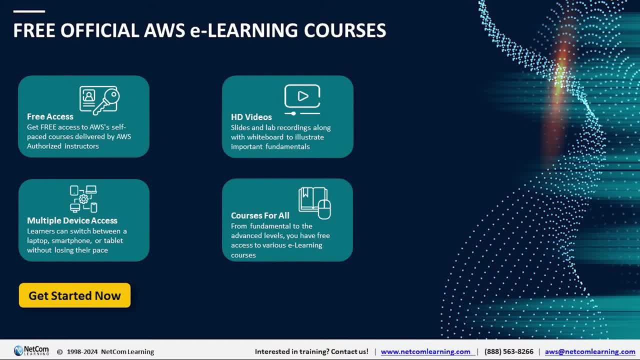 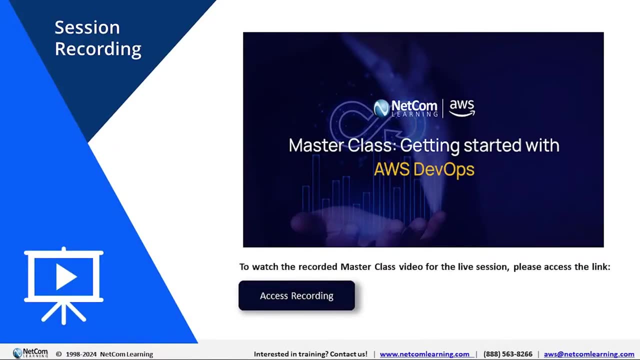 covering various AWS topics, explained in a very easy to comprehend language. You can simply sign up for free, watch these videos and make the most out of them. Also here, I would like to inform you that this session is being recorded, so in case you want to. 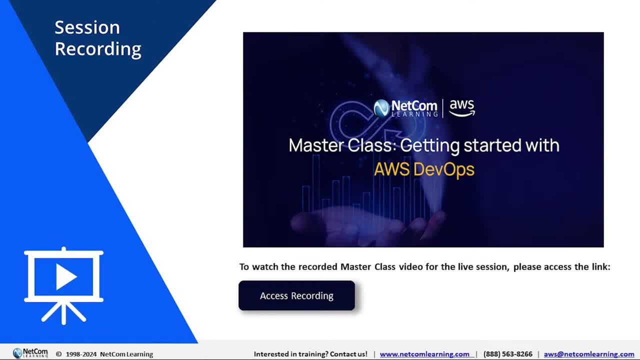 refer back to any of the topics that the trainer might have covered in today's session. we will be sharing the recording link with you through emails and also you can access it here by clicking on this button. So you have to download this handout for that and then if you want to revisit any topic, 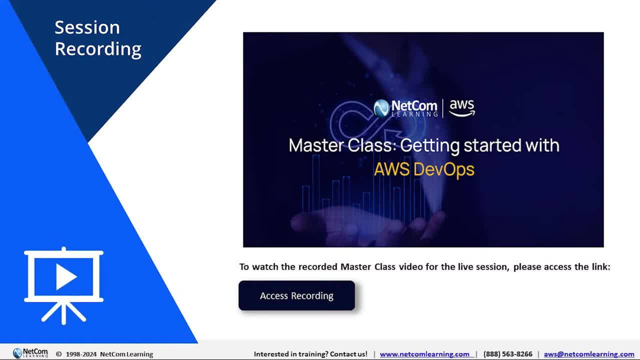 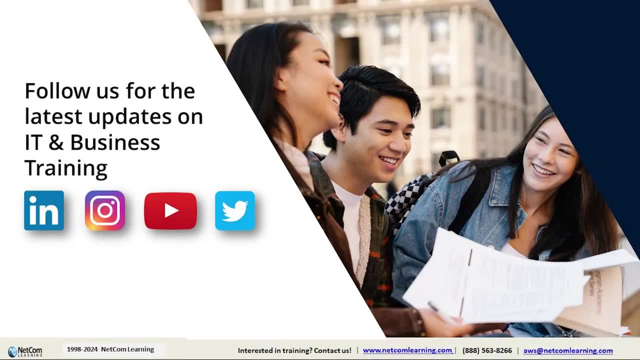 you can just simply click on the access recording and you can access it. You can revisit the session and learn at your own pace. Now, apart from our virtual sessions, you can also catch the relevant updates related to IT and business trainings on our social media handles. so please, 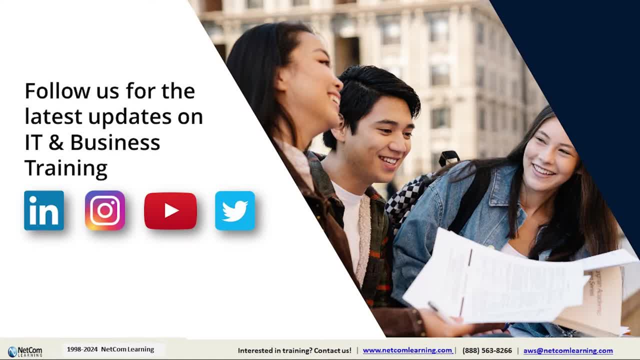 feel free to follow us on LinkedIn, Twitter, Instagram and subscribe to our YouTube channel for all the latest updates. Our official pages and channels are linked here on the icons. Finally, if you have any suggestions regarding the topics you would like to see covered in this session, please feel free to contact us at the link in the description. 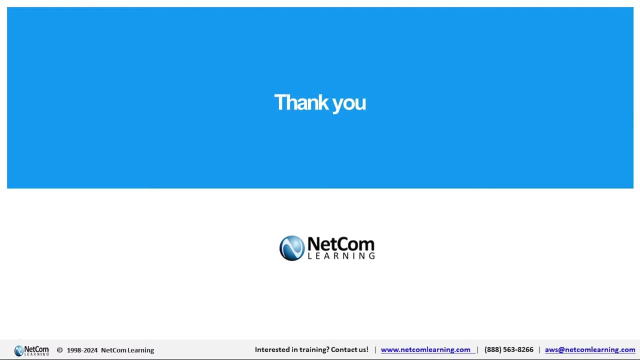 If you have any questions regarding the topics you would like us to cover in our upcoming webinars and masterclasses, please don't hesitate to send us a direct message. or you can leave a comment on our social media posts, or you can just simply email us at info at the rate. netcom learning dot com. 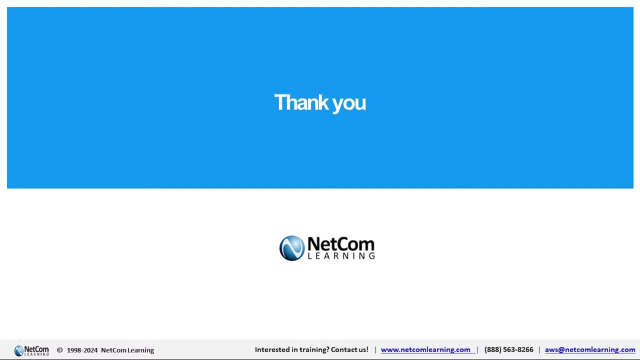 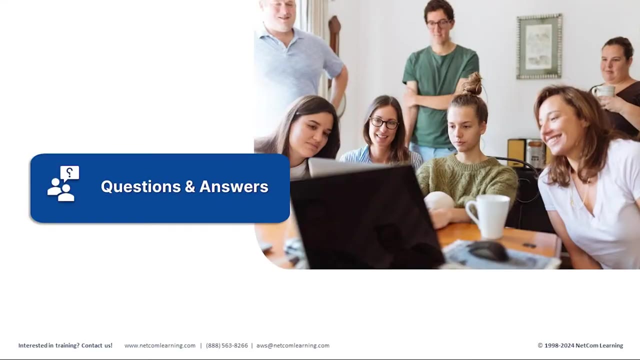 We would definitely try to come up with the sessions on your suggested topics. Thank you once again for joining us today. Over to you, Tracy. Thanks so much for guiding us through that information, Rennie. And now we're going to go ahead and jump right into our question and answer session. 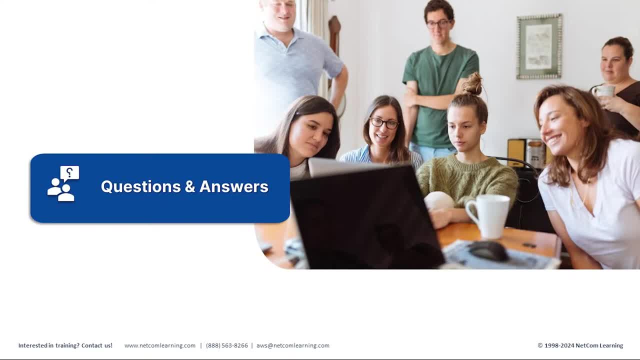 First question we have today is: what's the difference between CloudFormation template and CloudFormation stack? Okay, well, thank you for asking that question, and so, to answer that question, let me go ahead and kind of refer you back to what I mentioned when I was mentioning the infrastructure's code. 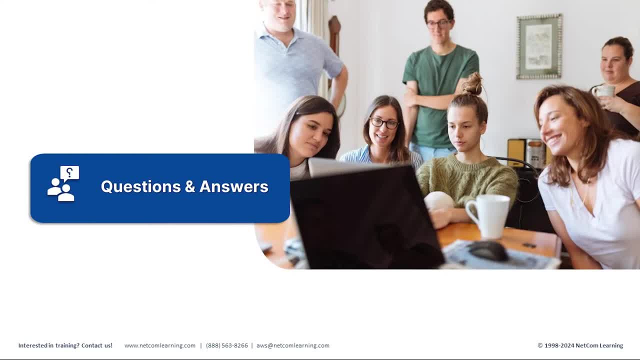 Remember I said that look, infrastructure code is a very important part of the infrastructure. infrastructure code is a very important part of the infrastructure, So it's almost like an application, right? so kind of imagine an application. so in the application when the developers created, they're created inside a source code. 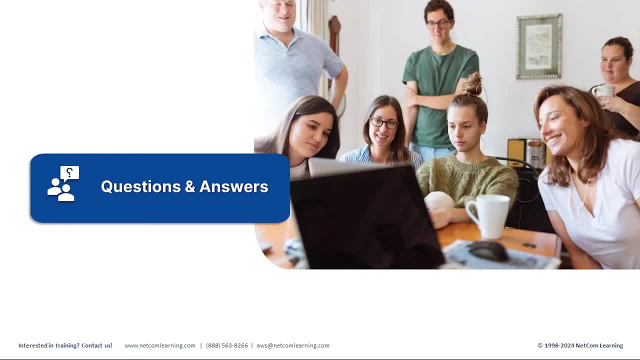 And then that needs to be built right like compiled and stuff, just like we did with the wild rice. then in the end you got an executable or, as I said, the artifact. okay, so with CloudFormation it's just like that. so the source code equivalent Of CloudFormation is the template. so the template. 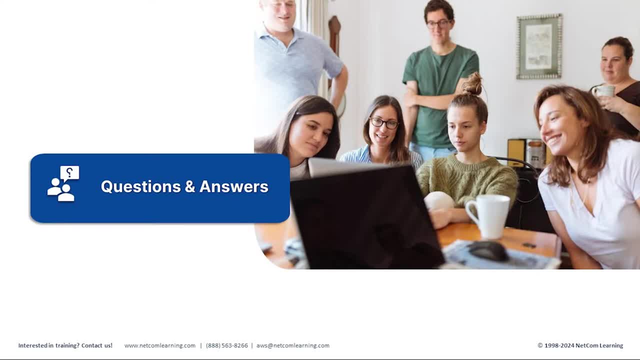 Is in the format either your choice, Jason or Yamo- file, so that's like a source code, okay. and in order for that source code to turn into the network and virtual machines and such, you have to build it, And the application you use to build is the CloudFormation right. so you build your template, which is a source code, right, using CloudFormation, and then the output that you get is: 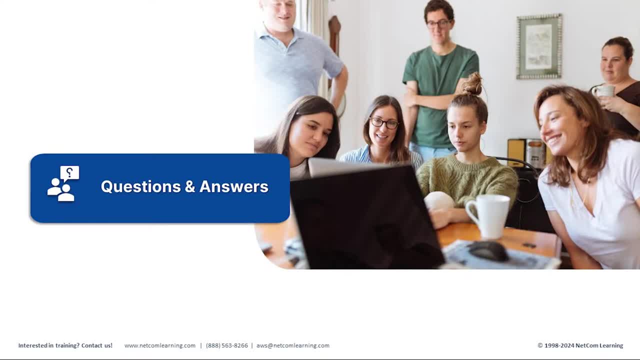 Is all the network and, you know, virtual machines That you wanted to have and that is called the stack. so the stack is a collection of all the resources, like the network, like the virtual machines and anything else that you've actually wanted to actually implement, and that grouping of that together is called a stack. 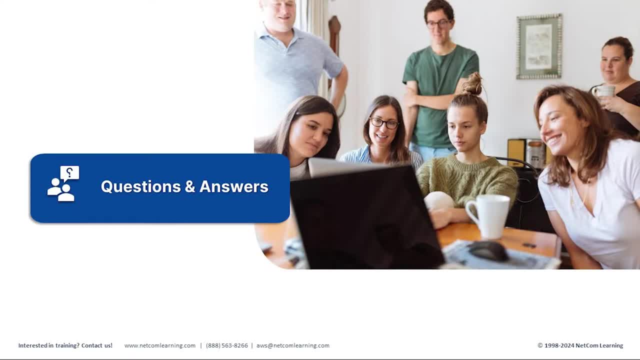 So source code Template, right, the output, the stack. The next question is from Sean and he's asking: can we use CloudFormation template to deploy resources to another region and another AWS account? Yeah, so that's a good question, right? so CloudFormation is very, very convenient, isn't it so? for examples, the CloudFormation template that we used in this webinar: it created the virtual machine, it created, you know, the EC2 instances and all the 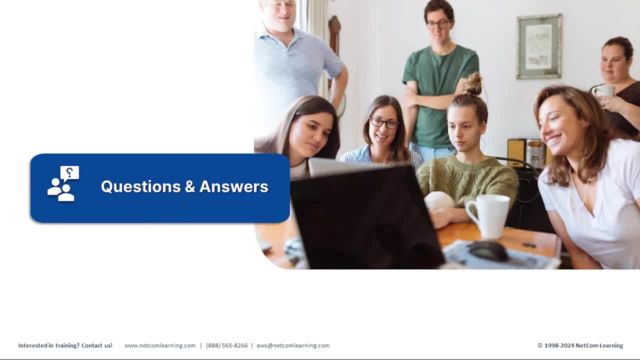 The in the virtual network is what I would say: let's create the virtual network. it created the virtual machine and everything we needed to run this wild rice you know website And in the tutorial, I deployed it in North Virginia. but what if I wanted to deploy that in Oregon? well, what if I want to deploy in Tokyo? but if I want to deploy in India, right, can I do that? right? so these are different regions and the answer is yes, with a caveat: okay. 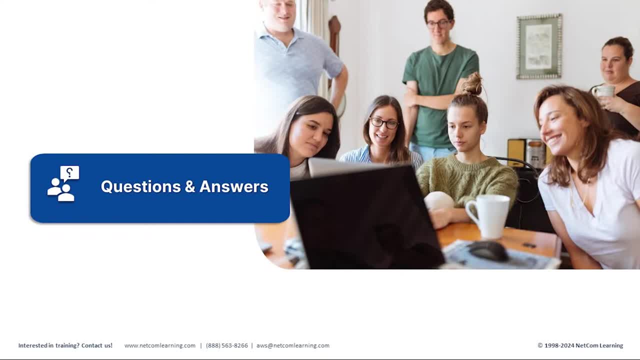 So the caveat means that there are certain things that must be true for these CloudFormation templates to work properly to create the stacks in those regions. so It will depend it's case by case depending upon what type of resources that you're trying to deploy. but take, for example, something like an EC2 server, right? so EC2 server requires an image called AMI, Amazon machine image. 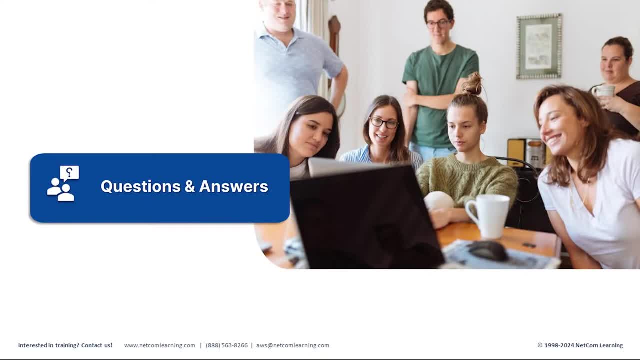 And Amazon machine image is going to have all the software that you need, you know, to Have this web server running, But that AMI image, Or Amazon machine image, is tied or anchored or locked into a particular region. so I need to make sure, though, that, before I run this CloudFormation template in a different region, that the there is a proper AMI available, so that, when the CloudFormation, it's time for it to refer to an AMI. 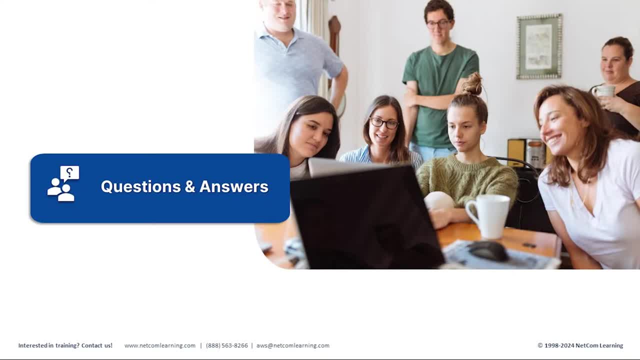 In that let's say in Oregon that there is A image in Oregon that CloudFormation can find okay, so so that would be. there will be some cautions that you have to to pay attention to. there are tools called task cat that you can try your CloudFormation template in various regions before you actually 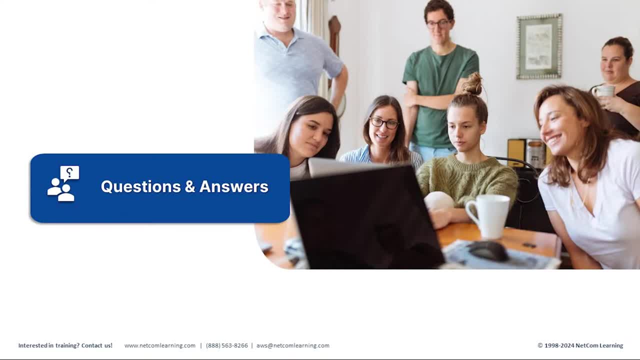 Release that to the you know to people and say, hey, go ahead and use it and you know you probably don't want people coming back with all kind of compliances that didn't work on the Oregon right, so make sure that you know you test it first. so the answer to 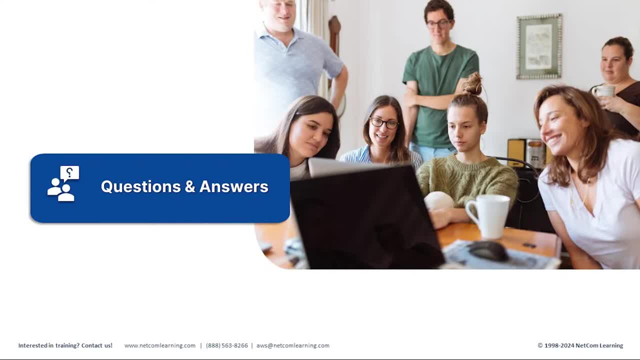 Would it run on other regions? the answer is yes, but you have to be careful of these certain details. now the second part of the question is: would it run on other accounts? and the answer is yes, but once again with the, with some caveat, right. So if you are a company that has multiple accounts, normally what you would do is you would manage that under one big umbrella called the organization. so within the organization, let's say you have like 10 accounts. 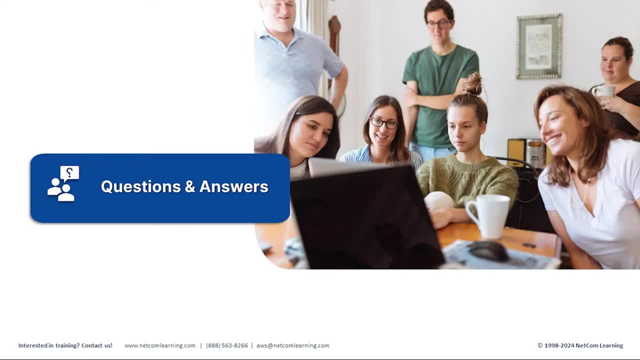 And if you have one CloudFormation template that you actually want to run on all these 10 accounts, there's something called stack set that you can create. so from one location, using one template, you can deploy into many accounts, Obviously you have to have permission right in those other accounts to deploy those resources like web servers. let's say you want to run, you want to actually deploy wild rides right to 10 accounts. well, you know, you don't want to be. you know, obviously you're not going to be able to. 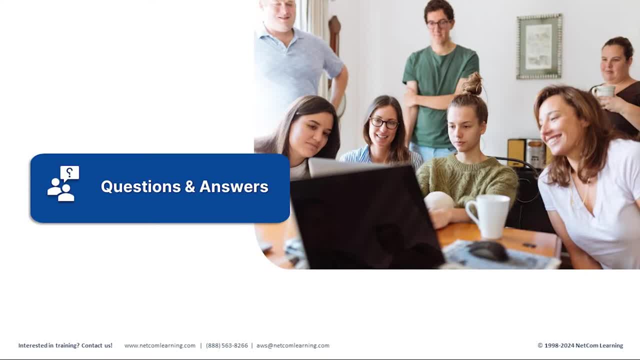 To deploy that into the account. that's not that you don't own or you don't control, right. so that's the one thing. but if it's in the organization, it's most likely that it's in your. your company and then your CloudFormation need to have access to those accounts. it's called cross account access. make sure you have that permission set. once you do, it's like it's like magic. it's pretty beautiful. you create a stack set in one location, you say deploy and boom, you'll start deploying on all those different accounts. okay, so I hope that's helpful for you. 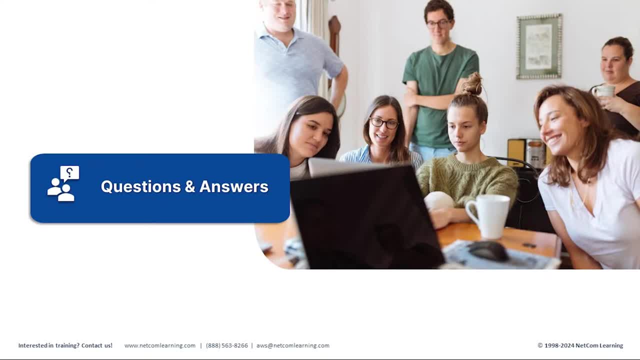 And let's take another question from Dan, who would like to know: can you provide more examples on integrating Jenkins with AWS DevOps? yeah, thank you so much. so I've used Jenkins before as well and Jenkins is very, very extensible. let's say okay. and for those of you that's used Jenkins before, you probably realize it has like tons and tons of plugins and the those plugins. 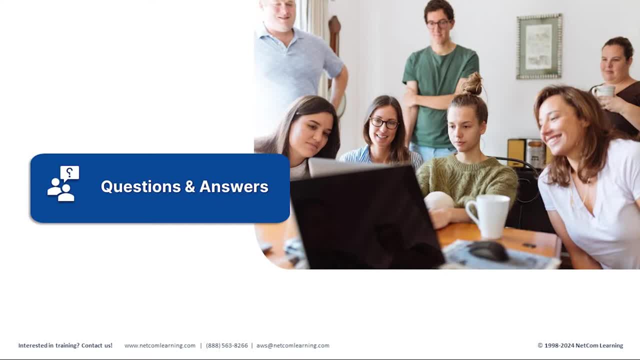 There are many, many AWS plugins. so the answer is yes, right, Jenkins, you can definitely integrate them in various places. so you could- I guess, not, not I guess, but you can- if you wanted to replace the whole code pipeline right with Jenkins. if you wanted to, and you could work with code build, code deploy using Jenkins, you could use code commit with Jenkins. so, yes, the Jenkins is highly integratable with AWS services, but not only that. 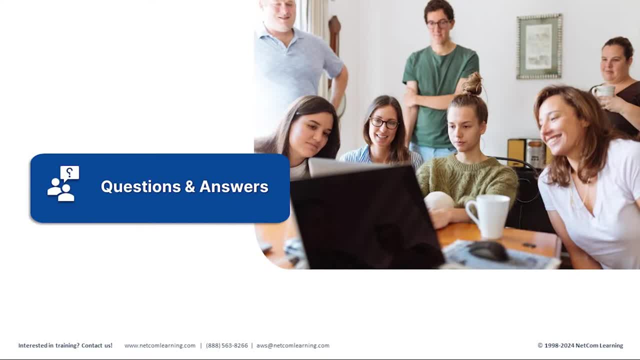 Not only that. if you wanted to, let's say, run Jenkins, right, you need a Jenkins server, don't you? okay, and normally what one would do is you take a EC2 instance and you install the open source version of Jenkins in there and you set up Jenkins, but with AWS. actually, AWS provides a way for you to make that more highly available. that is, there is a plugin on the EC2 that's just for Jenkins. 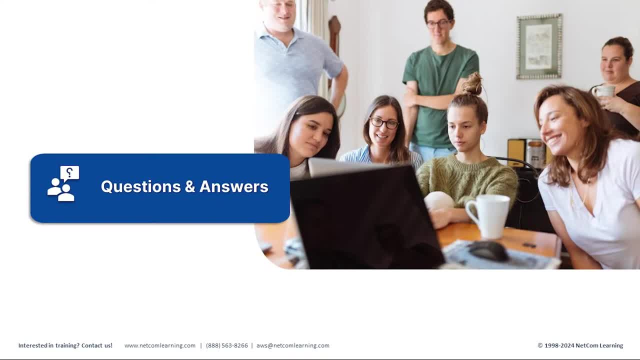 So that you can have a master Jenkins server and then you have the the worker Jenkins server, just in case you need to do like parallel work or more work than you need. so so you know, if you want to implement Jenkins inside AWS- I'm not even talking about integration with any other, like code build and stuff, just Jenkins- right, you can have it built as a very highly available version of Jenkins, which I think is like fantastic. 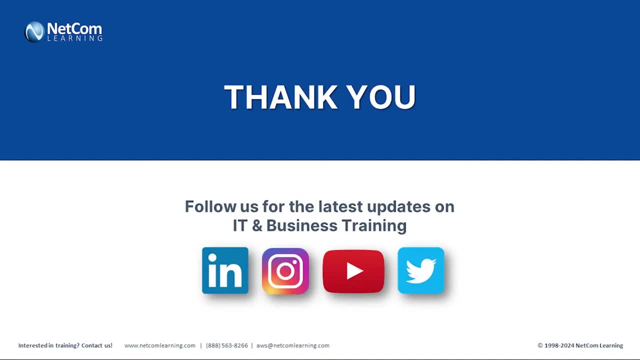 Once again, I want to thank you for your time. I want to remind you that as you leave the session today, you will be presented with a short survey. we would like to request for you to help us by taking a quick moment to participate in that survey. your feedback really helps us understand your learning experience, as we are constantly looking at how we can improve our future sessions. the survey answers are measured on a scale of one to five, five representing outstanding and one representing core. 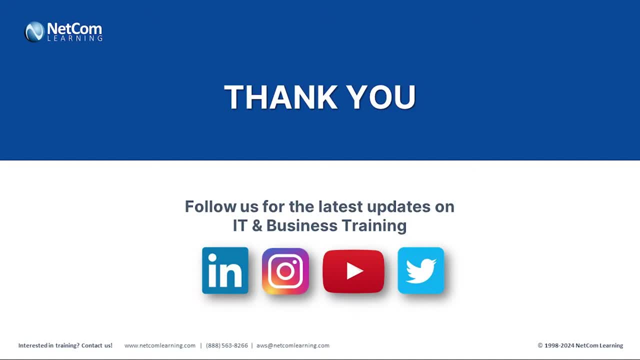 We want to thank all of you for joining us today and if you do come up with any additional questions, feel free to send them to webinar at net com learning dot com at any time. We hope that you found today's webinar informative and we look forward to seeing you back here with us soon. feel free to tell your friends and colleagues about our webinars and other courses. have a great day everyone. 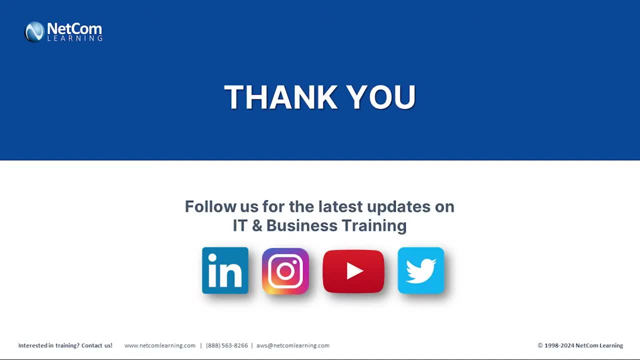 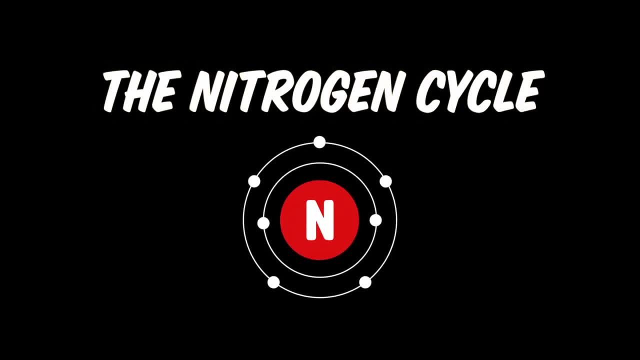 All right, now we've made it to nitrogen. Now this is the element that most people become first associated with in gardening when they start thinking about amendments or what minerals or elements or nutrients go in the soil. This is the first in the NPK. It is the